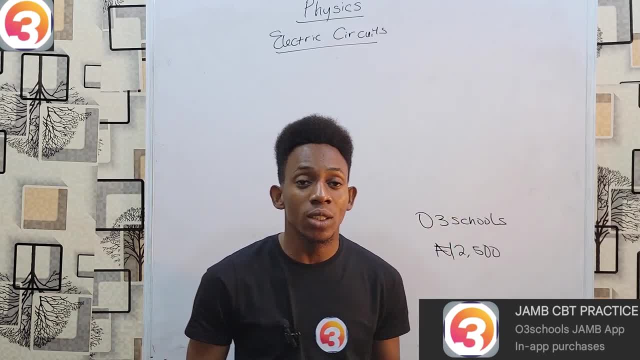 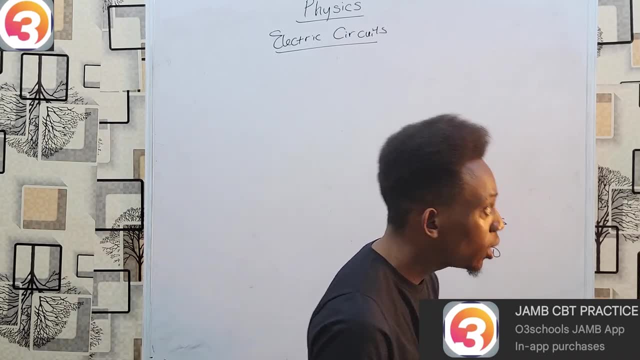 And one key thing we shall learn is that, when using these circuits, we don't just draw wires in the typical way you see them. If you look at the wires in your house, they are usually scattered. We do not draw our wires for our circuits in that manner Instead. 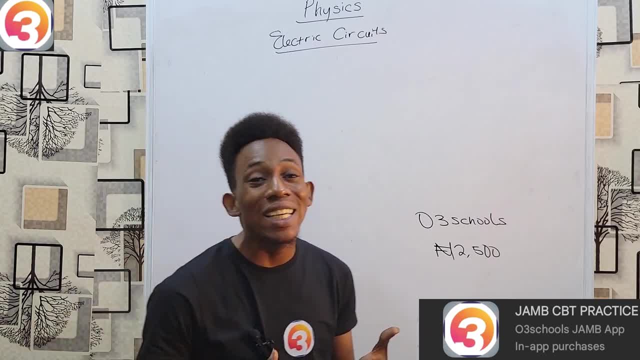 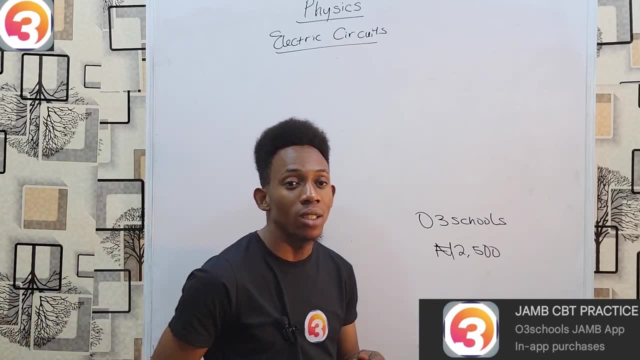 in circuits. they are simplified to give us ease of drawing and understanding And instead of drawing the complete feature of the circuit, we can draw the circuit in the way that we see it. So let's look at the circuit of a particular electronic device. We can use different symbols to represent. 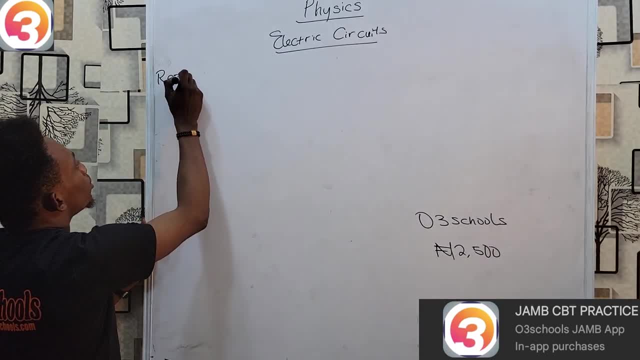 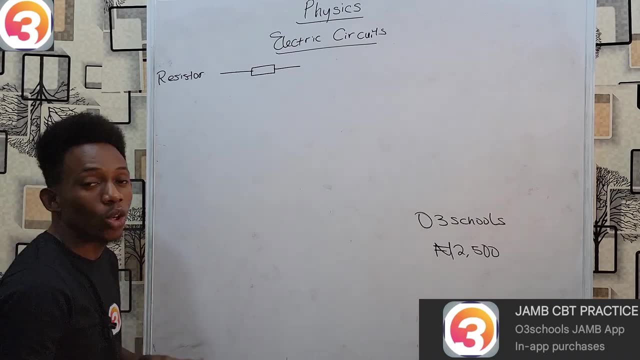 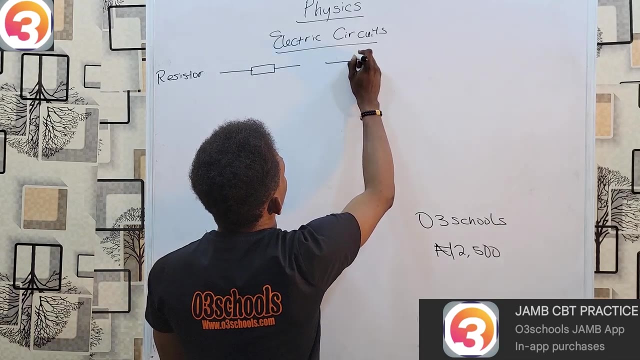 them. For example, a resistor is simply represented with this. That's all we used to represent a resistor. If you go through all the years of your past questions, you might see resistors also represented with this. So that's that for the circuit. 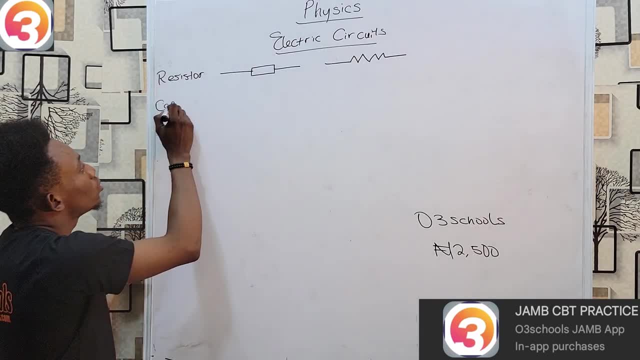 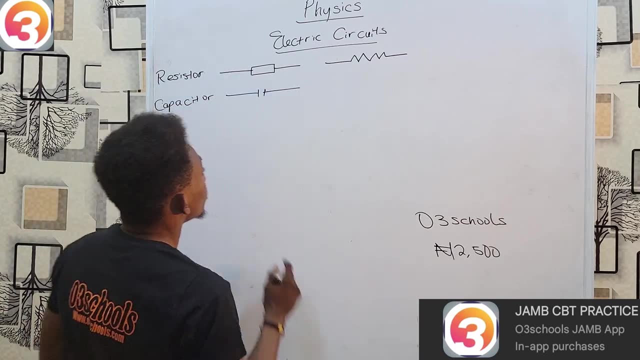 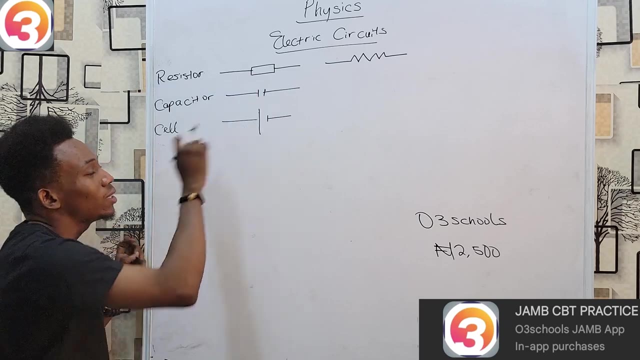 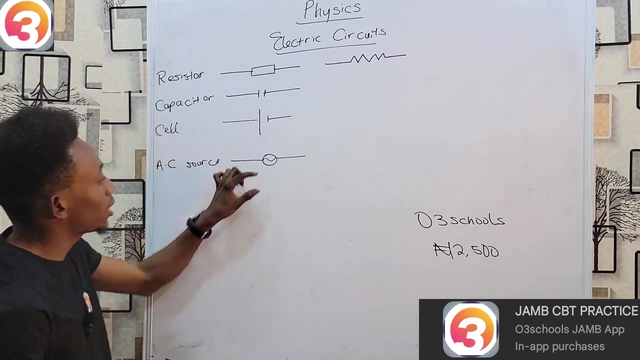 for the register of all, for your capacitor. a capacitor is presented simply with this. your cell or your battery is presented with something similar to the capacitor, but one is longer than the other. um, even your ac source, which is what we call our nepalite nigeria, is simply in this form. this is that. this is ac. this is getting from your cellular battery is 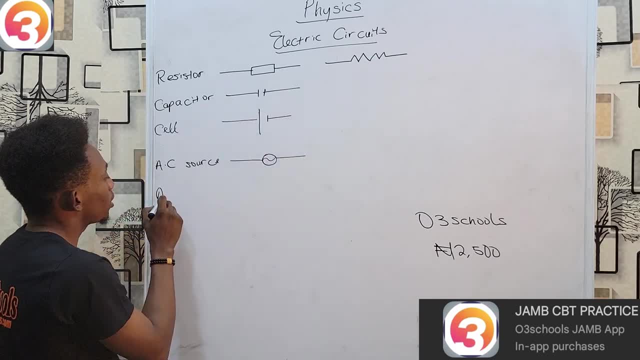 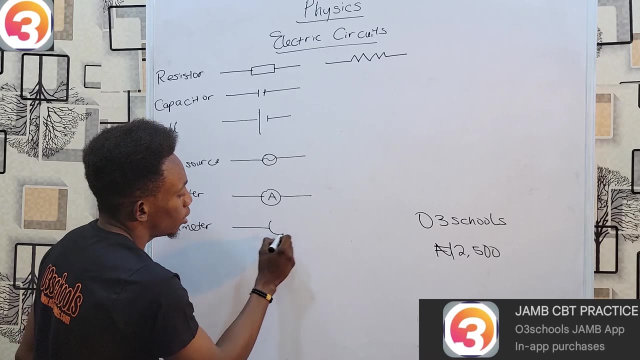 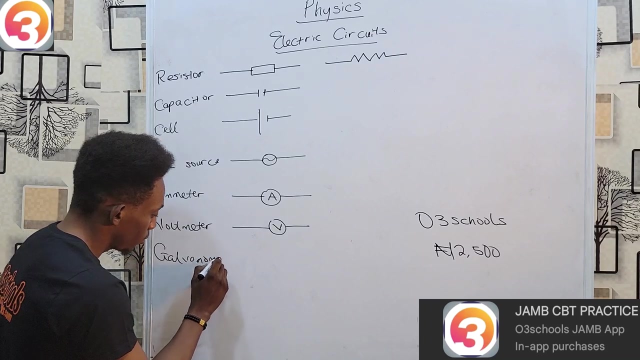 dc, then um, there are other things you could represent. an ammeter. an ammeter is simply like this: um, there's also your voltmeter, pretty much the same as your ammeter, but now we have v and even a golf andometer, also quite similar, but we have a g. then there's a transformer. 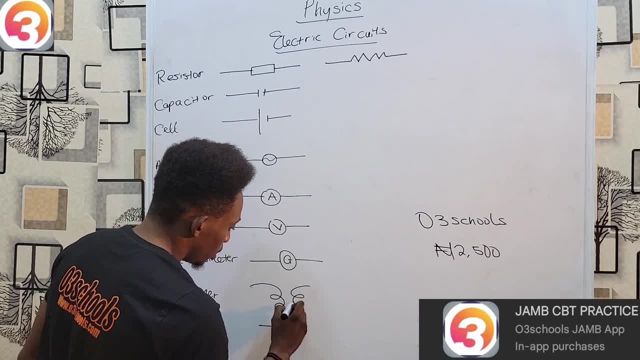 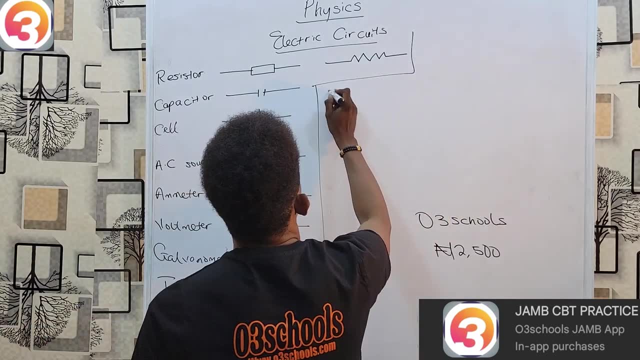 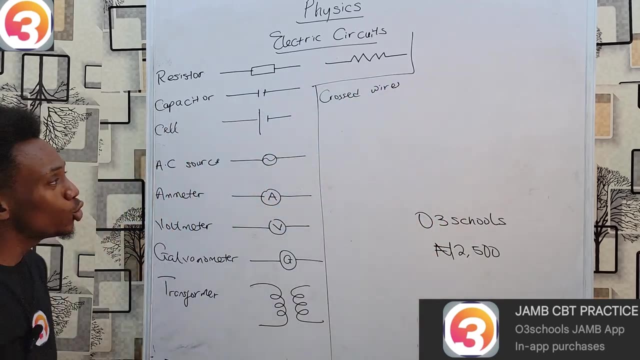 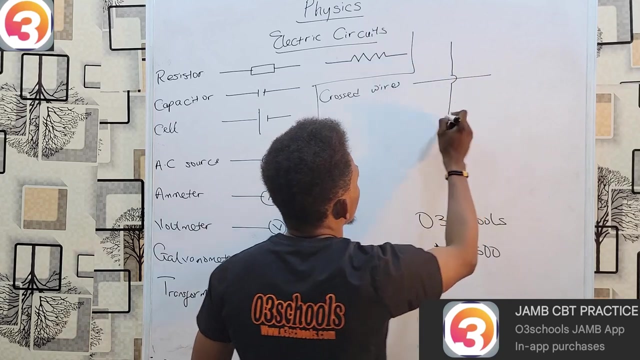 and um, this is your transformer, then um, we could also have what we refer to as crossed wires. what if a wire to pass another wire? we don't just draw them caught in each other, no, instead we draw something like this: now, once you see this in a circuit, this implies that this wire passes where this wire is. 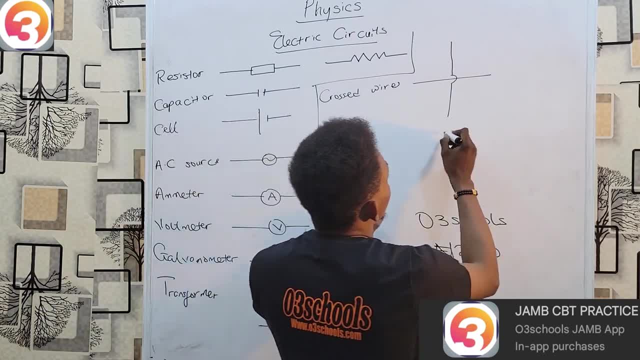 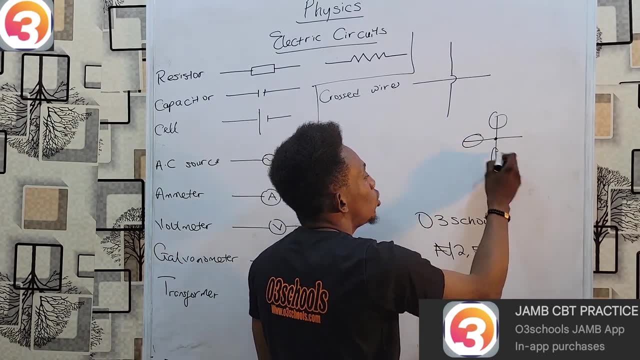 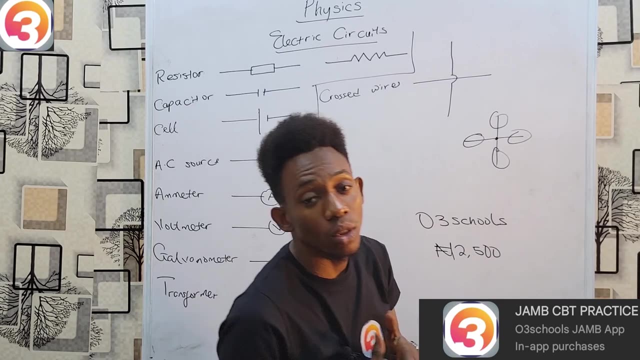 but they are not connected together. if it was drawn like this, then this would be a junction at which this wire, this wire, this wire and this wire are all connected and meeting. however, this tells us that his wires do not have any joints or any connections between them, and 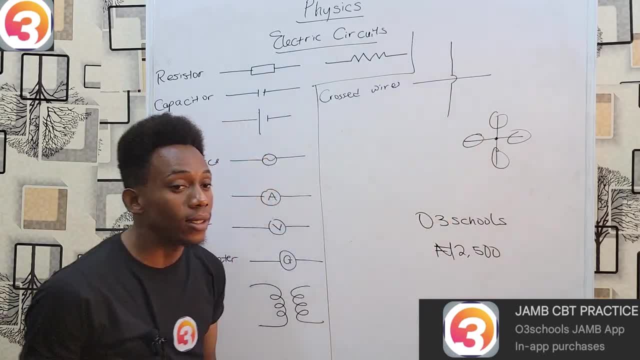 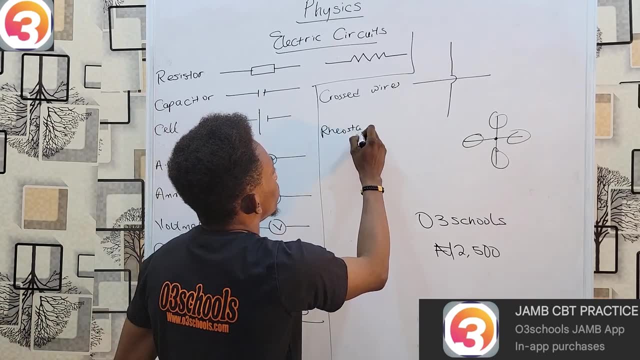 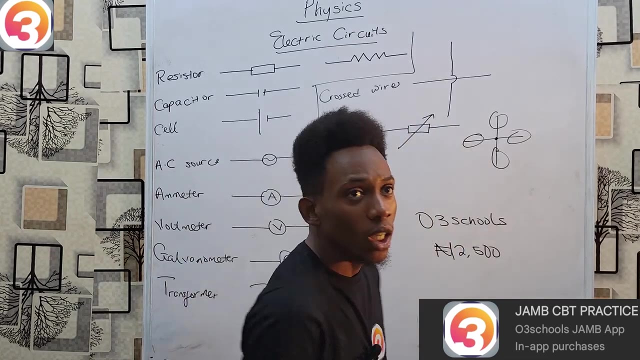 even they do, it doesn't exist at this point in the circuit. so there are so many things. there's even a real stat or a variable resistor. we simply register whose value can be alternated. a good um, a good way to picture. that is in the controls for your. 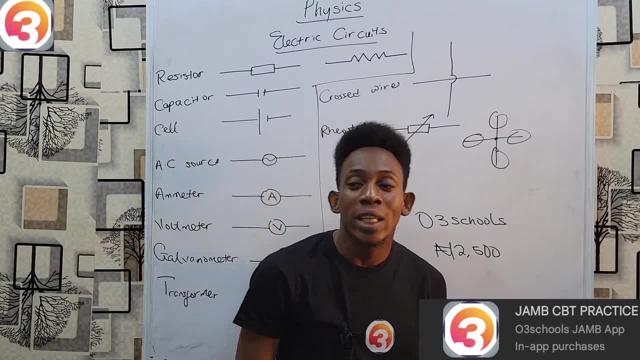 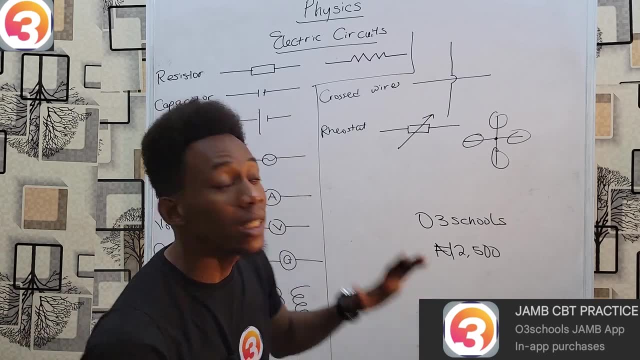 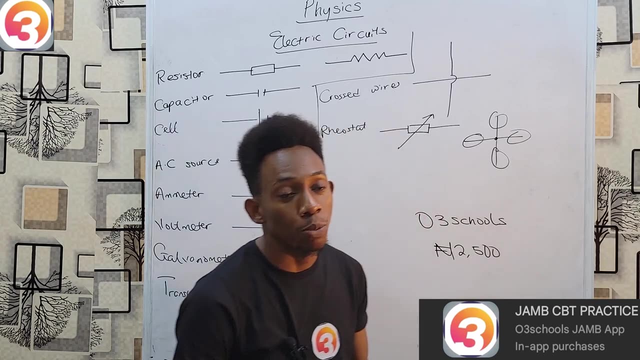 ceiling fan or standing fan. you are able to increase or decrease the speed of these fans by moving your switch. all you're simply doing is that you are varying the resistance and, as a result, you are varying the amount of current getting into the fan and, as such, the speed. 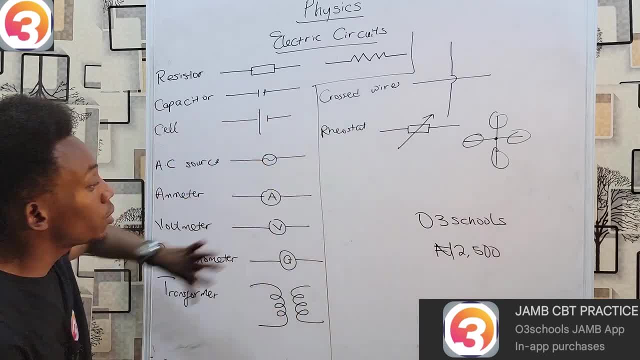 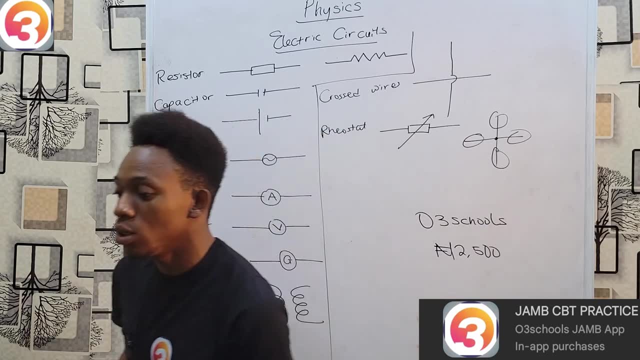 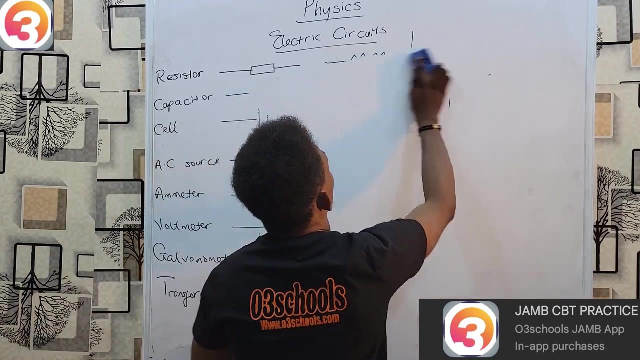 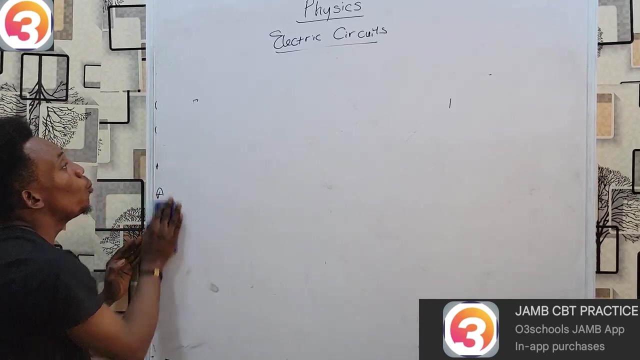 can vary as well. so these are several elements which i see inside electric circuits, but for now we shall pay special attention to the resistor. and the reason for this attention to the resistor comes from one of the fundamental basic laws in physics, which is ohm's law. 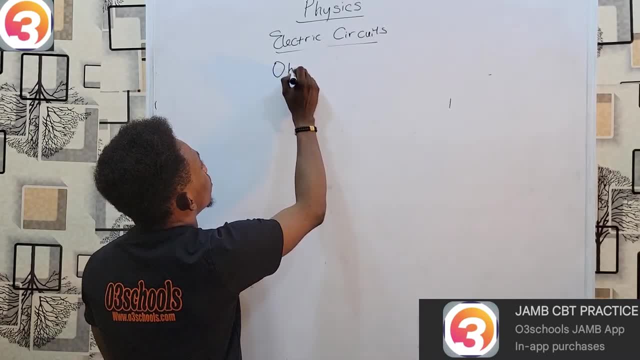 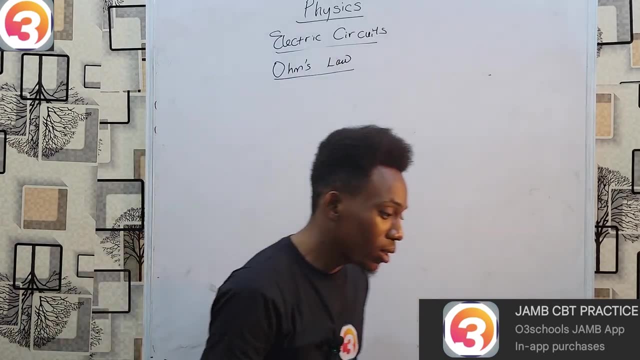 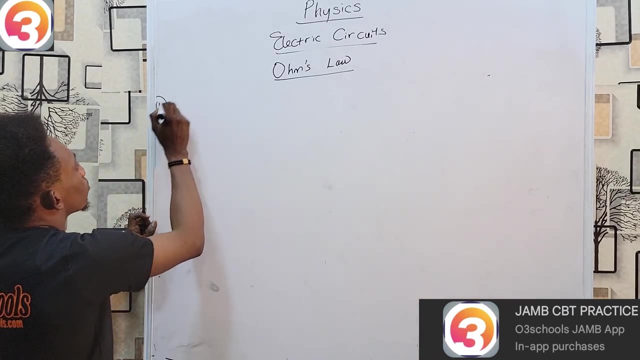 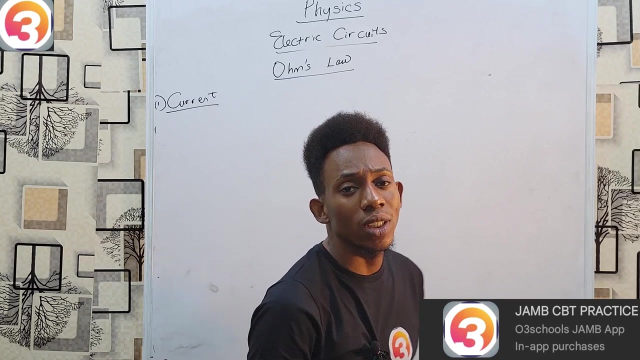 so we shall be studying ohm's law. however, to fully understand what this law is telling us, there are a few elements we need to understand first, so we should start by looking at currents. what is electric current? now, contrary to what a lot of us think, current is not something you can. 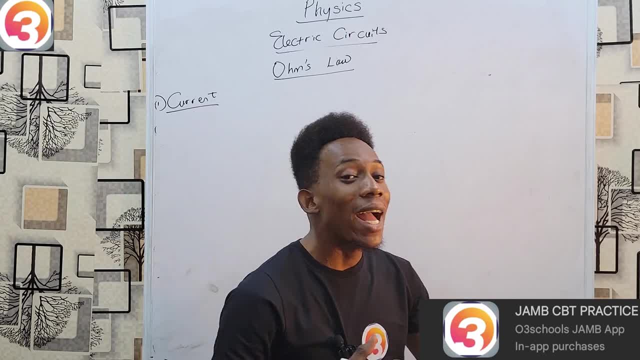 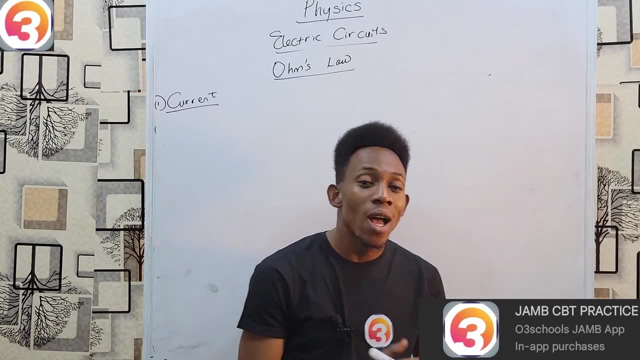 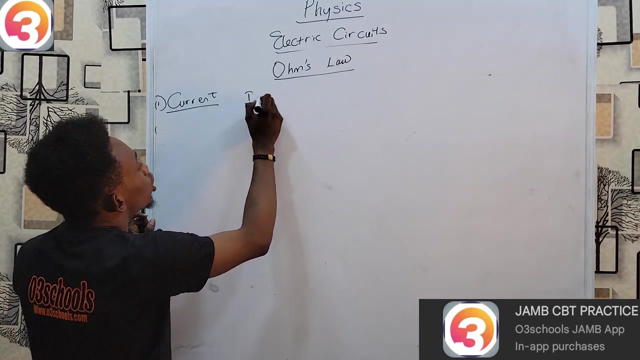 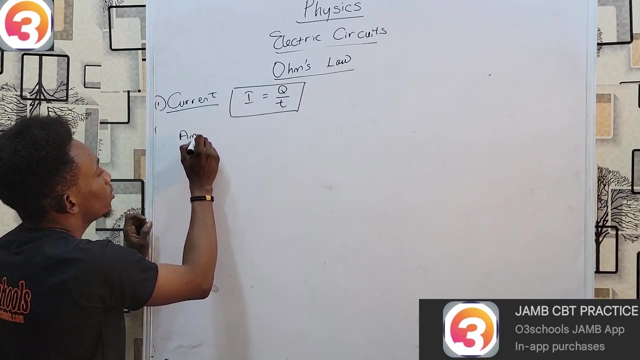 see or touch what passes through your wires are charges, not current. current is simply a measure of how fast these charges are moving. current is the number of charges passing through a wire per second. so while current is not something tangible, charges are. so current is it charges a second? current can be measured with an ammeter. 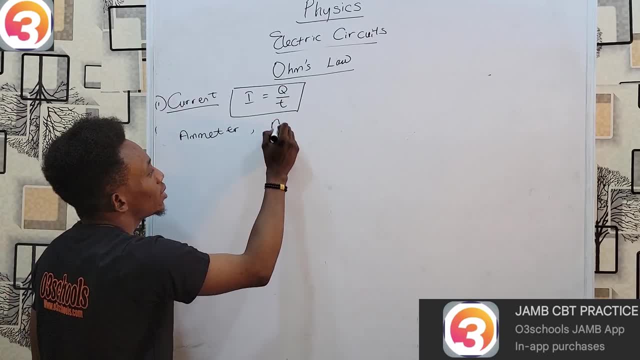 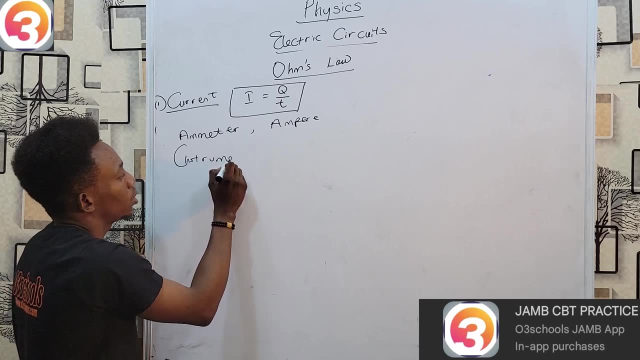 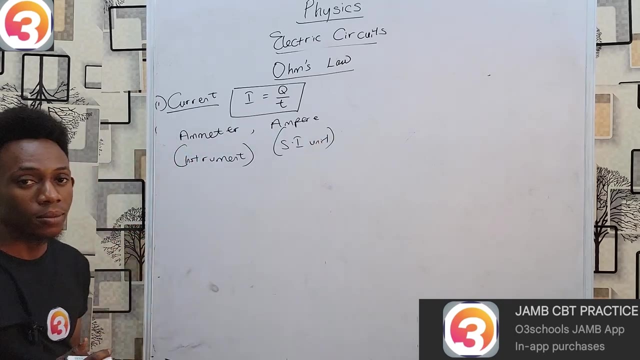 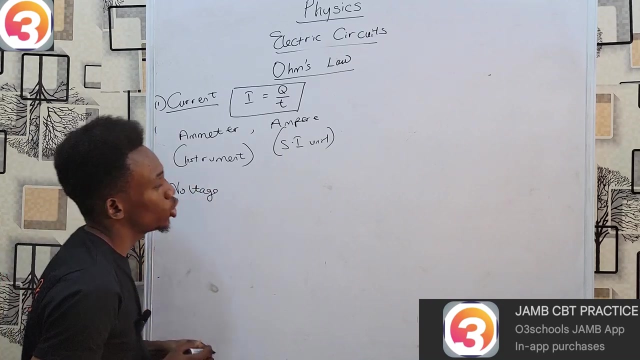 which is measured with an ammeter, and the unit of electric current is ampere. ammeter is the instrument to measure the ampere, but we'll focus on the circuit of electric current by seeing policuees and much more, while ampere is the si unit or current. now, the next thing we shall look at is voltage. 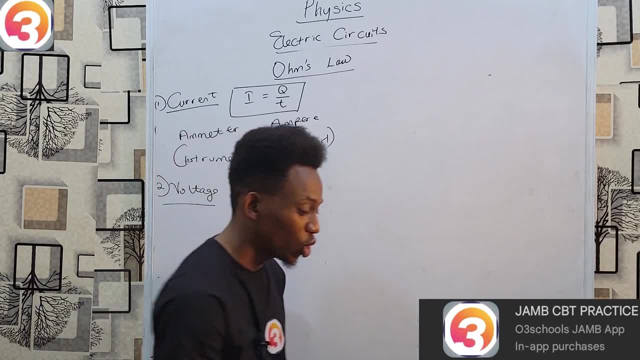 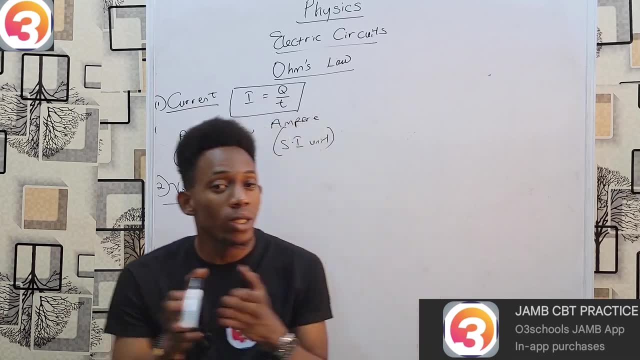 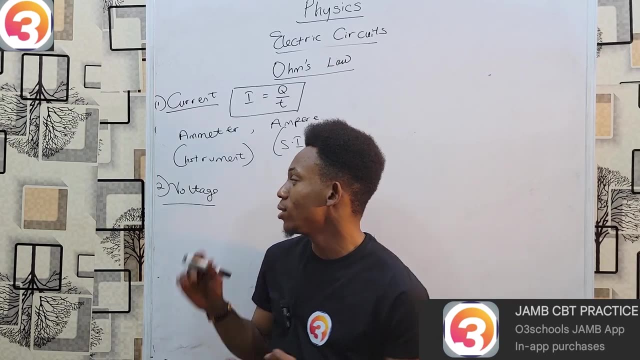 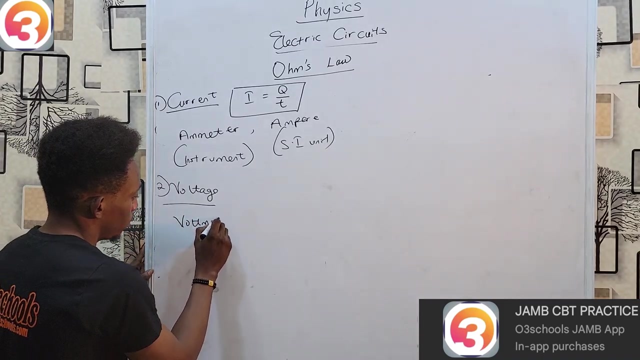 voltage is the driving force, or electric current, for current to flow. something has to make this current move from one point to another. now, that necessary agent for the movement of this current is what we then refer to as voltage. voltage is measured with a voltmeter, and its unit is volts. so, just like before, voltmeter is the instrument. 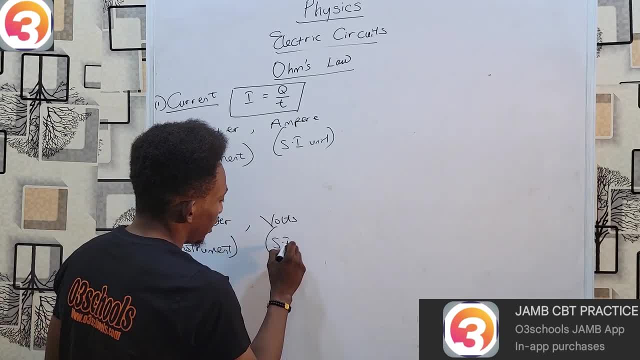 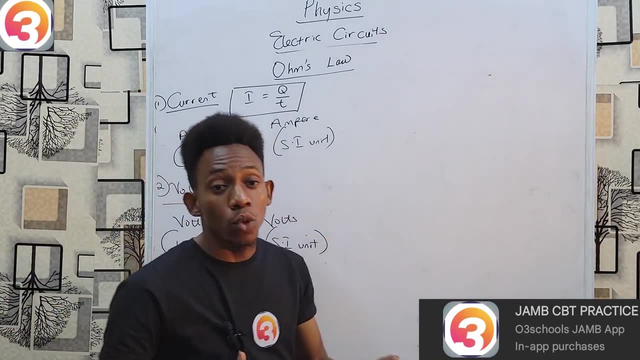 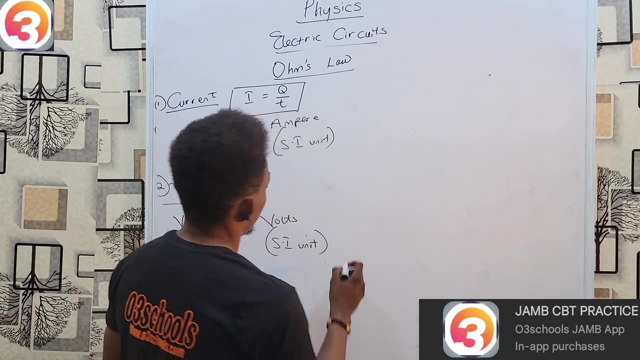 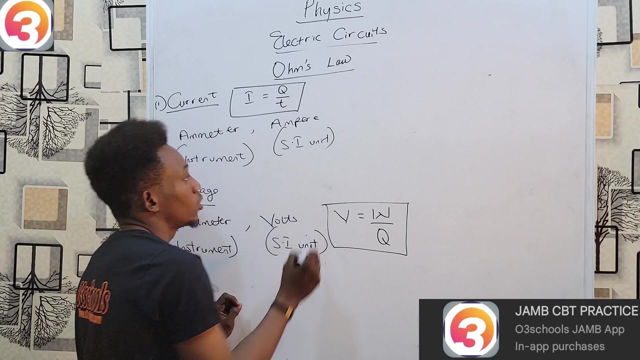 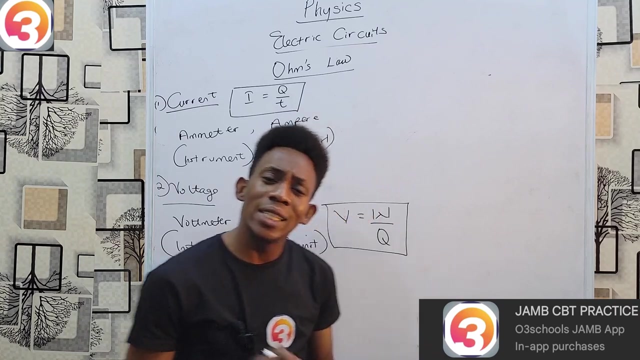 while volts is the si i units. however, to get the full amount of voltage, remember that voltage, therefore, is to be the work done in moving a unit charge. therefore voltage goes to work done over charge. so current is charged over time, voltage is worked on over charge. now, in the analysis of voltage, however, there are two ways voltage is studied. 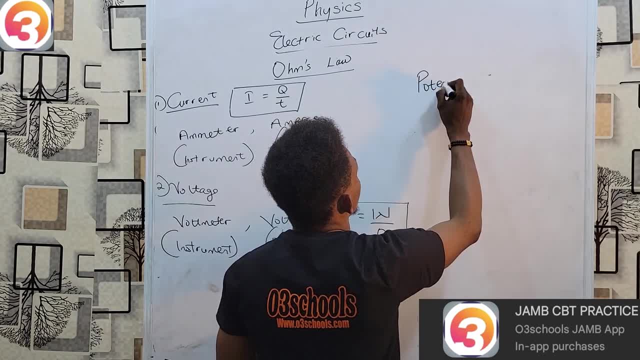 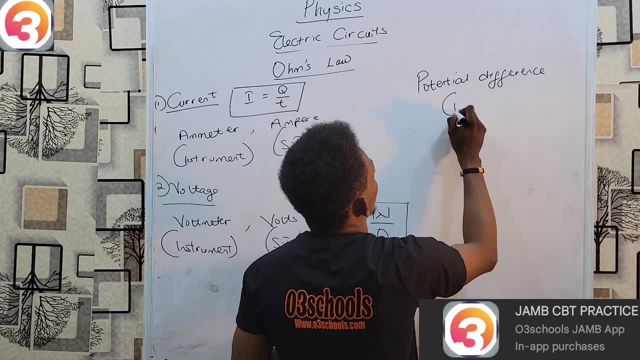 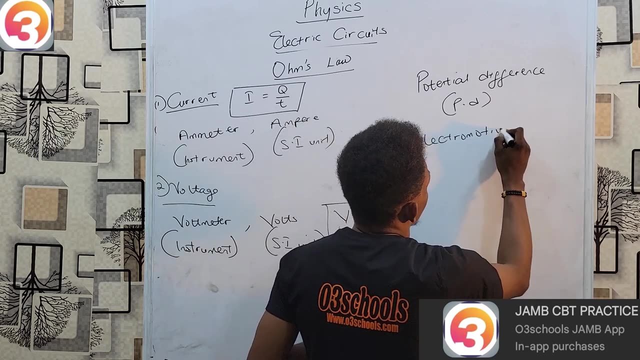 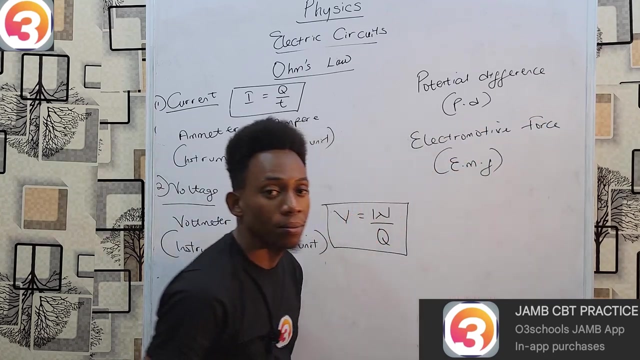 one is to work on over charge and the other is to work on over charge, and one of them is potential difference. there is potential difference, and this is often called pd, and then there is electro multi force, electro multi force, and he's commonly called e m f. now, the potential difference is the work done. 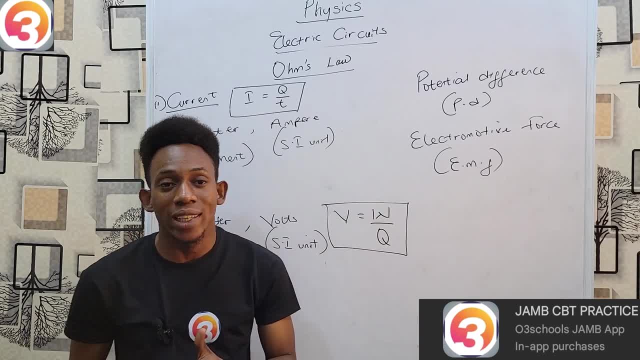 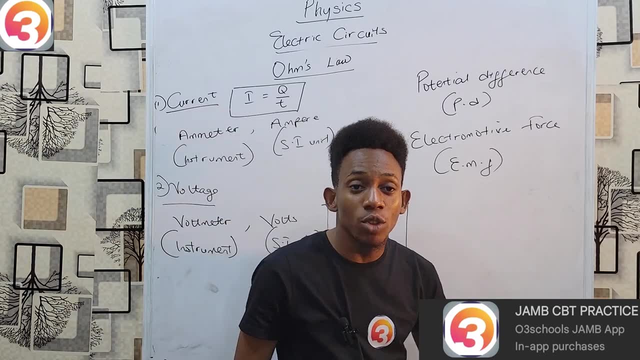 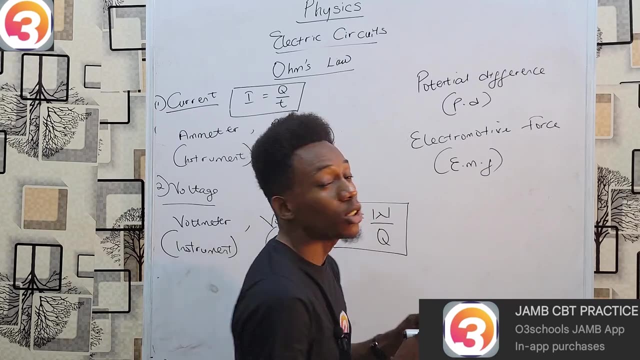 in moving a unit charge from a point within the circuit to another point, while the electromotive force, on the other hand, is well done in moving that unit positive charge in from infinity to a point in the circuit. that means it's what the force takes the charge pretty much around the circuit. 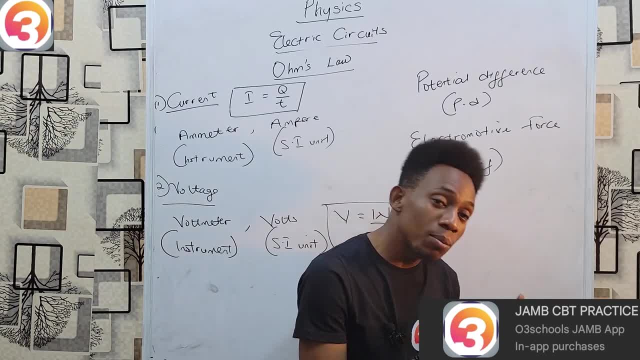 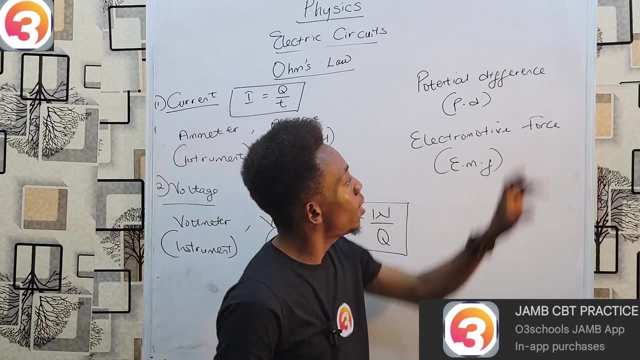 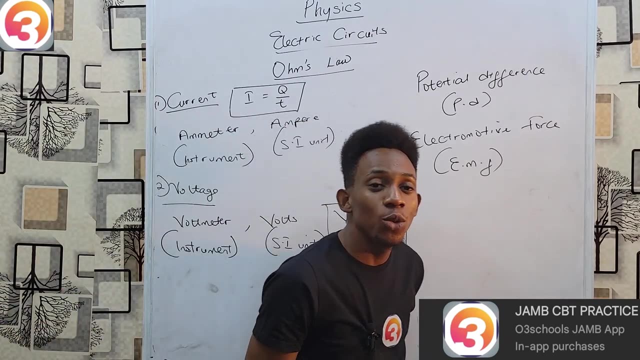 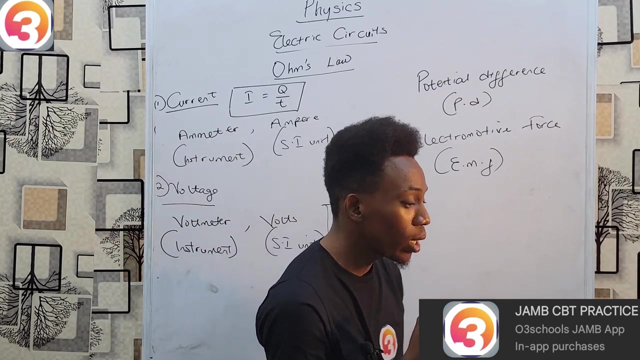 the initial difference simply tells us the difference between a certain point and another point in that circuit, difference between their potentials. so, however, both of them can be generally referred to as voltage, so commonly they are used interchangeably. but in analysis of cells or batteries, electromotive force is usually the 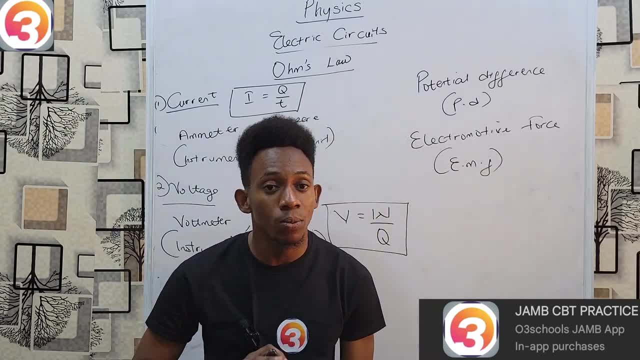 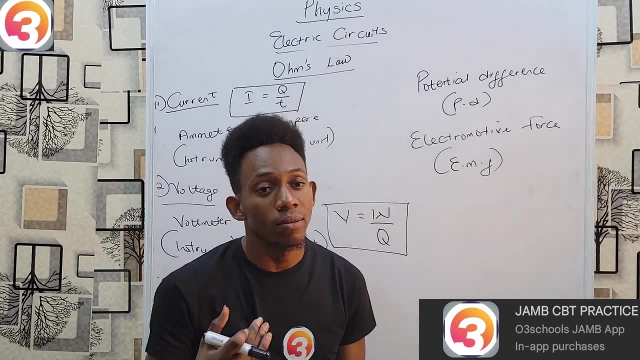 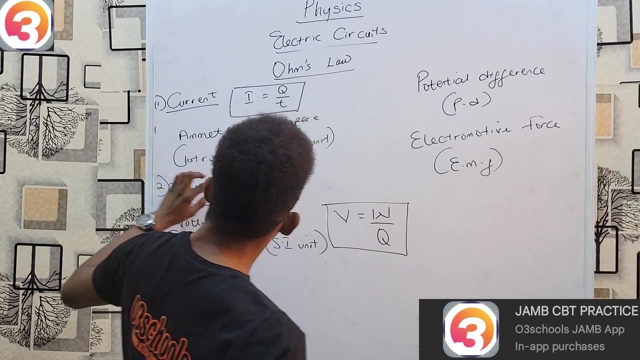 rating for the battery when it is not in use as a whole. but when it is in use we commonly get voltage of potential difference out of it. but that's topic from that time right now. we're focusing now on just this basic knowledge that we can analyze voltage. 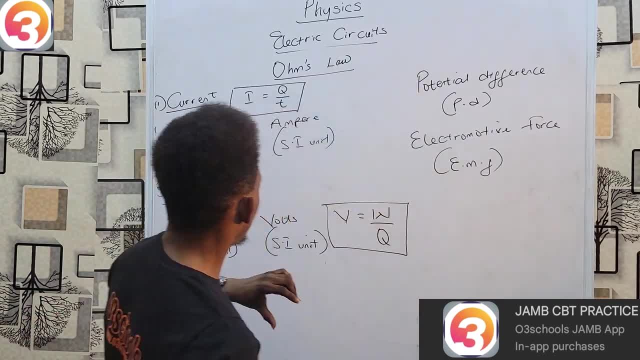 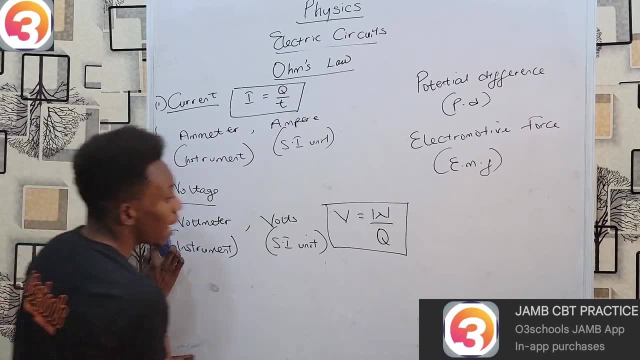 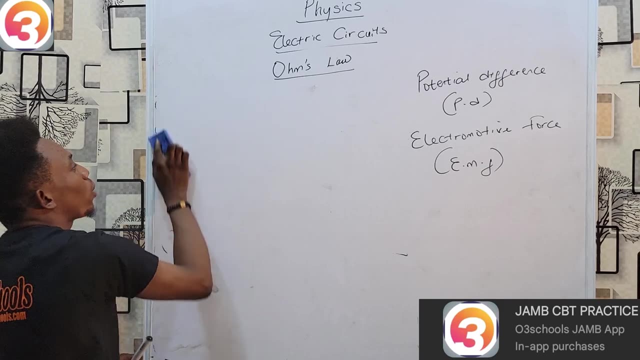 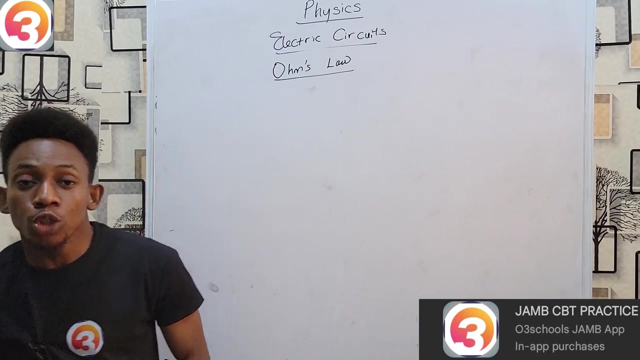 in terms of both potential difference and electromotive force. so this is my first base, and once we note this, we can then actually move forward and study ohms law. now. ohms law is quite simple and it can be stated very simply. ohms law states that the current flowing 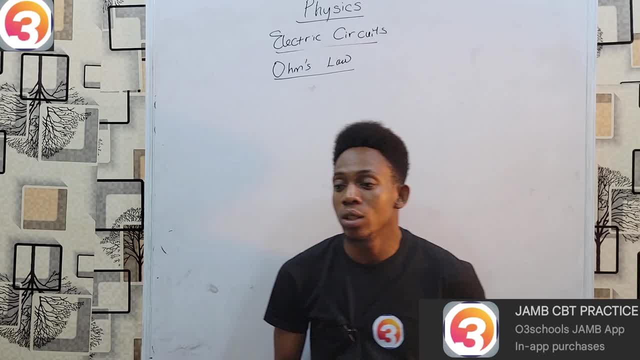 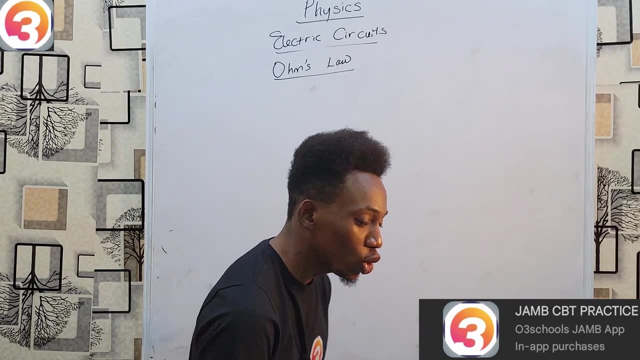 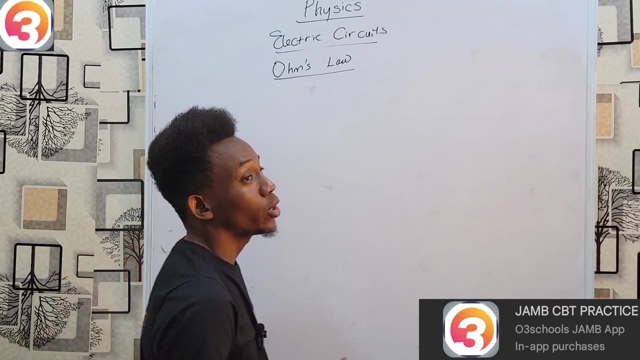 through a metalic conductor is directly proportional to the potential difference across its end. provided temperature and other physical factors remain constant. the current flowing through said conductor or any metallic conductor is proportional to the potential difference across the ends of that conductor, provided that temperature and other physical factors remain constant. 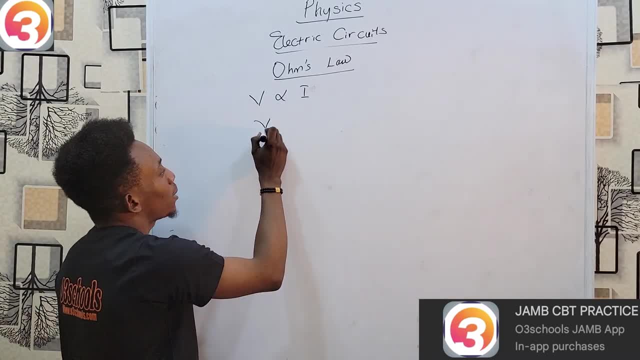 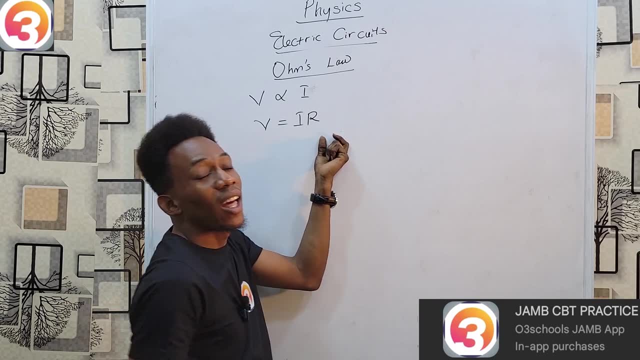 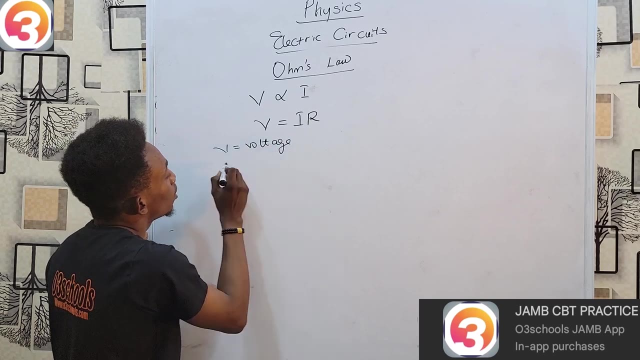 in this case, in fact, we are doing the same stupid thing. so we are going to look at the rule of law. we are going to use a constant for this datum. we are going to use a constant for this datum which is v proportional to i. and then, from a knowledge of mathematics, 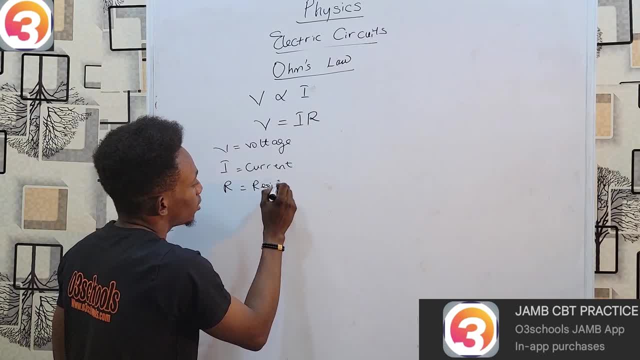 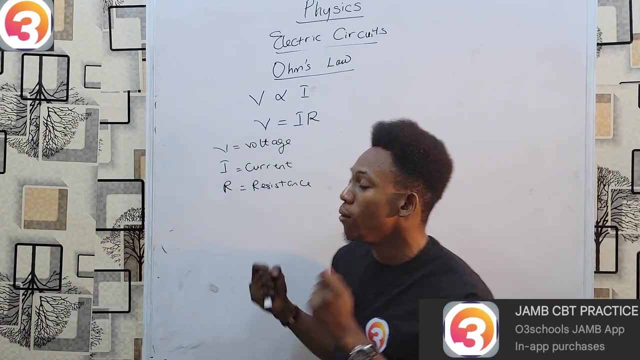 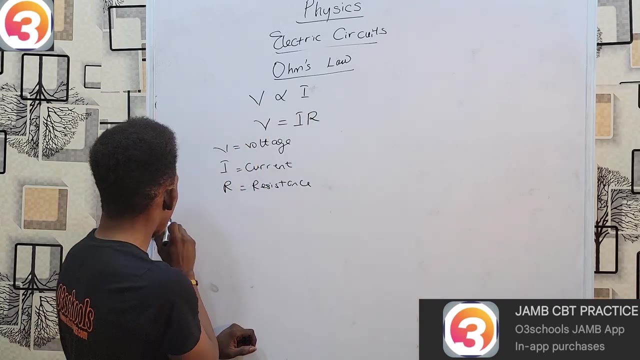 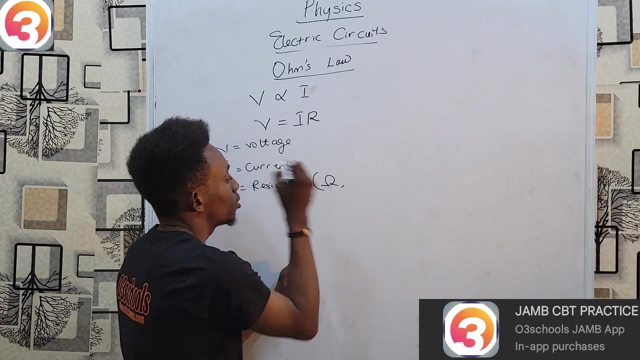 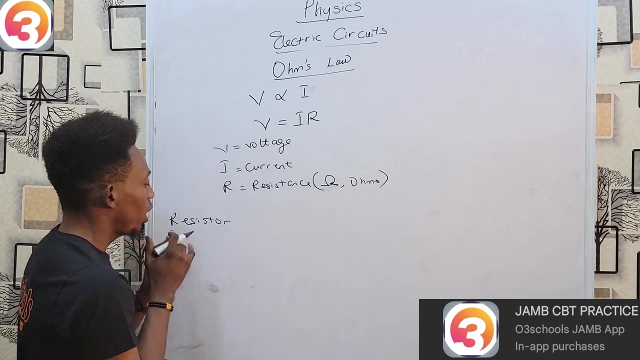 you must introduce a constant, but this constant, in this case, is referred to as r, and r is the. resistance is the opposition to the flow of electric current, and the device whose job it is simply to provide resistance is referred to as a resistor. the unit of resistance is ohms- ohms in words, for its symbol is your Omega. so a resistor is a. 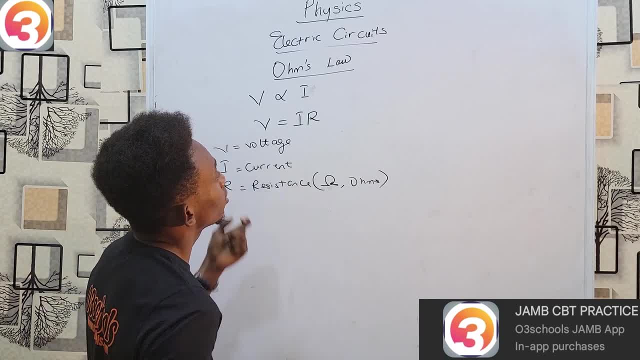 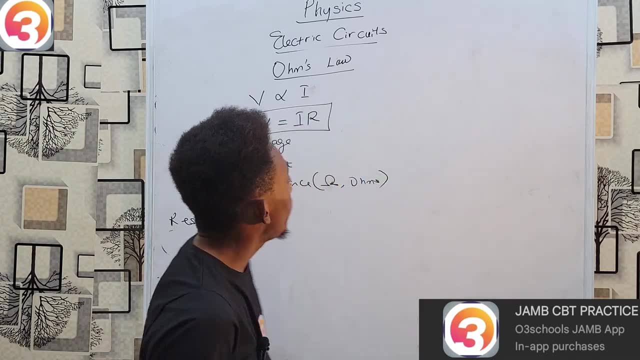 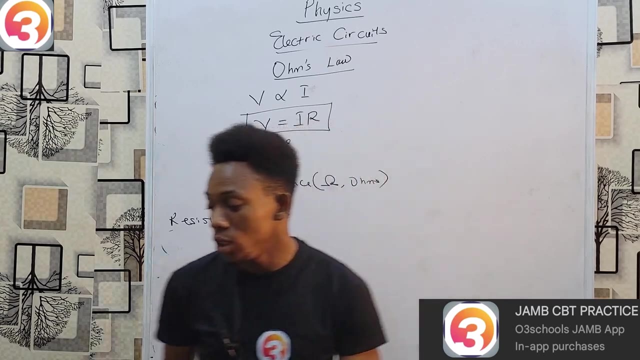 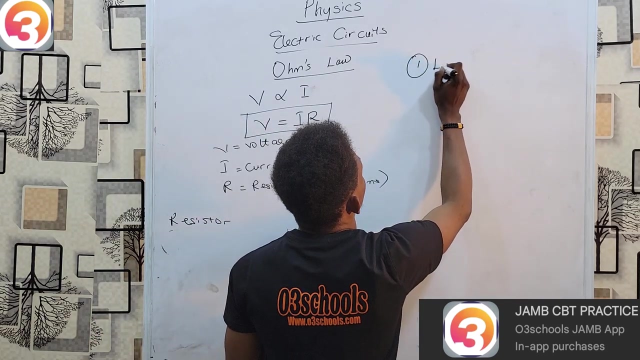 device whose job it is to provide resistance, and this is our formula for ohms- ohms. now, if we want to get resistance from a resistor, what are then the factors that can affect the resistance of this resistor? now, there are about four factors that affect it, the first of which is the length of the resistor and all we must. 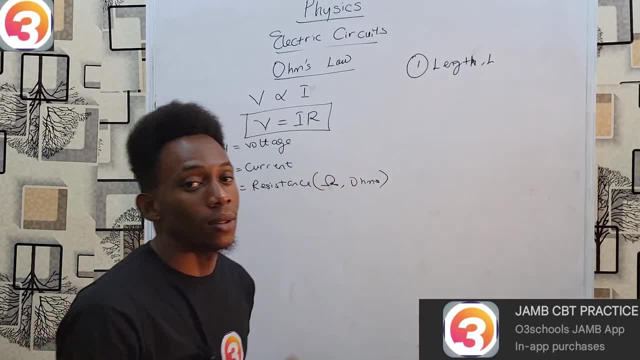 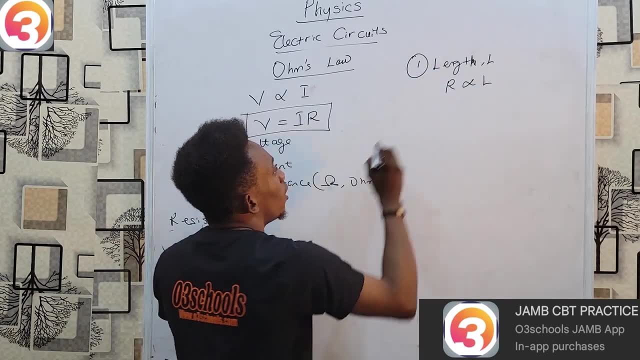 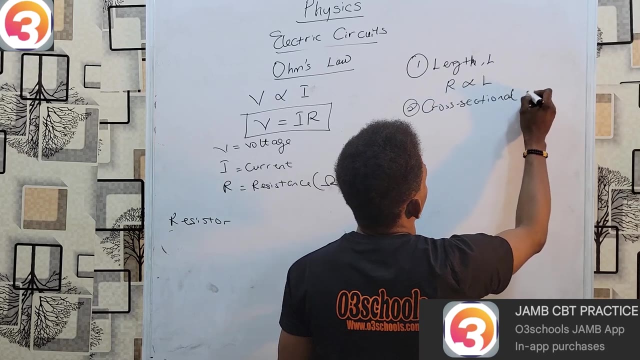 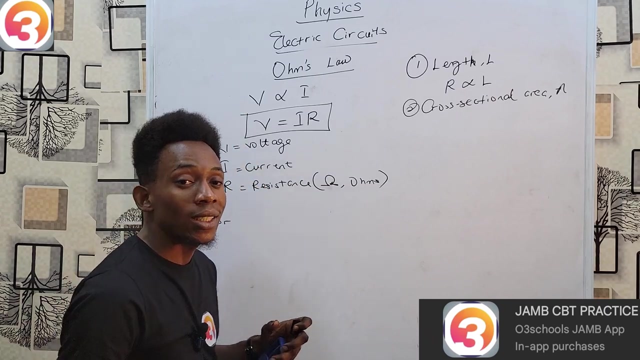 know about this is that the greater the length, the greater the resistance. the shorter the length, the shorter the resistance. that is the direct variation. then, two, we also have the cross-sectional area of that resistor and for this it's an inverse relationship, indicating that the bigger the area, the smaller the resistance. and 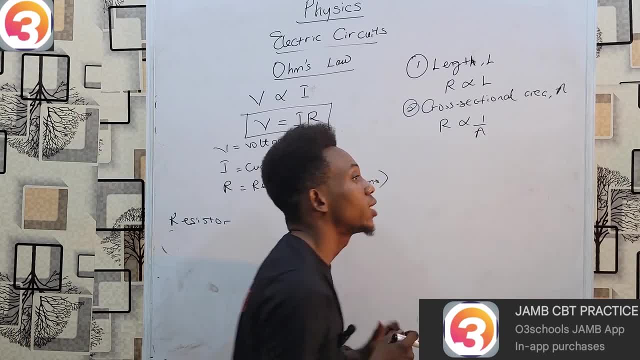 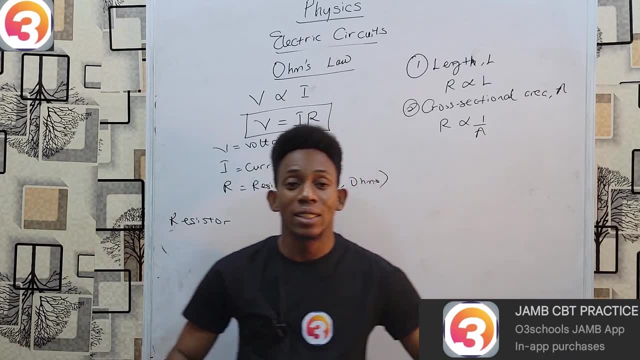 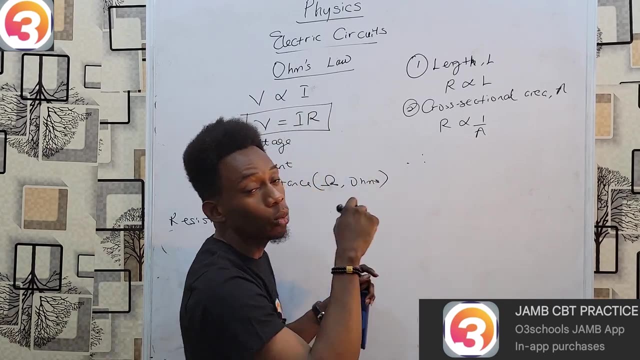 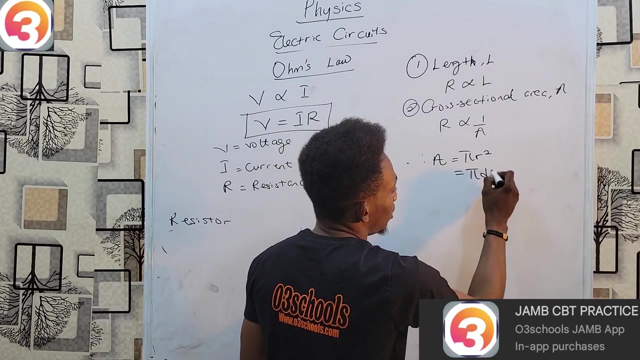 the smaller the area, the bigger the resistance. now, typically most wires come in cylindrical forms. there are tiny cylinders, which means that the cross-section is usually a circular cross-section and therefore in those situations the area is given as pi R squared or pi D squared over 4. that's for. 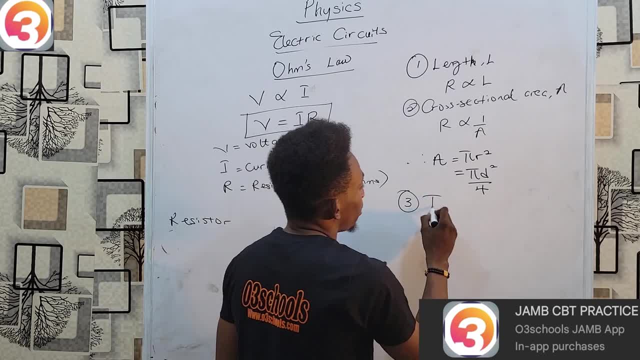 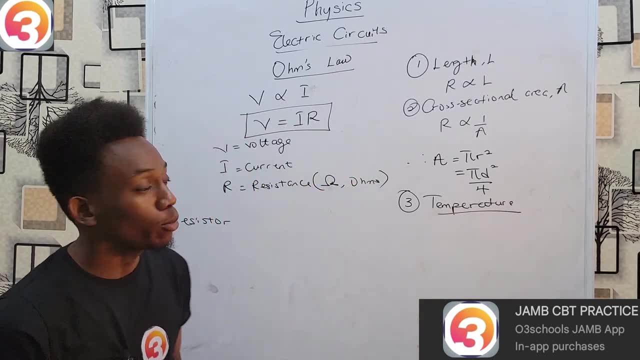 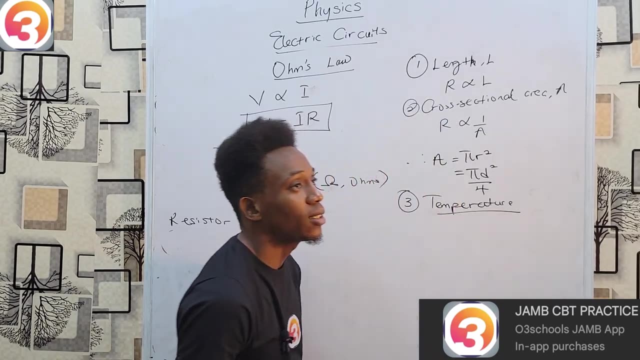 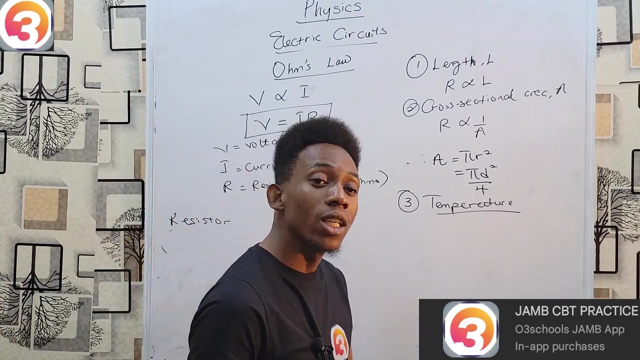 the area, then the third thing that can affect is temperature. now, the behavior with temperature differs for different types of materials, or metals or your semi metals, but generally resistance decreases with temperature. that means resistance decreases with increased temperature and increases with decrease in temperature. well, last but not least, 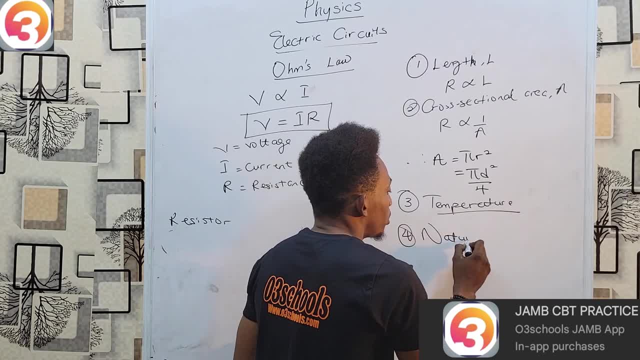 4. the nature of the material. 4. the nature of the material. what does this imply? what will the material's body health affect? do not react to certain acids or substances, blood or water content levels of毌�uc. 배우의 사 расск기. 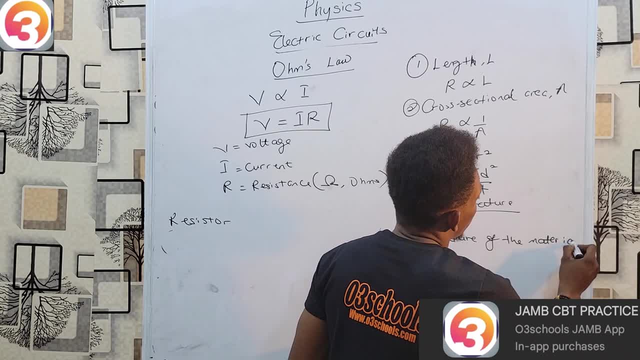 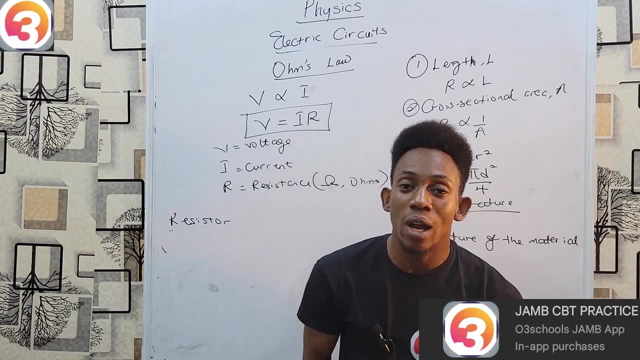 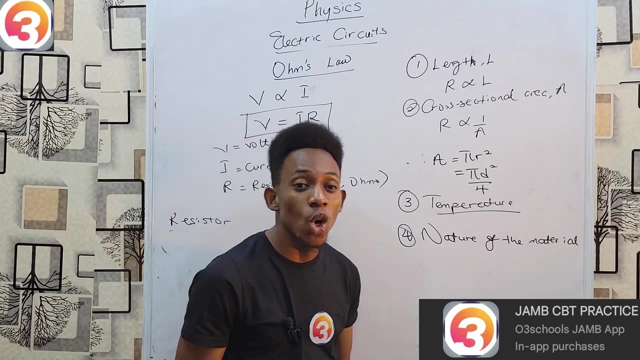 Tell us. what does this conveyという어 means is that it has to take several samples of different materials of the same length, same constitutional area, all at the same temperature. these two shall not have the same resistance. there's an intrinsic property to every single material that determines its level of resistance. 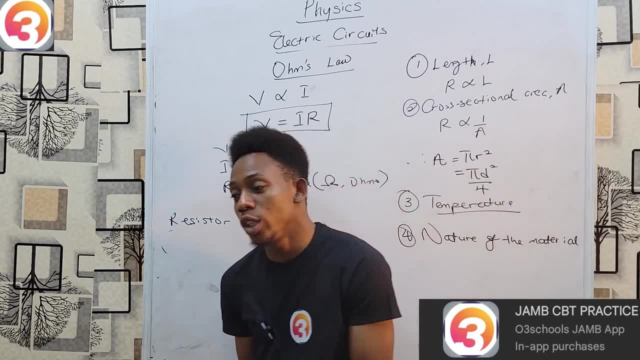 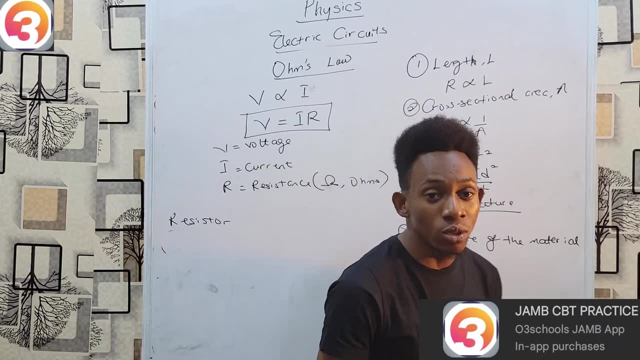 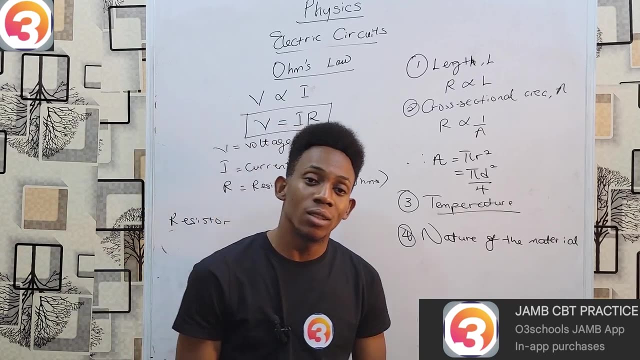 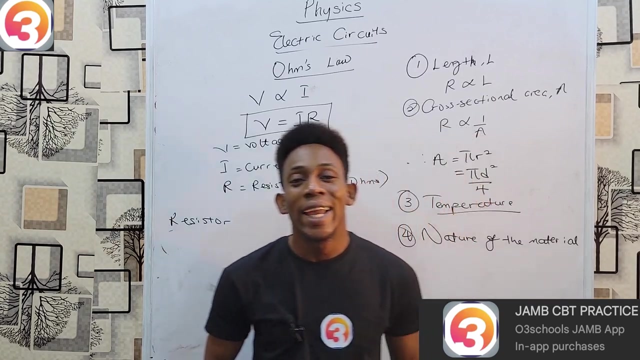 generally, we refer to them in terms of conductors and insulators. conductors are those materials that let electricity pass through easily, while insulators are those which not let electricity pass through easily. please keep in mind: insulators eventually do let the electricity pass through, but it is not easy. the voltage required for electricity to pass through most insulators is very, very high. 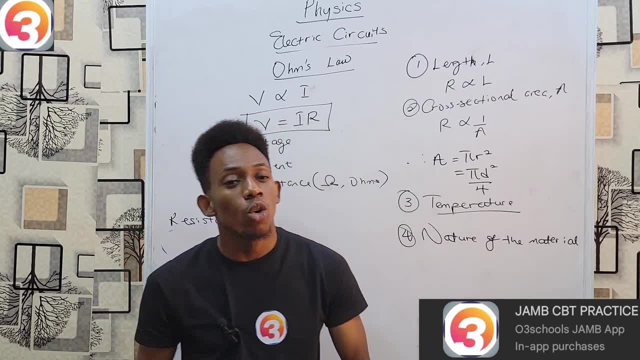 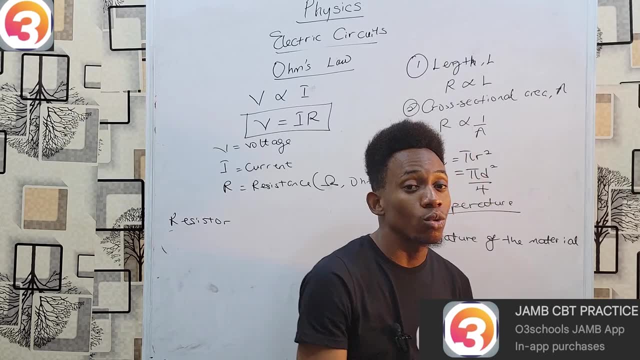 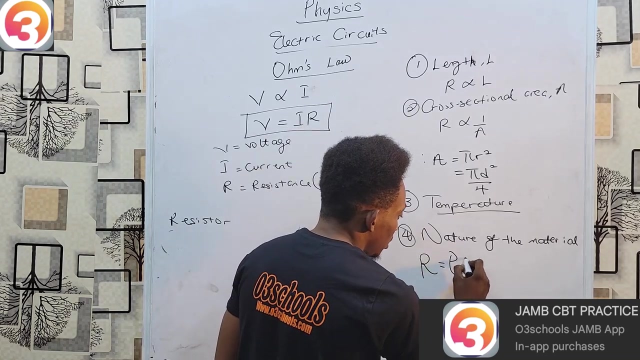 but they are not to be confused and called non-conductors. the term non-conductor seem to imply that hsd can never work, pass through, which is simply not true. it is simply very difficult. so combining all these into one formula, we can then see that resistance of any material equals the resistivity that means the. 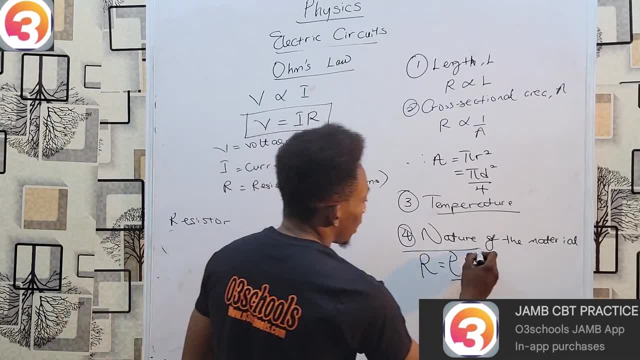 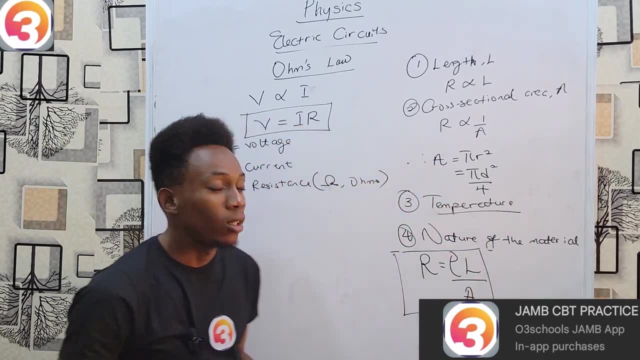 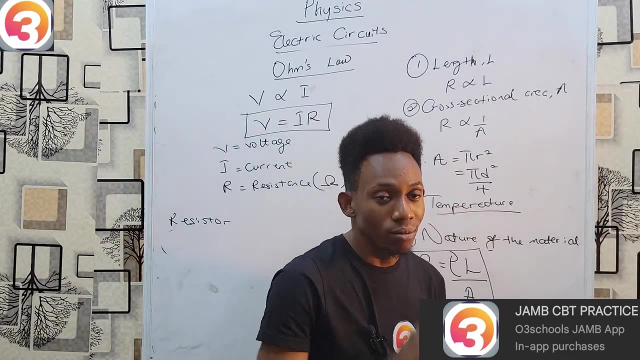 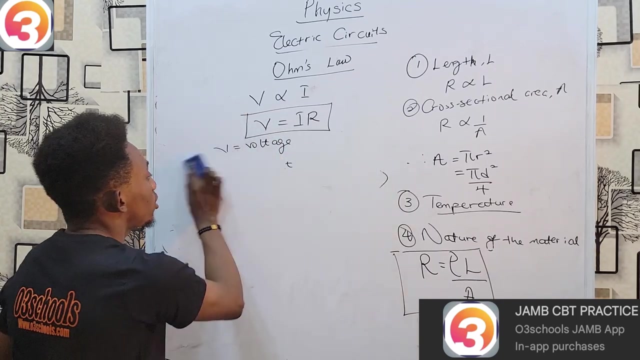 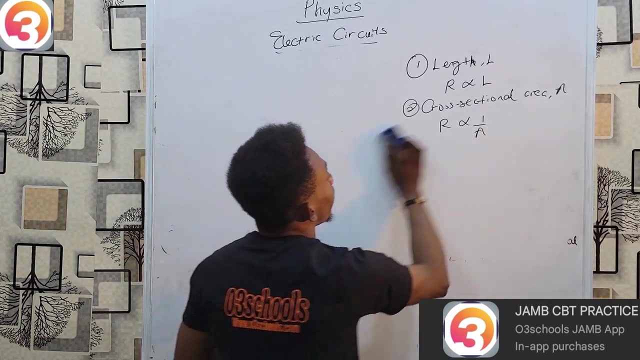 length over the area of that material. this resistivity here is gotten based on the nature of the material. that means different materials made of different things each have their own separate resistivities. okay, so that is that for the basic property of your resistor. however, these resistors in circuits can also be connected in more than one way. what if i want to combine? 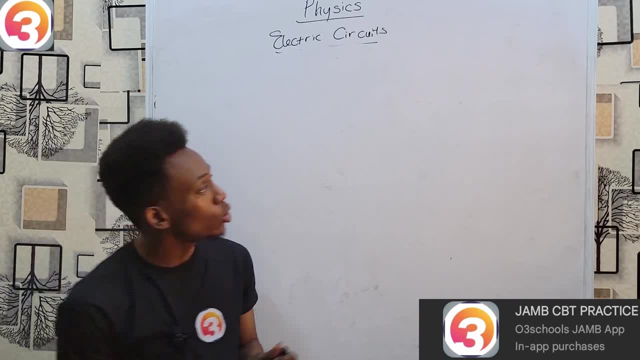 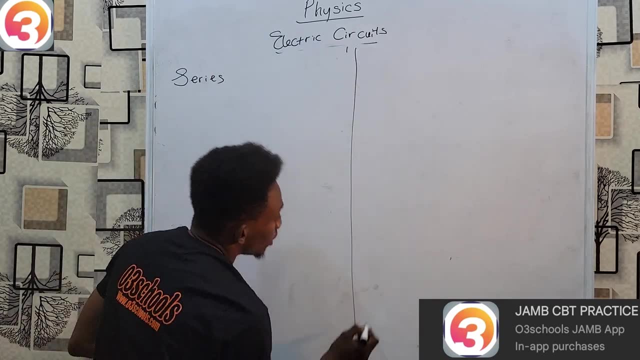 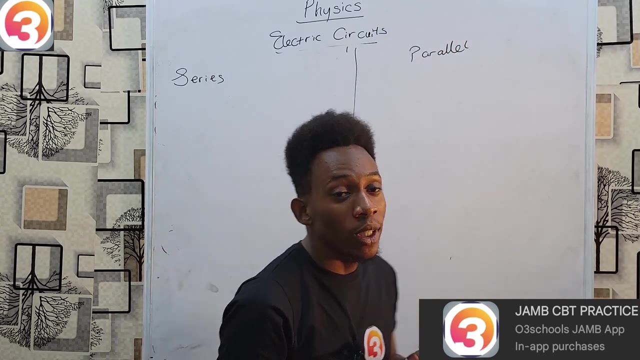 different resistors. that brings us right back to시: both the series and the parallel connection. now, please keep in mind, a series connection can still be identified for the fact that they are connected head to tail. it doesn't have to be straight. all you have to note is: 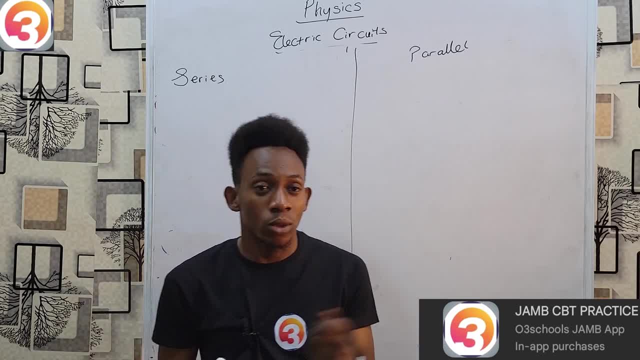 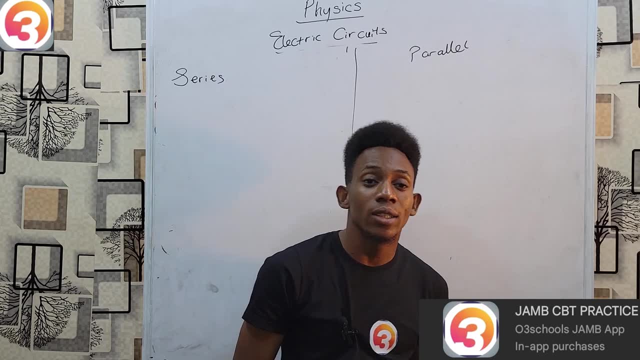 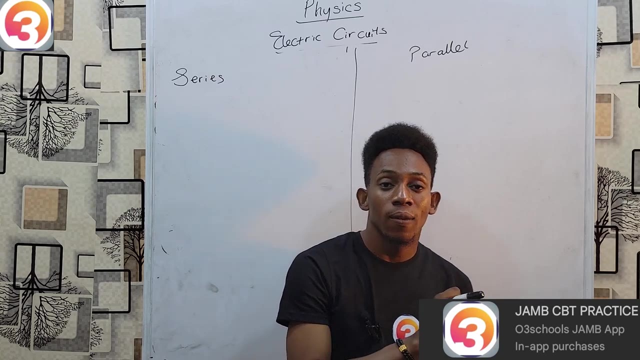 that you have a single wire connecting one resistor on that resistor and on that wire connecting that resistor to the next resistor. a parallel connection, on the other hand, implies that all the wires coming off from one side of the resistor of the resistors are taken together and the wires coming from the 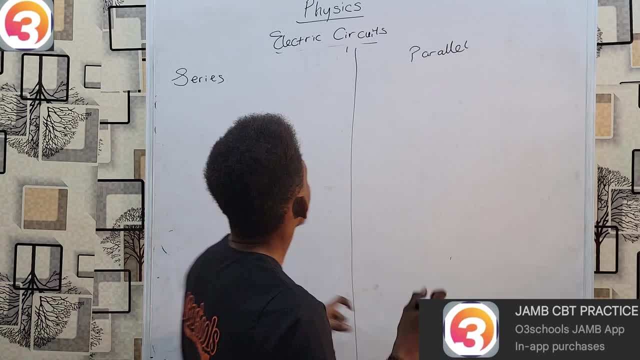 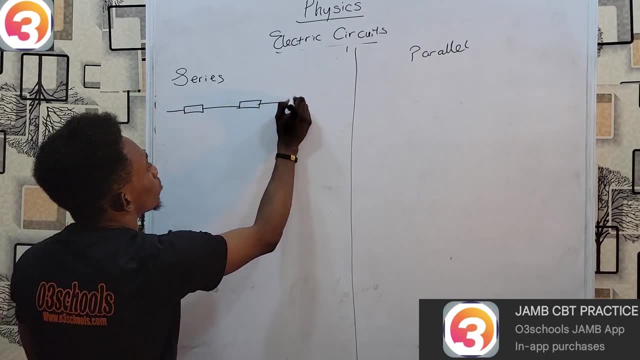 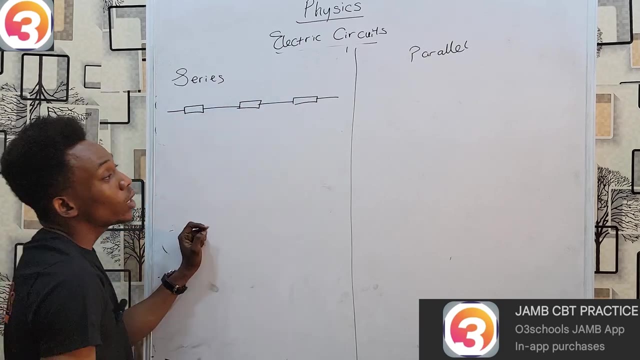 other side of the resistors are taken together, which means a series connection can look like this: see a wire connecting this and this, a wire connecting this and this. on the other hand, for a parallel connection, we could now have two wires connecting consp�� ver. 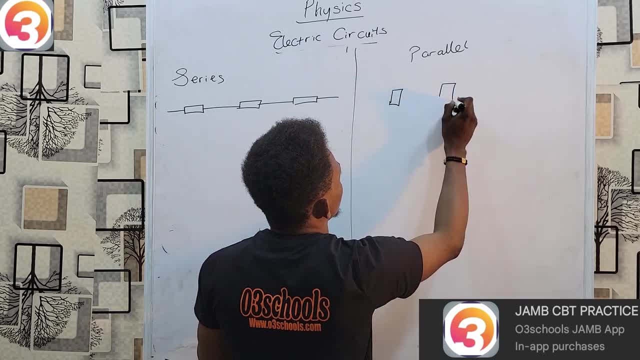 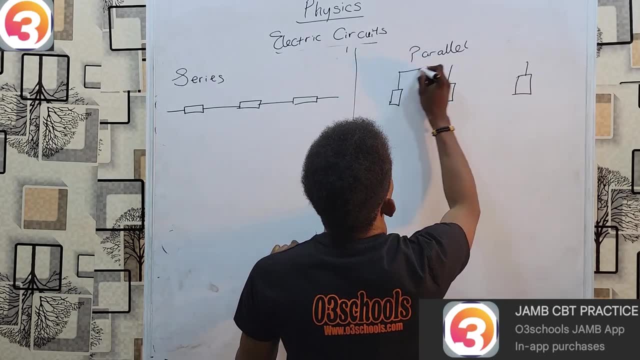 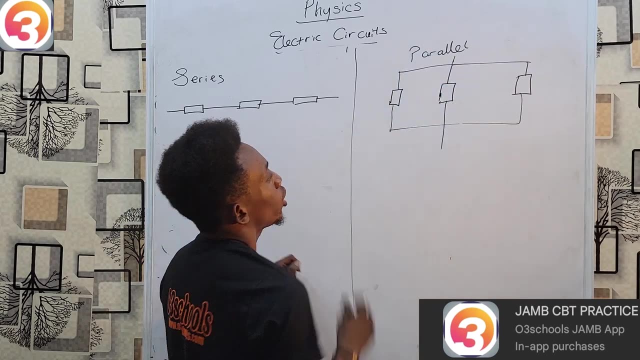 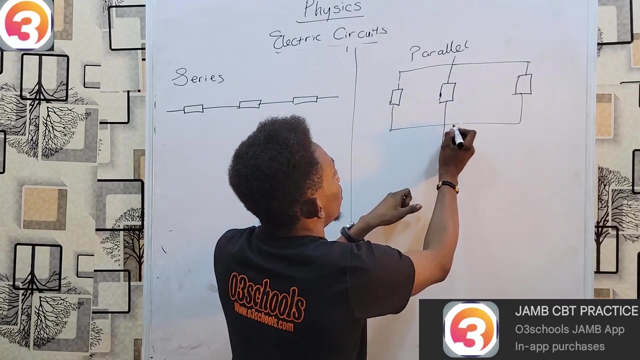 have something like this, and all three of them would then join at the setting point, while all three also be drained. so, as you can see, this is a parallel connection. they all come to join from each other points and join when it's ois connections, just single wire joining them and, as such, based on this, 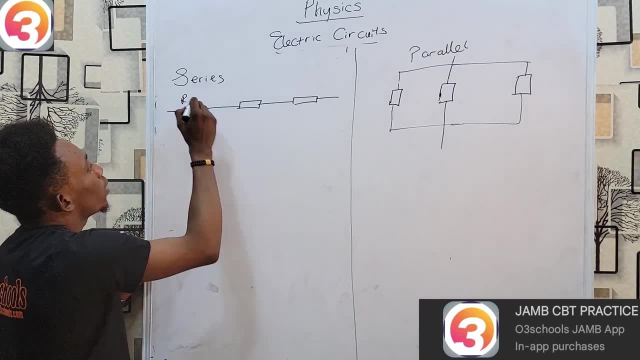 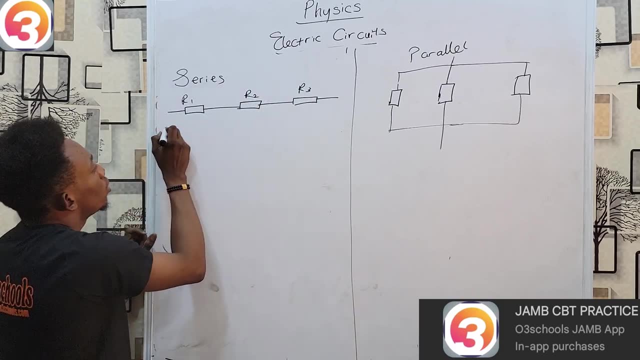 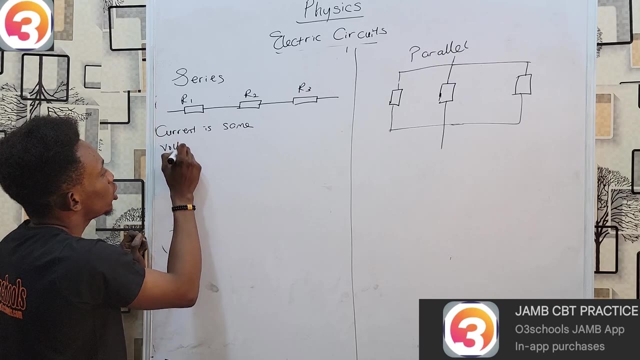 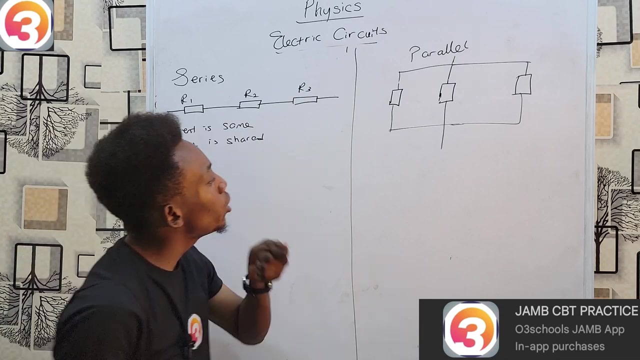 the analysis then differs if I call this r1,r2, and r3,. it must be noted that in a series connection, the current is the same. current is same while voltage is shared. current is the same while voltage is shared. In a parallel connection, current is shared. 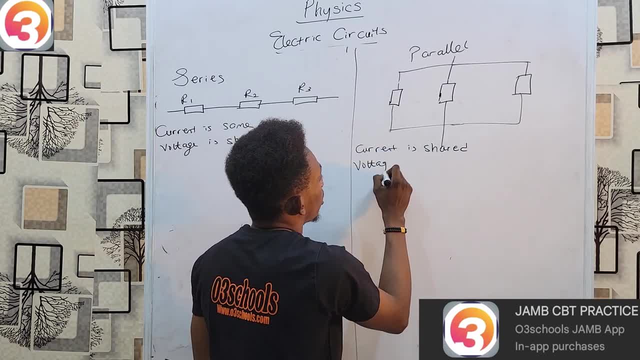 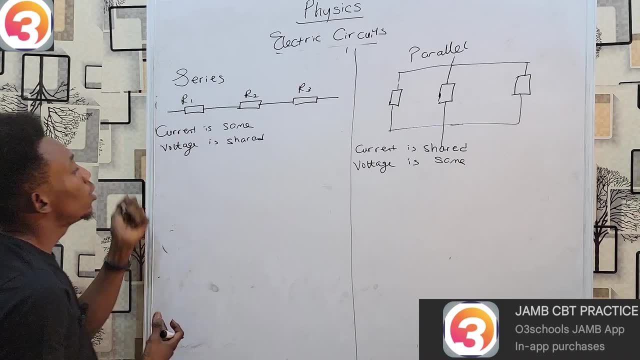 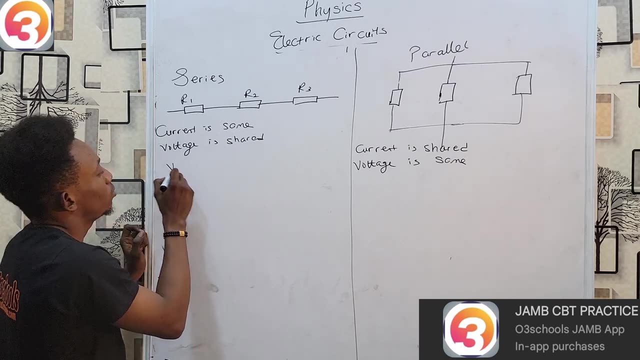 current gets shared, while voltage is the same. Therefore, how can I analyze this? Based on the voltage is getting shared, it means each of them are going to have their own individual voltage V1, the voltage in the first resistor will be current, which is the same for all. 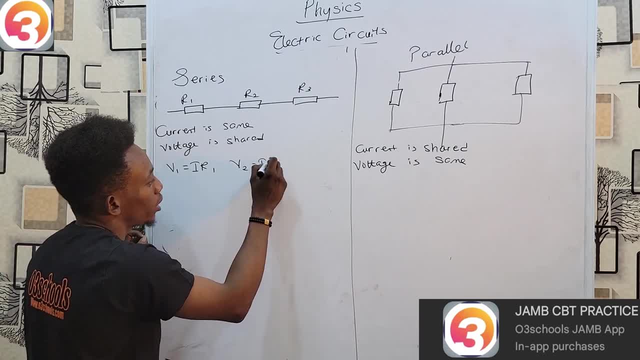 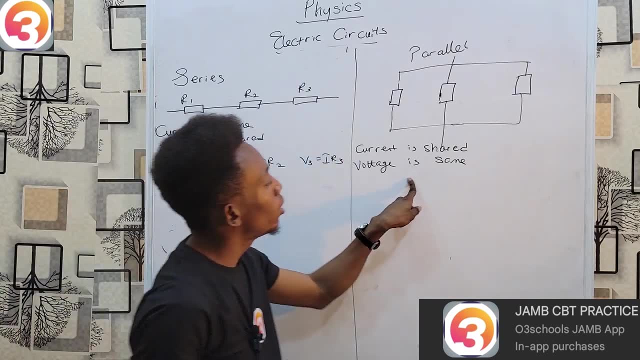 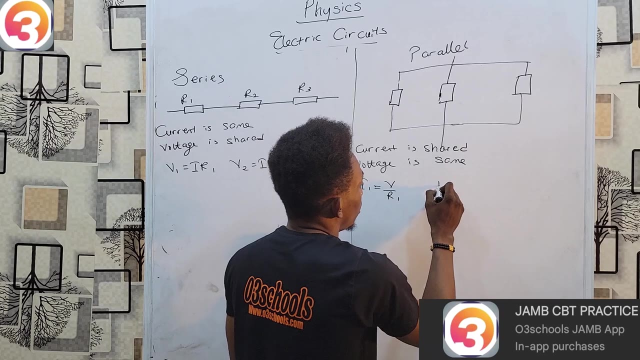 times R1, V2 will be I times R2, then V3 will be I times R3.. While over here voltage is what is the same. Therefore, I1 will be V over R1, I2 will be V over R2,. 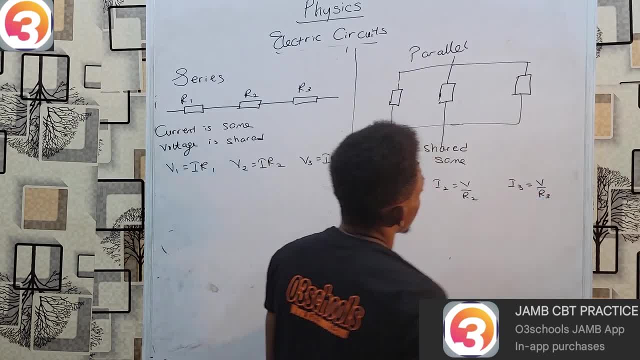 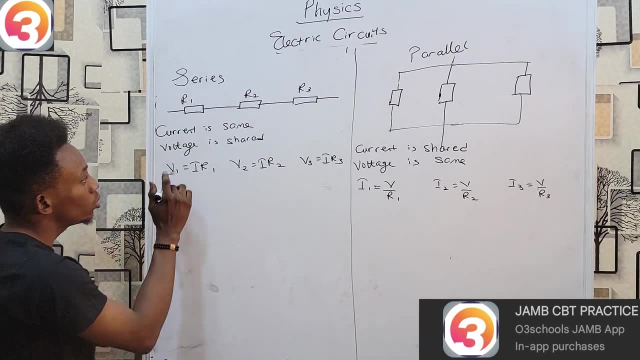 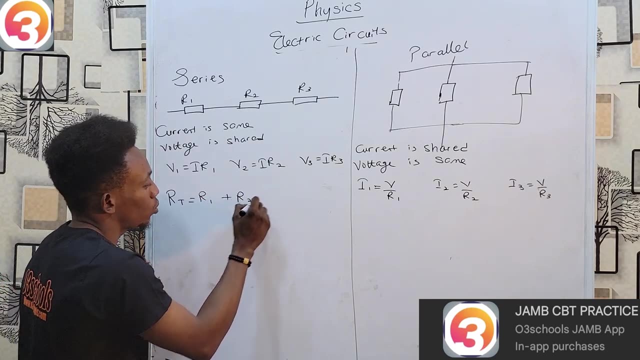 I3 will be V over R3.. Next up, we did a bit of proving, which we do not truly need for the properties of our jamb. We must then know that the total resistance in this circuit will be R1 plus R2 plus R3.. 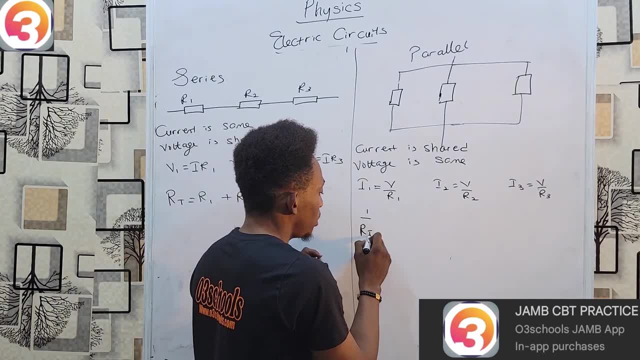 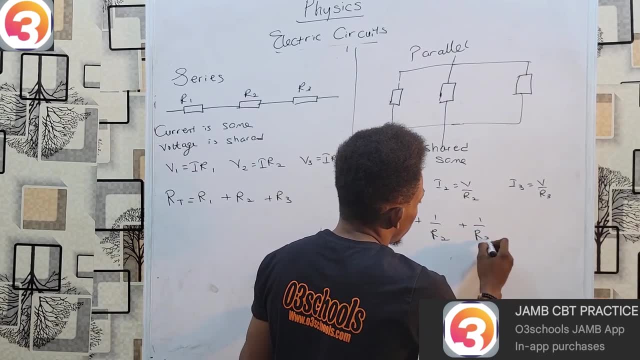 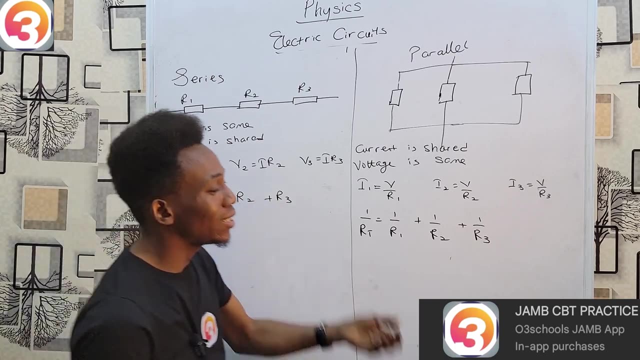 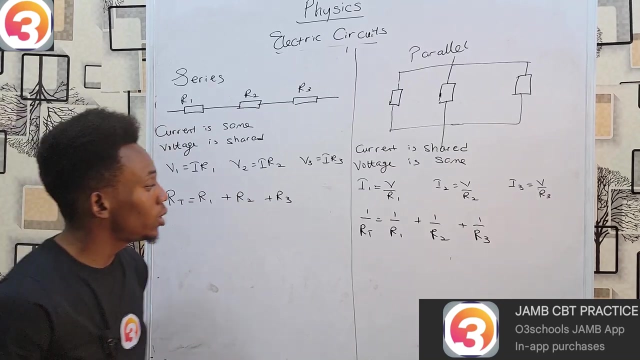 While in this case it will be 1 over Rt plus there is one overило R3.. And these are the different formulas for resistors in series in parallel. okay then, once this is noted, the next one was they look at is: 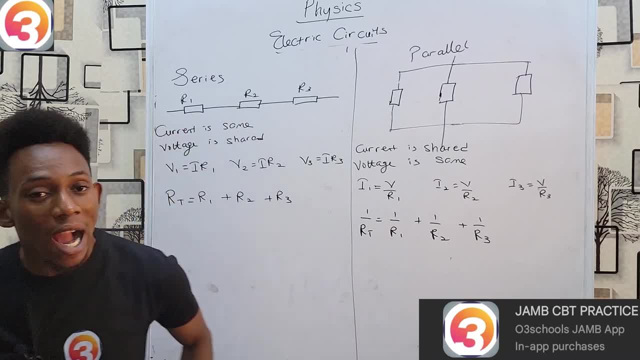 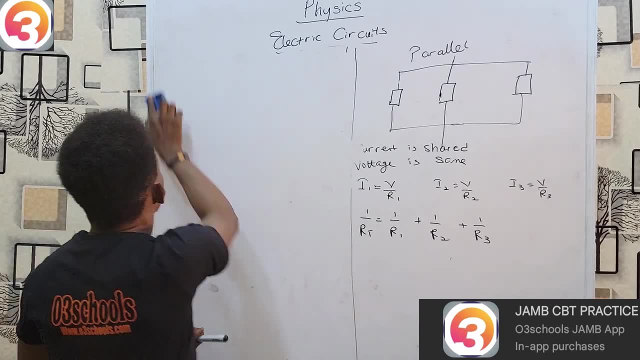 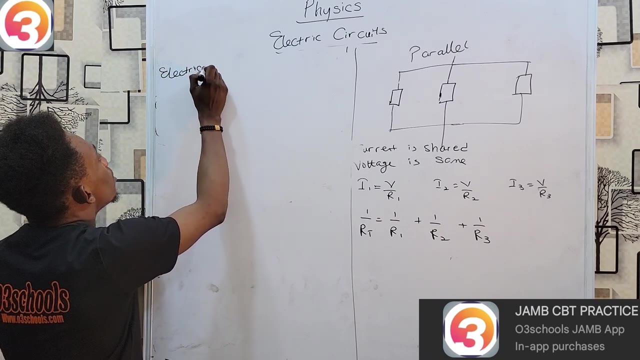 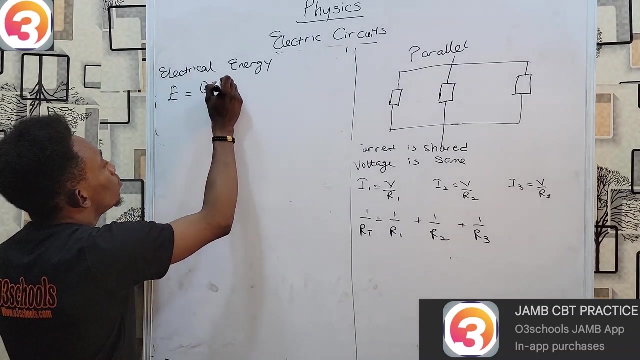 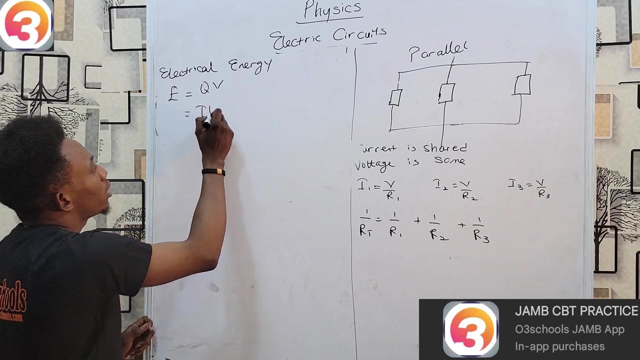 electrical energy and electrical power. energy and power. let's go. energy is easily analyzed for every single system. let's go. energy being generated, the energy I'm giving us. e equals to Q, V, because energy equals to walk, if you recall, and charge is going to be current, thanks time, times. voltage for energy is 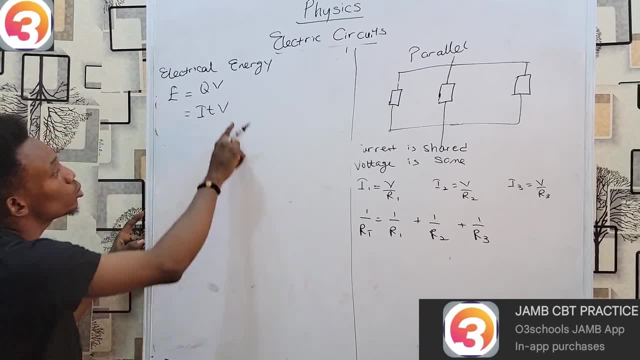 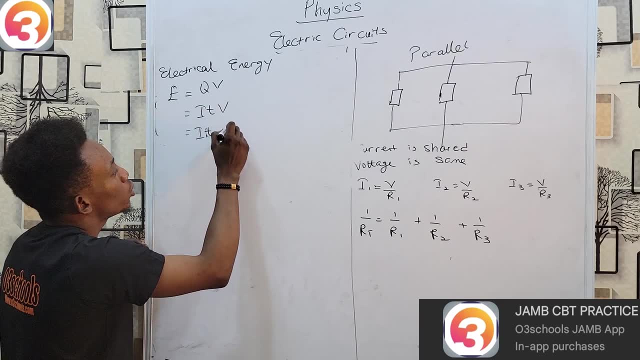 coastal I TV, but there's also from homes. low V equals to IR. that would be I are. I see a festival. that is view which is going to be I, our items eyes. I See a festival that is view which is going to be I, our items eyes. I squared our see, so that's one. 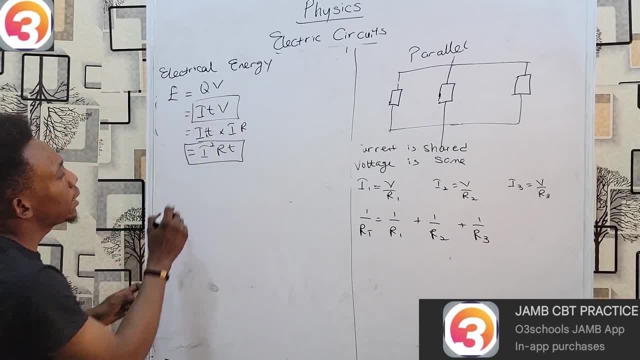 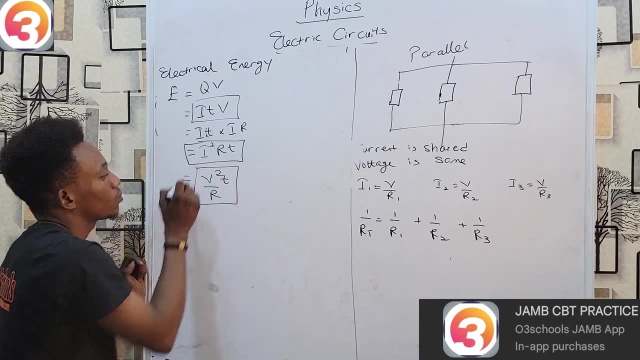 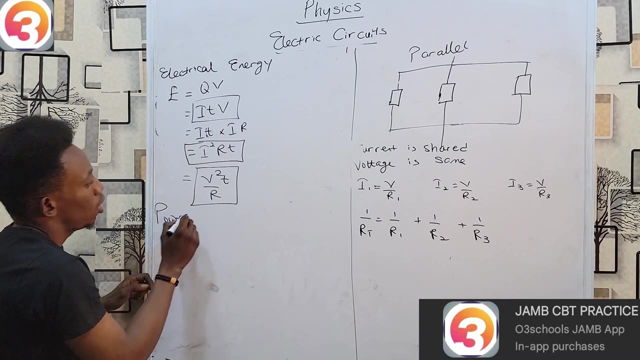 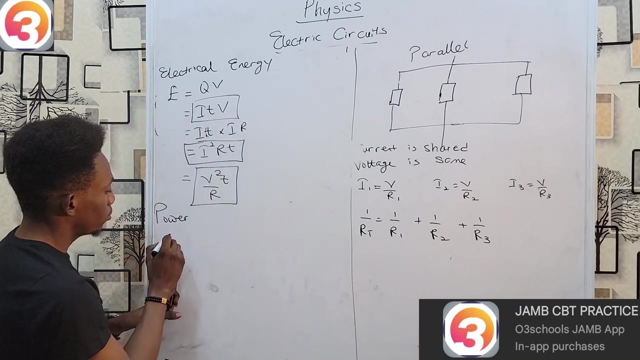 formula- this is another formula, and it is a 10 one- which is that energy equals to V squared C over R. so any of these will help you get your energy, while for power, power is always simply equals to energy over time. and therefore how I shall be coastal that that semi-see goes away? ivy, but by time I squared our and again. 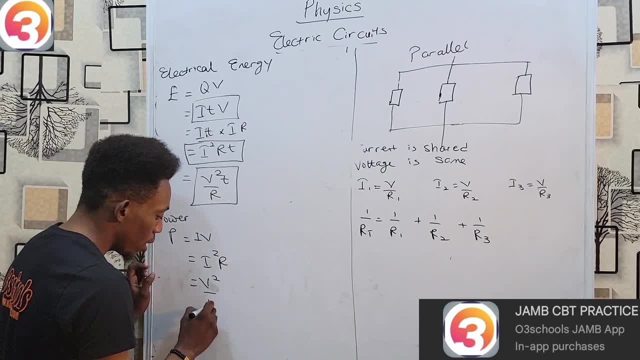 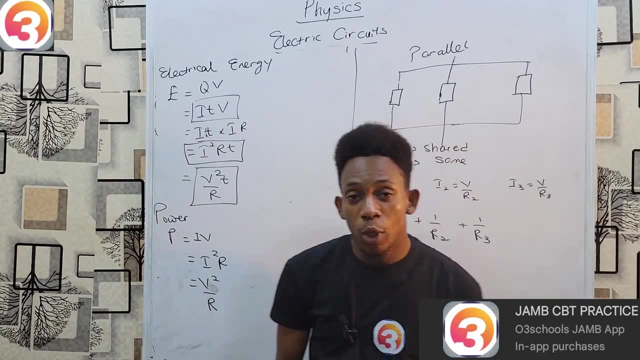 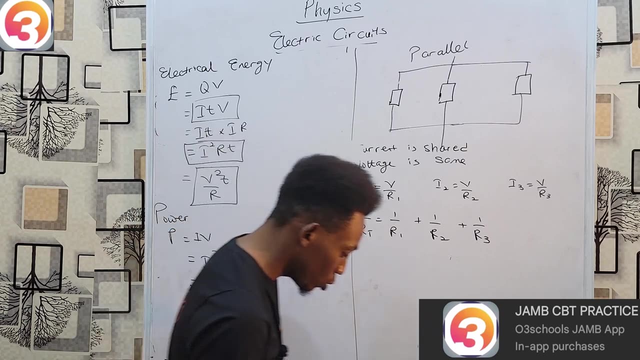 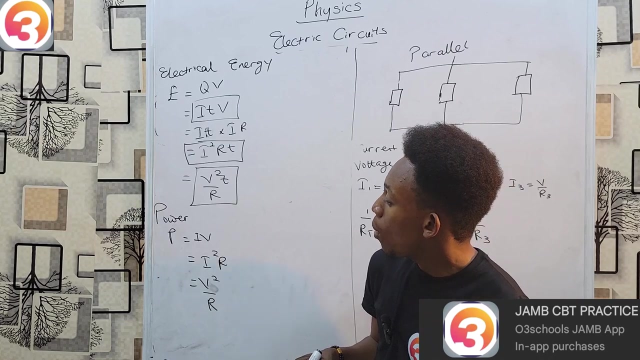 is very bad time. this squared over our means when edges juice, but then for power is wax was should be noted that when calculating the cost of electricity, electricity generated two houses as any measured in terms of kilowatts or R, not joules. To get it in kilowatt hour, all you have to do is convert your power. 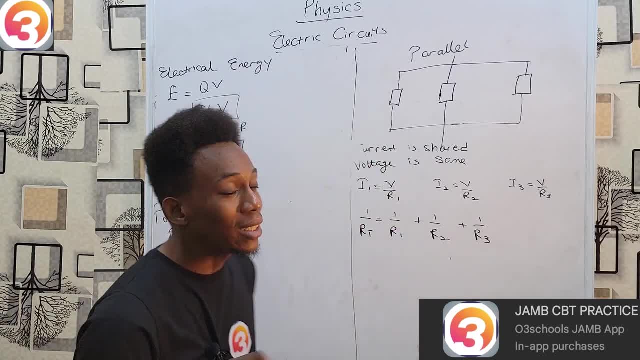 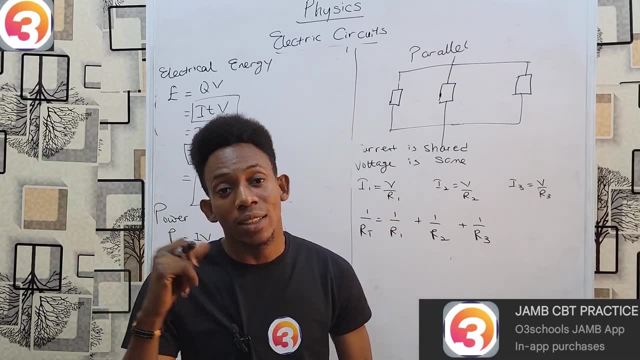 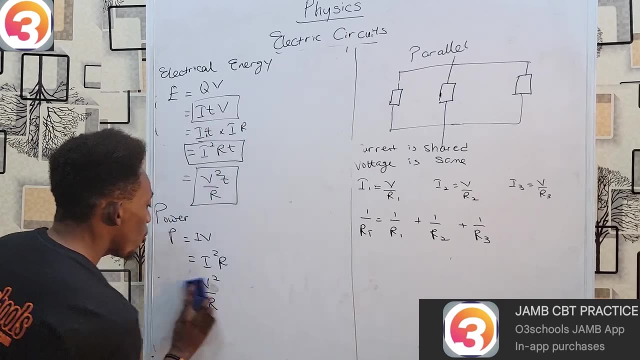 from watts into kilowatts and then multiply by the time in hours. That will give you how much energy you've consumed in kilowatt hour, and then you can multiply that by whatever rate is given to you in the question, And with that I believe we can now move on. 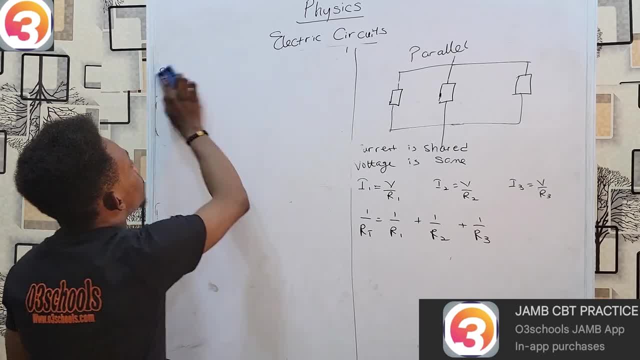 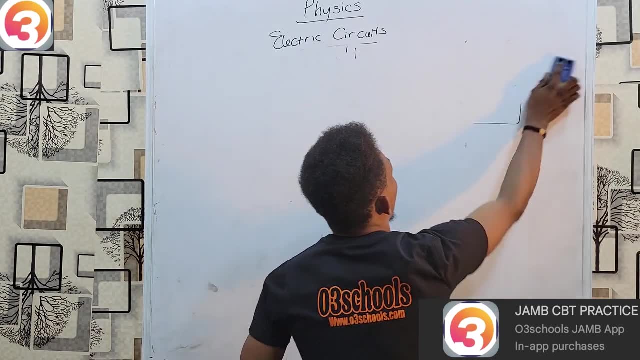 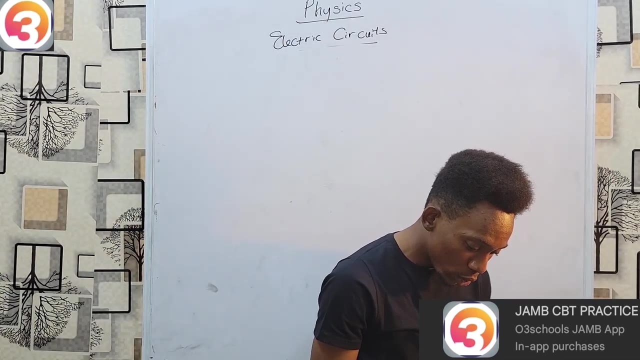 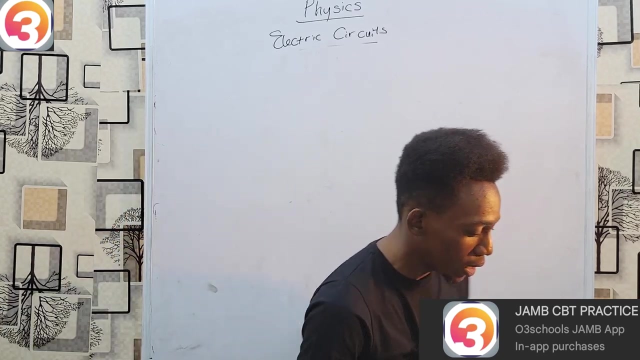 to our O3 Schools jump app from which to sort out several questions having to do with this topic, and we can solve and analyse. So let's get out our apps. Remember, your app has to be activated to enjoy this range of features. Our first question will come from 1995, question 34.. 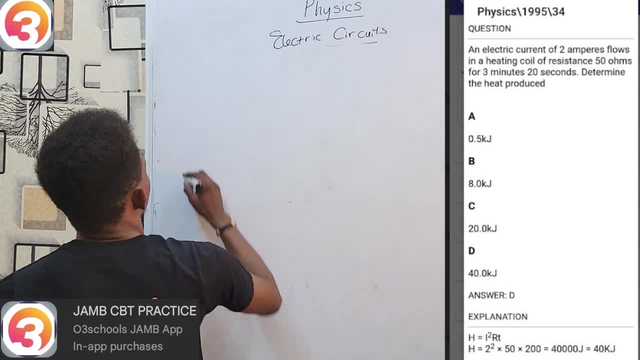 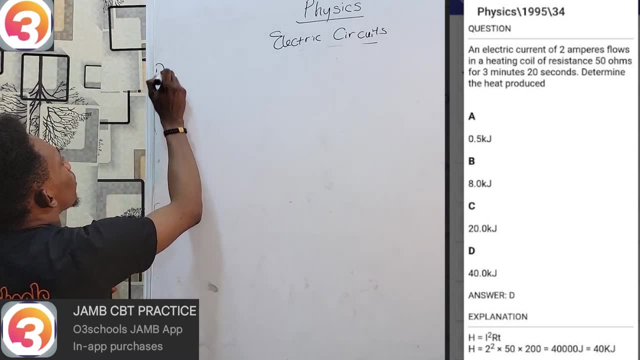 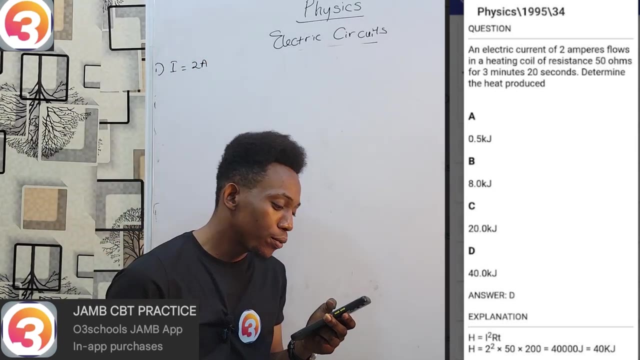 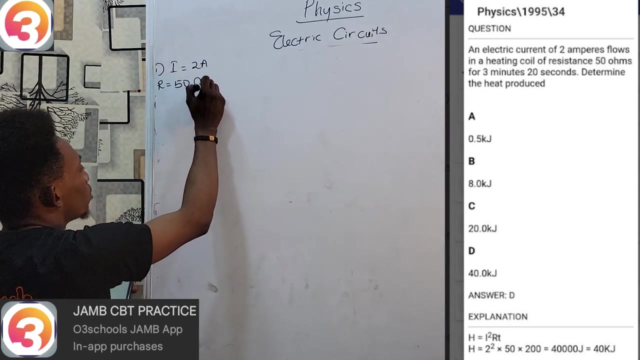 The year 1995, question number 34.. And this question simply states that an electric current of 2 ampere- and my current i equals to 2 ampere- flows in a heating coil of resistance 50 ohms. resistance is 50 ohms for 3 minutes 20 seconds. 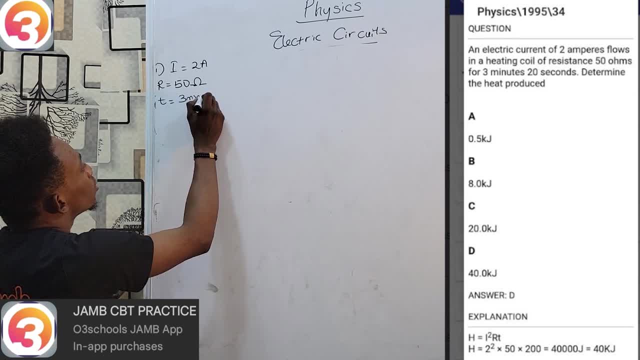 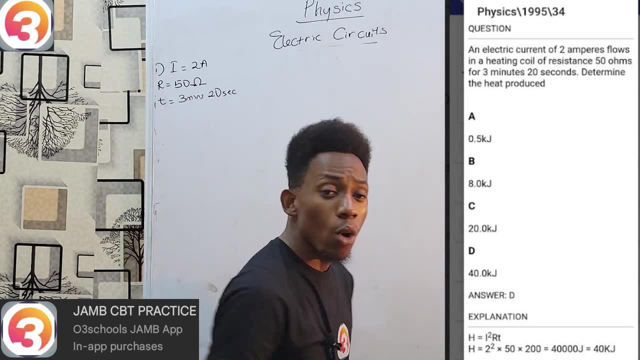 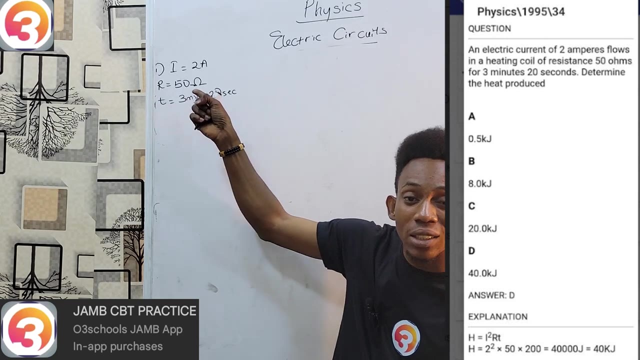 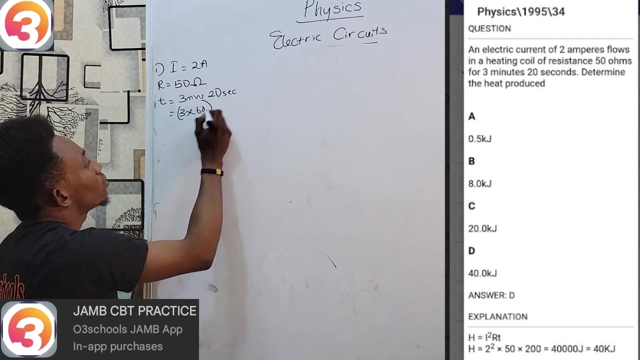 and the time is 3 minutes 20 seconds. well, to find the heat produced now, all you have to remember is well for energy right now, and we don't solve our power to for energy with our time in minutes. it has to go to seconds. how do i convert this to seconds? that becomes 3 times 60. so this is 20.. 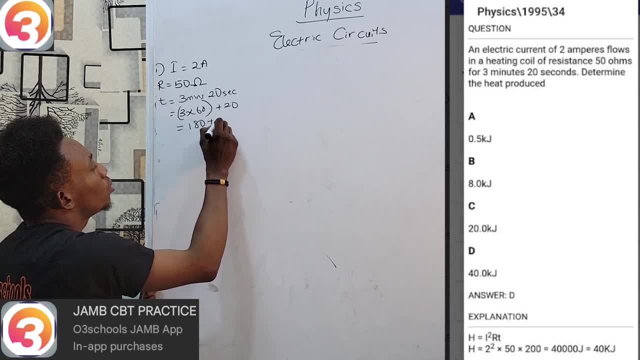 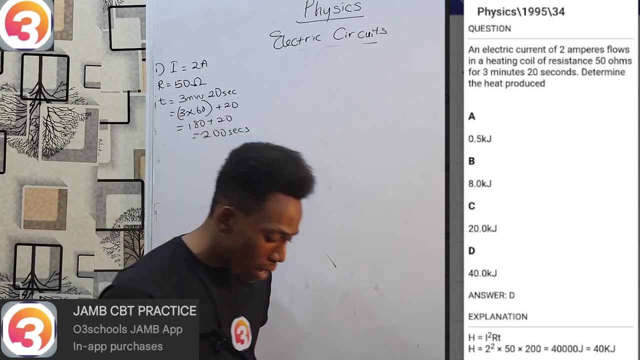 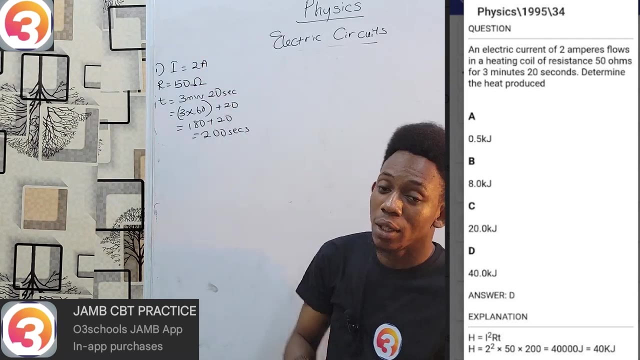 3 times 60 is going to be 180 seconds plus 20 seconds, and that is 200 seconds. now to get my energy, i have about four formulas for energy. i simply have to find one that makes use of i, r and t and, if you can recall, 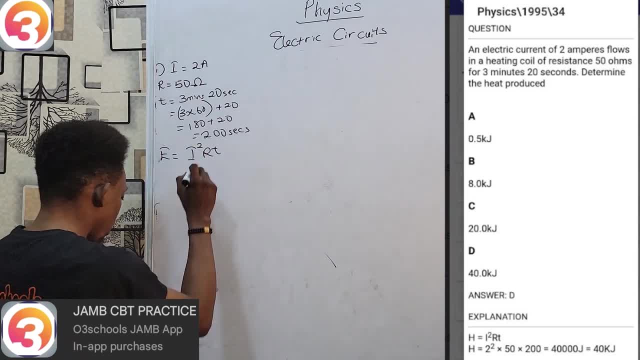 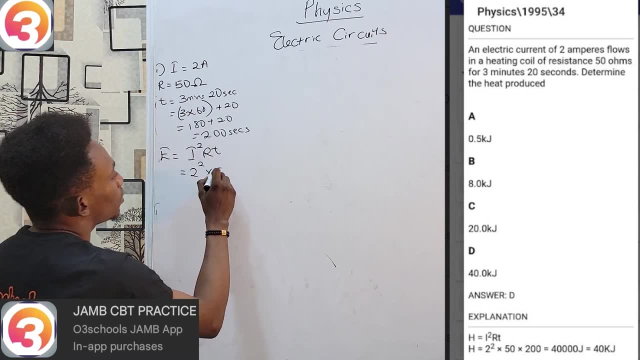 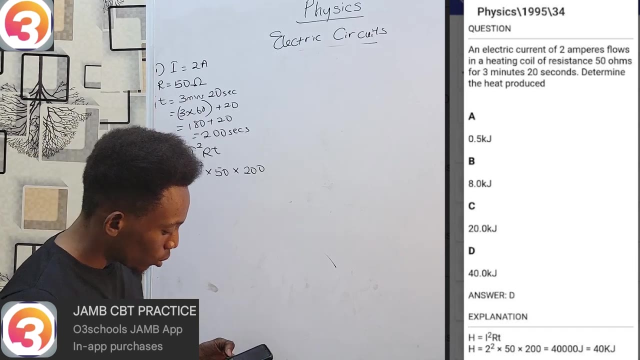 that formula is given by i squared r, c. so my i is 2 squared, my r is 50 and t is 200.. i remember we have to get our size now calculator. so if you open your calculator, two squared is four, four times fifty times two hundred. 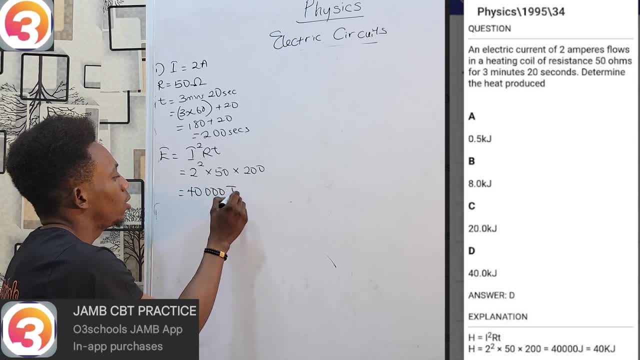 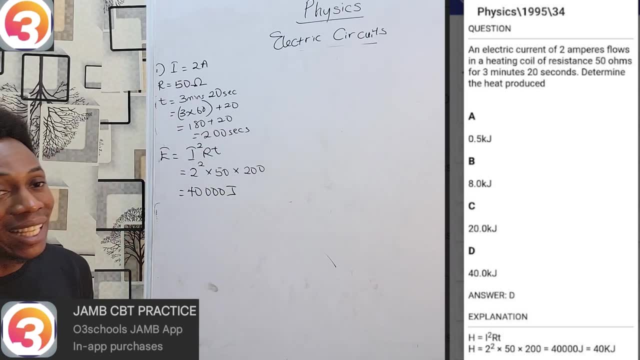 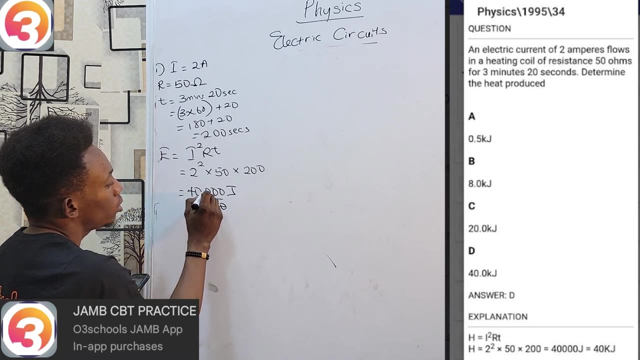 and that gives you forty thousand jewels, but if you take a look at your options, i just got 40 000 there. all my answers are expressed in kilos, so, as we have to divide by 1000, mix, three, three zeros, take care of these three zeros. 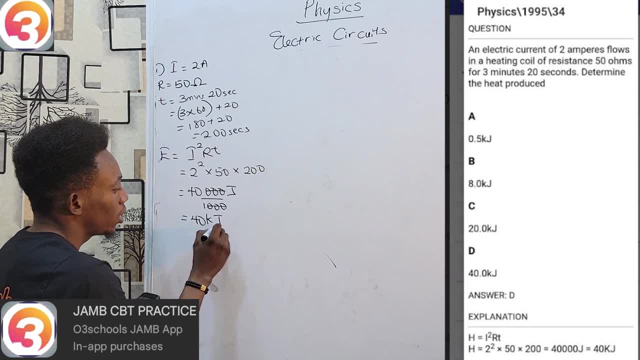 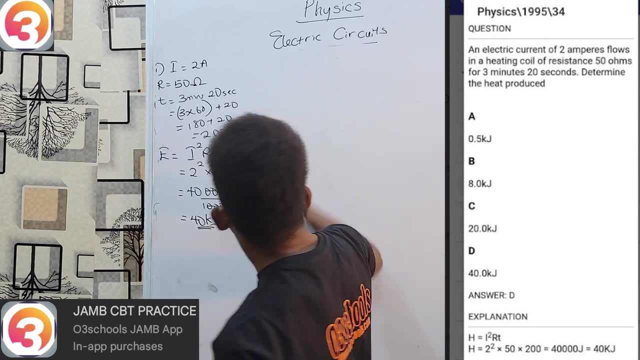 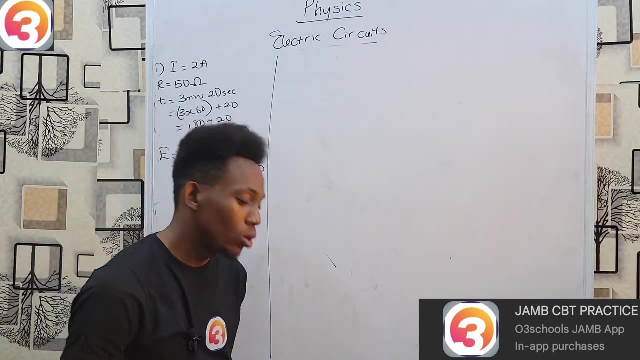 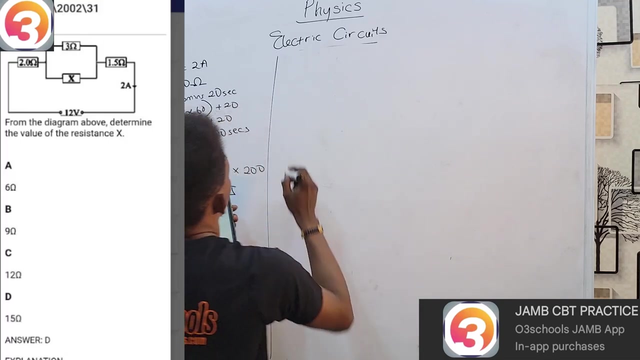 my energy is going to be 40 kilojoules and that is all. i hope there's no problem with that so we can move on to a second question, still using our o3 schools. jump up. we're looking at 2002, question number 31, and in this question we have a circuit i'm going to draw. 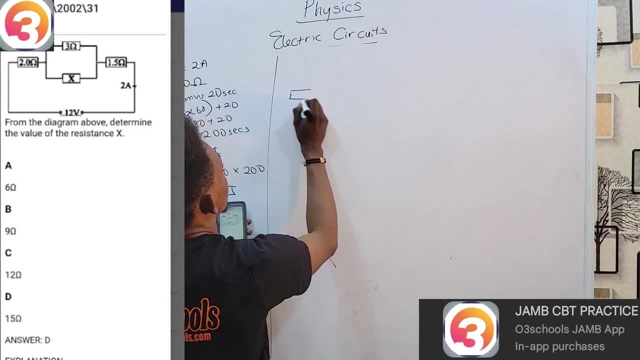 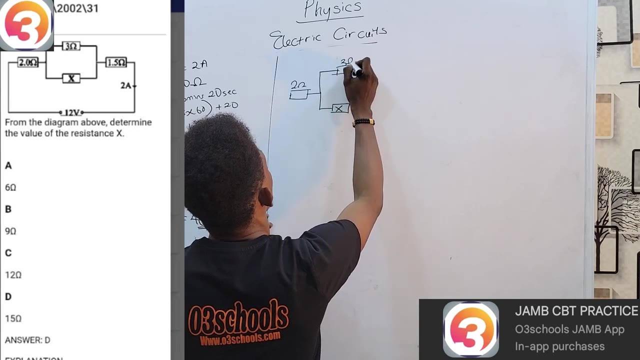 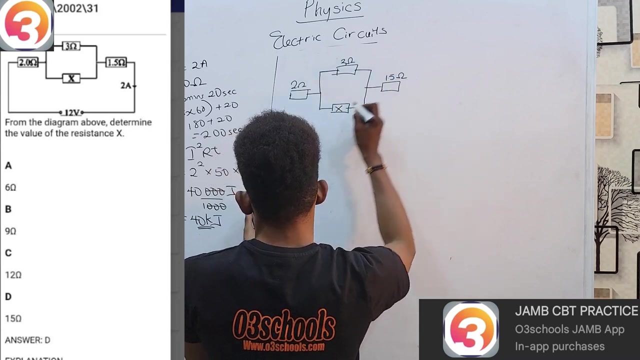 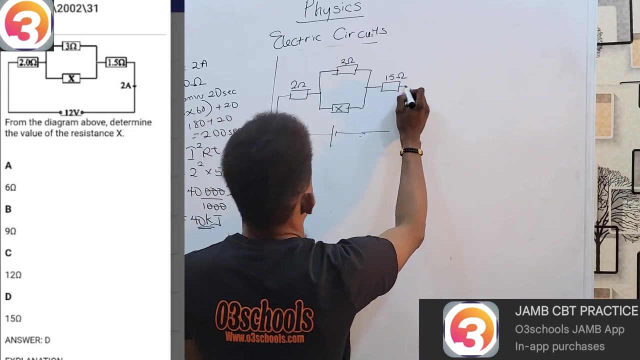 the circuit so we can analyze together my circuit. there's a resistor on this side, two ohms connected to these two resistors, one is x and the other is three ohms. so or connected to a voltage of 12 volts and we are told that the current is two ampere. 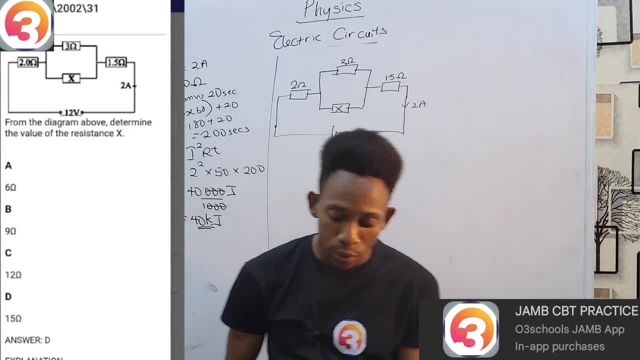 we are told from the diagram above, determine the value of the resistance x, and from a steady point of view, this might seem complicated, but reality. all you have to do is to measure the current of this resistor, and it's hadn't driven one. this resistor, jay be here. 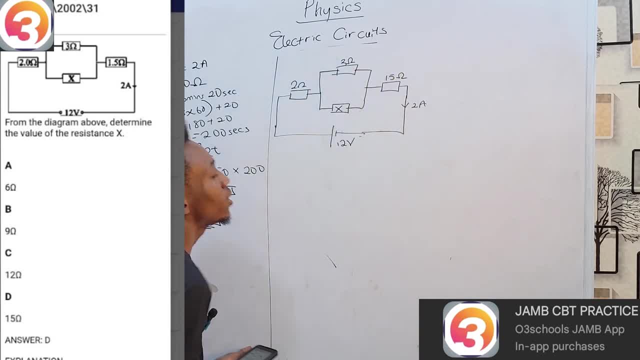 we're going to look at the current point of view and this might seem complicated. so we're going to look at the current point of view and this might seem complicated, to find this value of X. now I can't find the value of X. I know my voltage, I know. 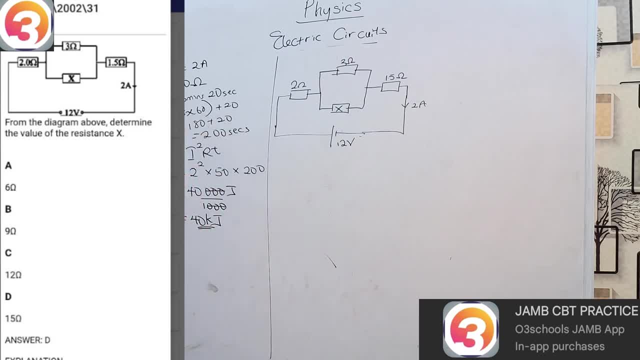 the current passing through the circuits. now what this tells me is that V equals to R from ohms law and that if I'm able to find this resistance, I would know what this overall resistance ought to give me. that means R equals V over I, and V is 12. I is 2. that gives me 6 ohms. that means, if I combine all these, 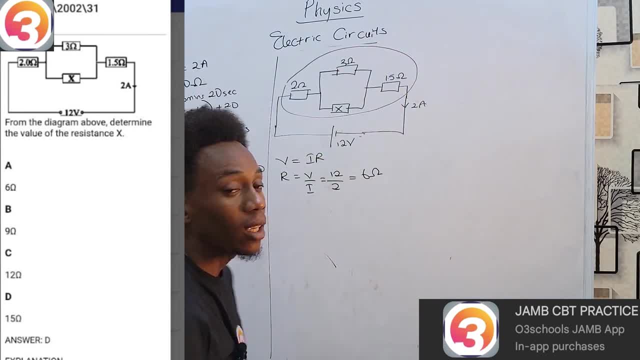 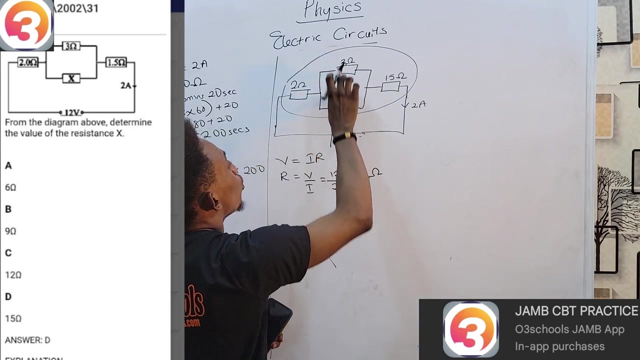 resistances together, I should be getting a resistance of 6 ohms next up. this is what type of connection is a combination of both series and parallel connections. these two are parallel to one another, but in series with the entire system. if I can reduce these two to a single resistor, which I may call A, then I 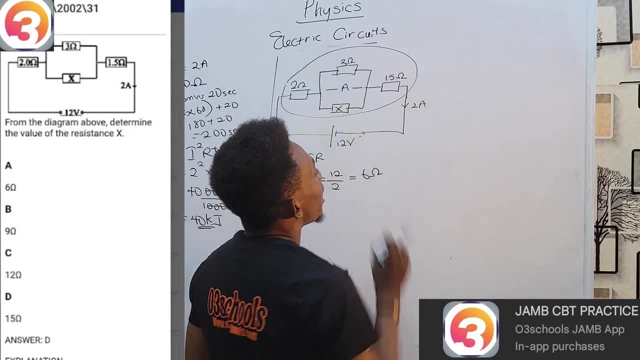 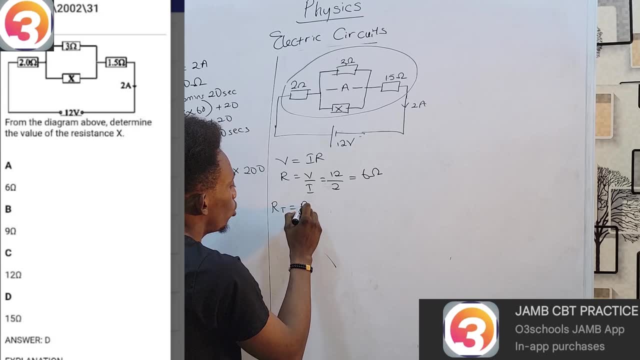 will have that 2, A and 1.5 would all be in series. as I'm aware, for a series connection, R T equals to R 1 plus R 2 plus R 3. therefore I know that my total resistance is 6. you can see, R 1 is our first one, that's 2. 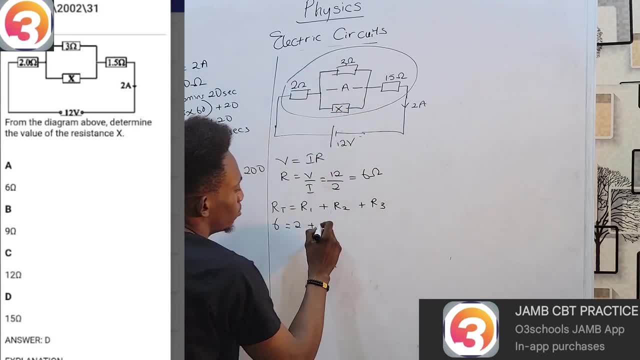 I wrote. so is this unknown? II. an R 3 is 1.5. so now give me that 6 equals 2, 2 plus 1.5 is 3.5 plus a. take 3.5 the other way: A equals to 6 minus 3.5. so A equals 2.5 ohms. and keep in mind we are not yet done. 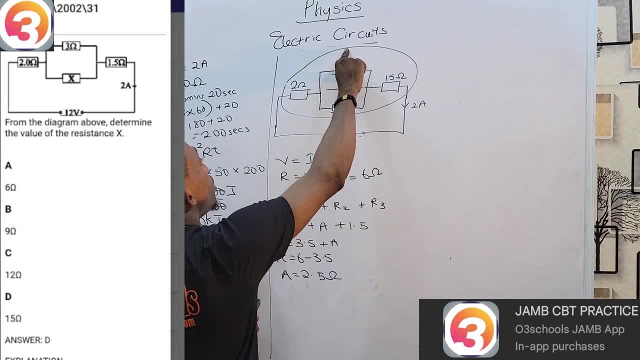 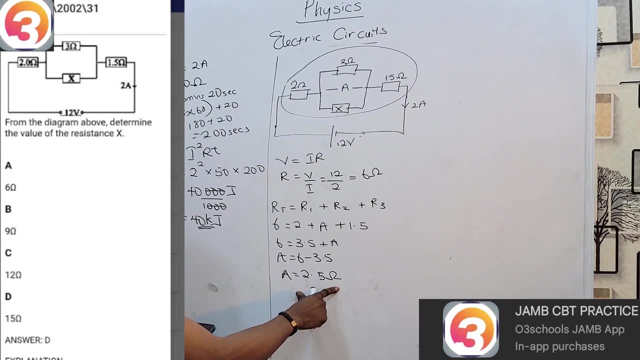 what we know is that the current voltage is higher than the current voltage know. however, though, is that this resistance and this in parallel, when i combine them, i should be getting a value of 2.5, and that's your way for parallel resistances. i formalize that one over. 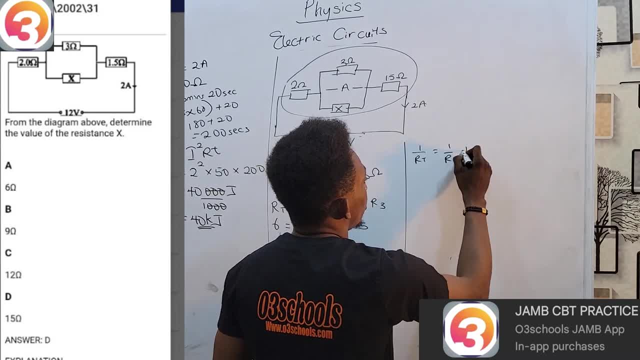 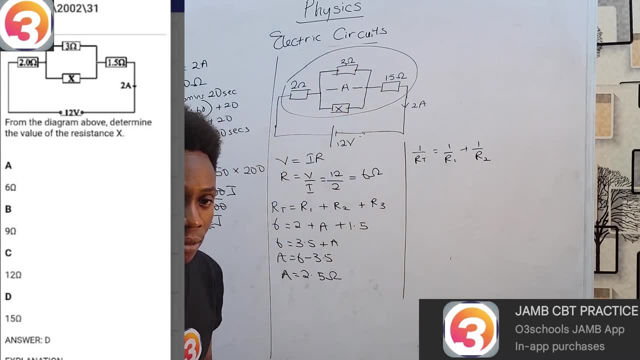 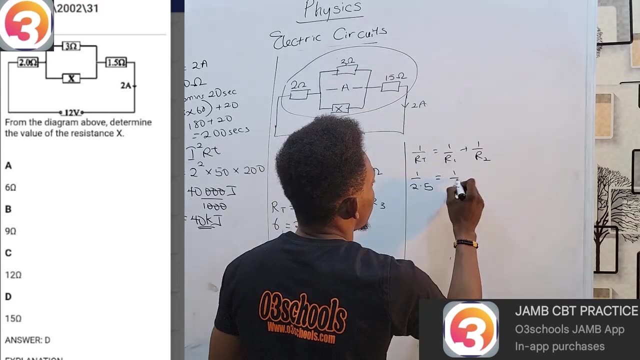 arrow t, plus the one over r1, plus one by r2. i examined my formula there because i have just two resistances i'm dealing with. now. i know that my total should be 2.5 and that my first resistance update is three, so i want to find this one x. 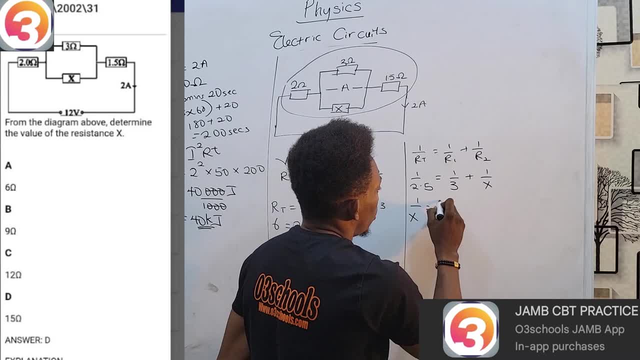 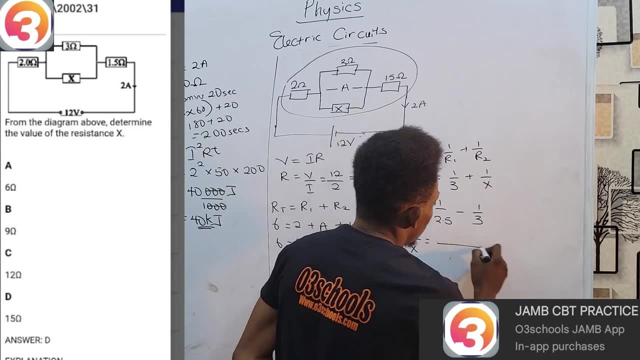 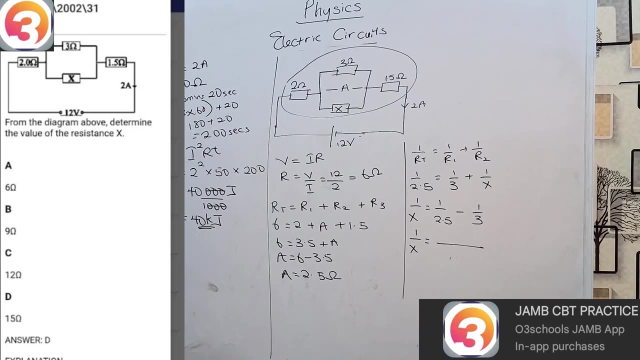 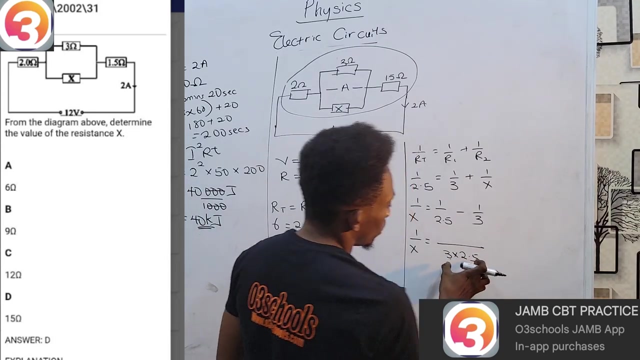 collect items. 1 over x equals 1 over 2.5 minus 1 over 3. now what's the lc move? 2.5 and 3.. that may seem a little bit confusing. in that case, all you simply have to do is multiply them together 3 times 2.5. then, if you 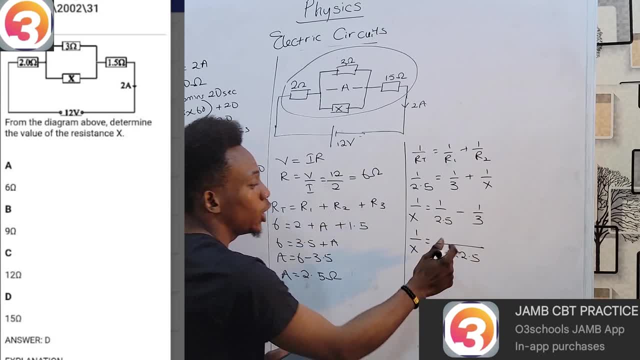 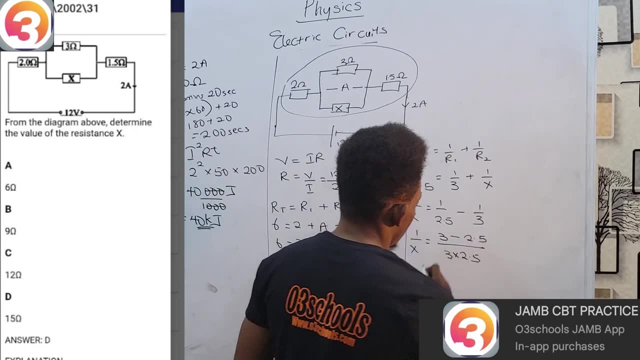 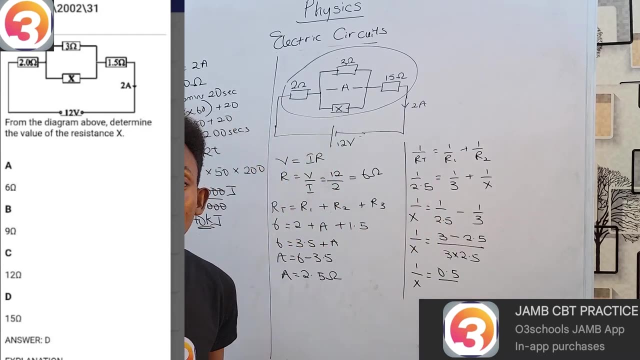 divide by this 2.5 equals 2.5, you are left with 3, and divide by this 3 equals 3, you are left with 2.5. so 1 over x shall be 0.5 over 3 times 2.5, and if you press that in your calculator, you get. 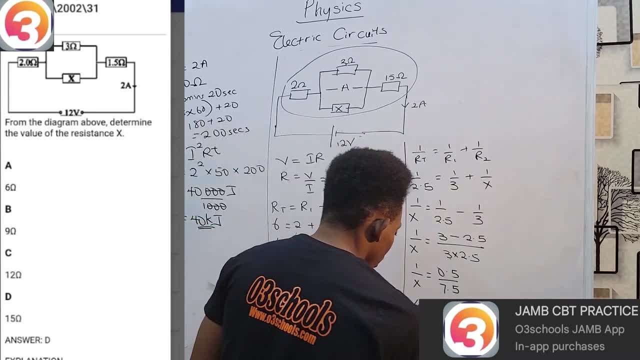 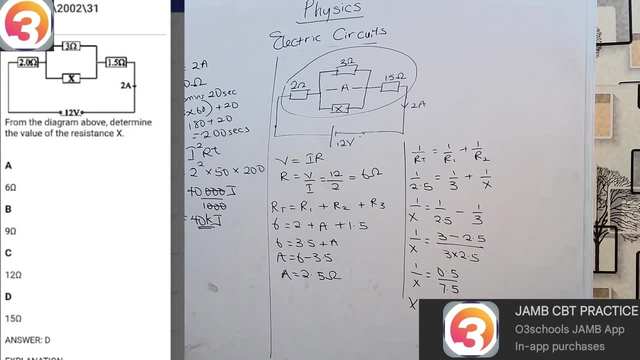 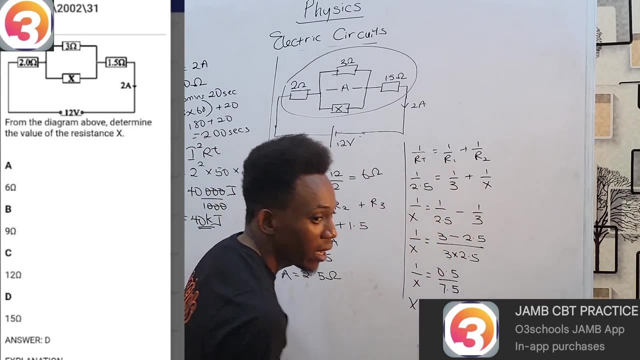 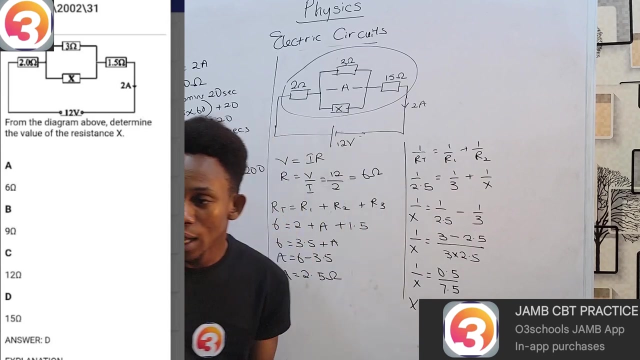 0.5. so my source, both sides x shall be 7.5 over 0.5, and if you divide that using your calculator, 7.5 by 2.5, or rather 0.5, gives you 15 ohms. and that is our answer, option d. 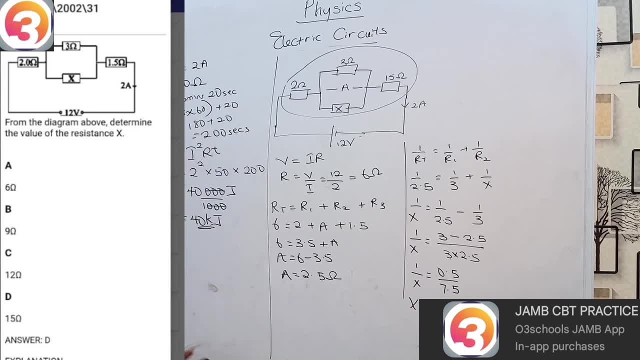 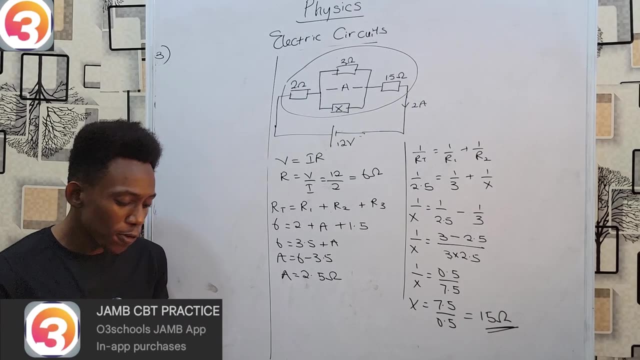 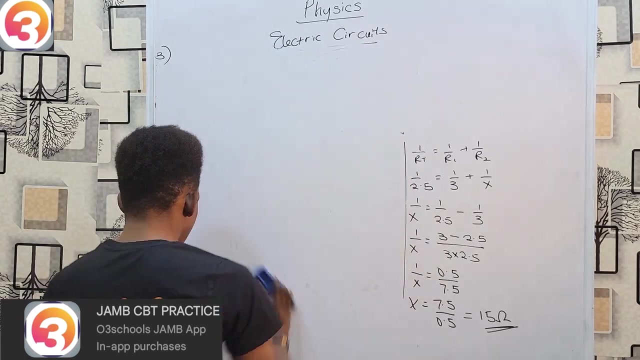 as you can see, the steps are quite simple. understand your basics and apply your steps. all right, go to 2001, question number 32, still making use of our old preschools. jump up 2001, question number 32. in this case, again, we have a circuit. i have simply told then the diagram. 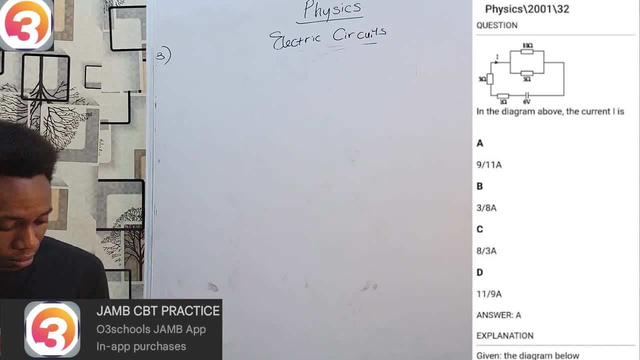 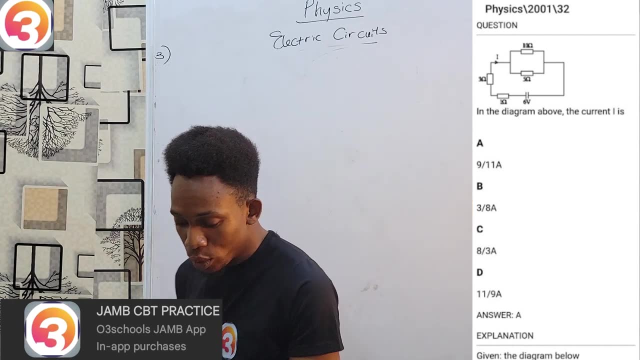 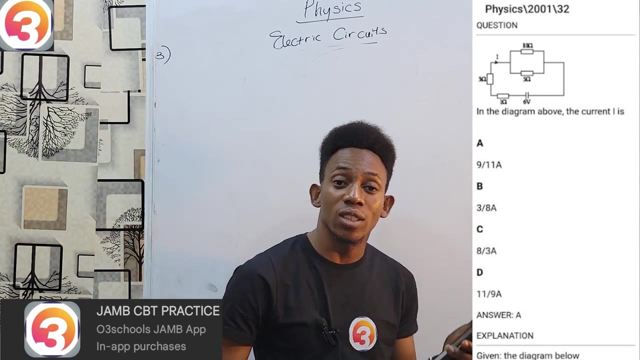 above our current is what now? to get the current as well away? we are giving the voltage at six. now to get our current, we simply need to find out my total resistance and if you look at it, we're having two resistances plus two other resistances in parallel. 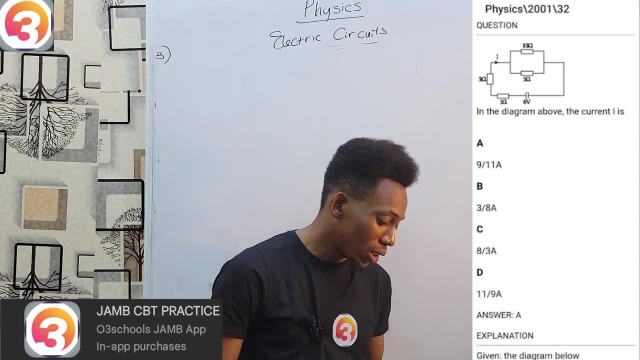 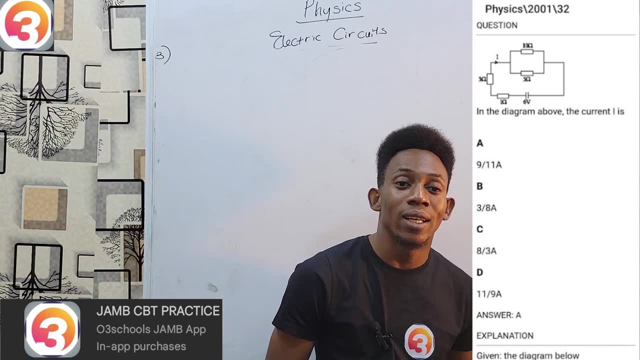 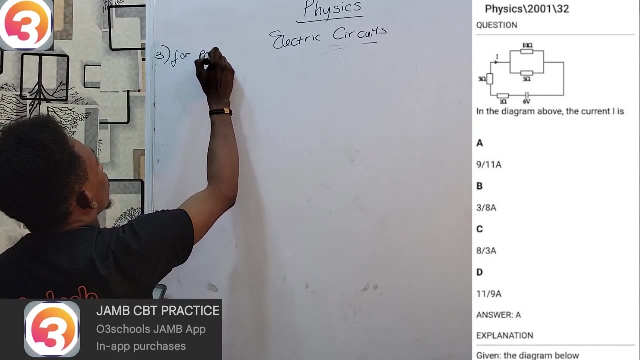 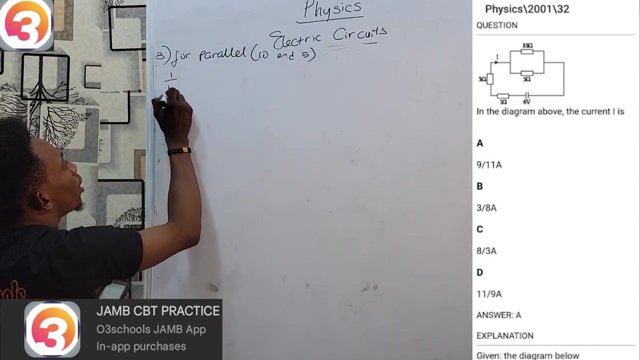 your one ohm and your three ohms are both in series and on the other hand the ten and five are in parallel. so if I can combine everything together up to first of all combine that parallel combination, so I can say for parallel, which I know is 10 and 5, 1 over R will be 1 over 10, plus 1 over 5 and my LCM. 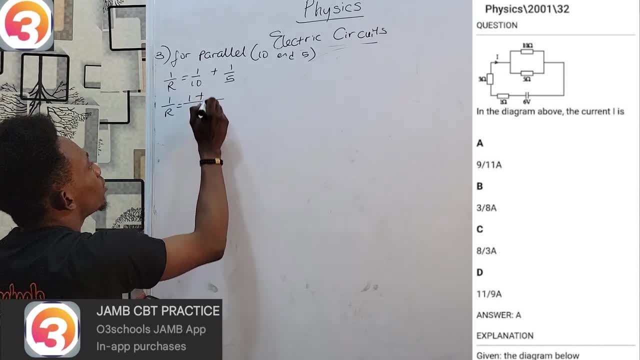 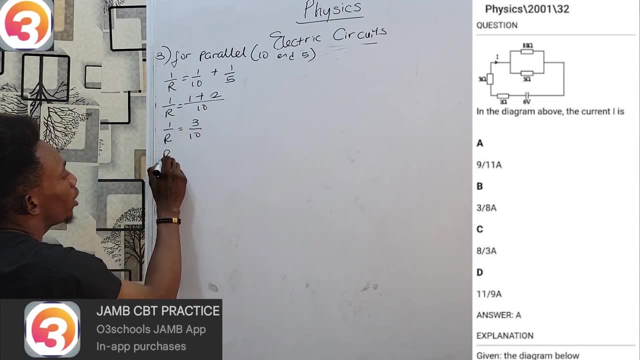 for 10 and 5 is 10, 10 into 10 is 1, 10 to 5 is 2. so that will give me 3 over 10 and when I sum assault our equals 10 over 3, you've made 3.3, 30 ohms and I. 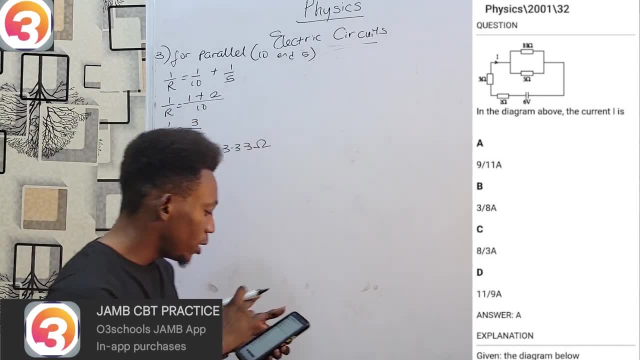 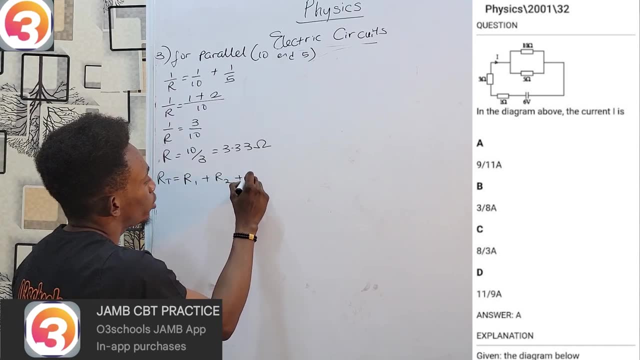 know that those two come back to me 3.33. then everything becomes a series connection. of a series connection I mean our one plus our two plus our three, three. so that would be my one ohm, those three ohms, those three point three, three, one. 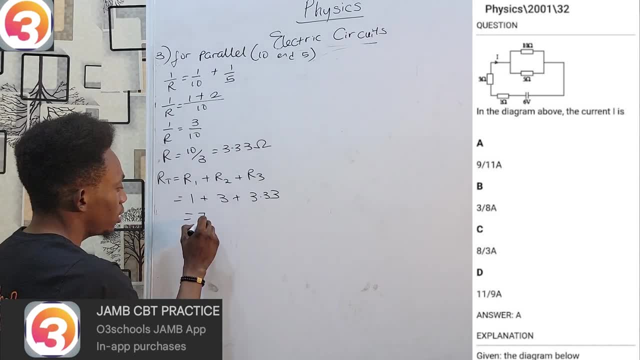 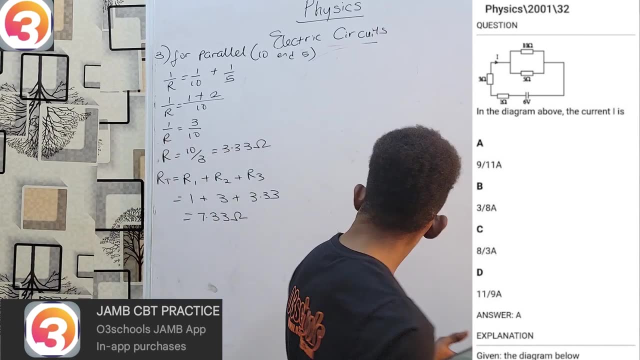 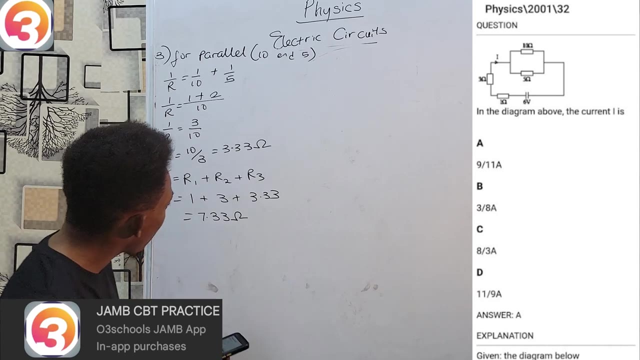 plus three is four or plus three point three. three is seven, point three: three ohms. however, if you take a good look of your options, realize that that doesn't seem to appear my options. so whatever can we do, Danny, all you have to remember is is we are looking for correct, not resistance. do not panic and try to stop. 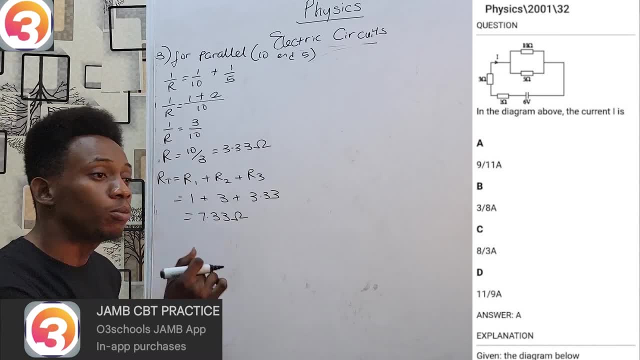 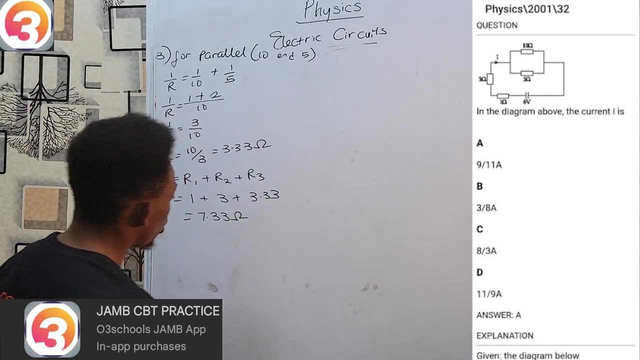 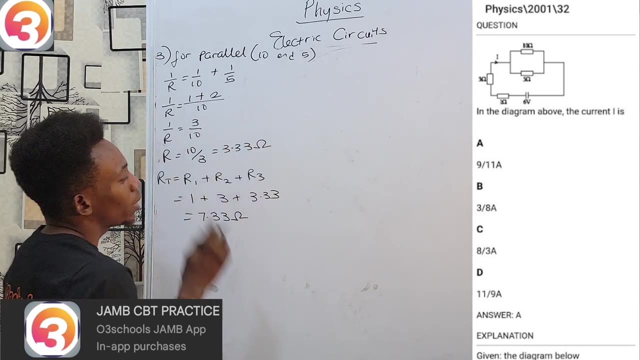 here just because you saw this and you're like: oh no, I'm done. always make sure you ruin your questions with your logical conclusion. the only team of sport right now do is that in your options, everything is in fraction form. but we express, statement our resistance in decimal andチャモ. 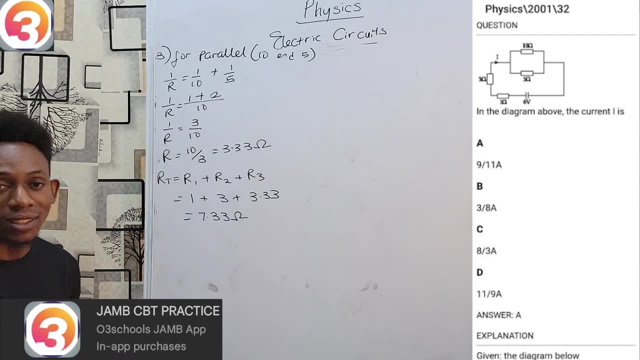 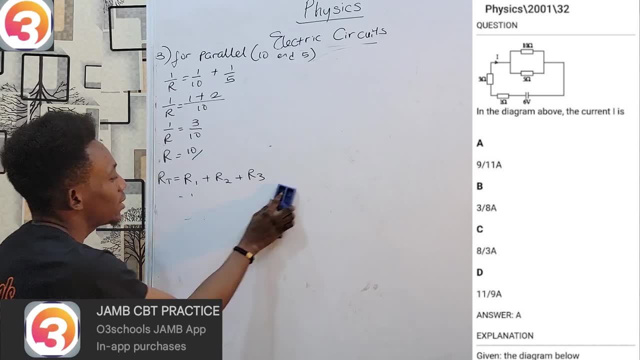 i may not get the same answer appearing as it is in the options. so what do i do? it means i must come back here and decide that i'm going to leave my answer as 10 over 3 oomps and not put it in decimal form, which means when i come back here i will have, as before, one plus three, but now close. 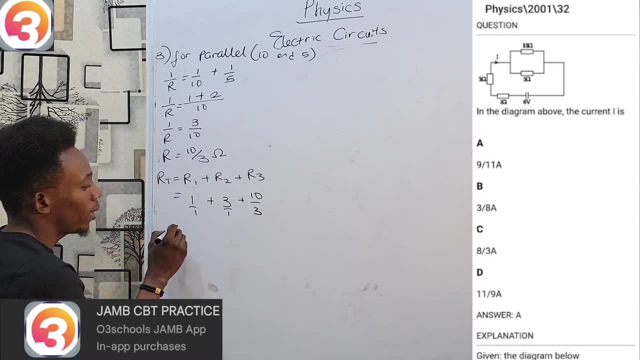 10 over three over one over one. if i take lcm that'll be three three times one is three. three times three is nine. yeah, three into three gives me one. so i have ten. update: three plus nine. twelve. three plus ten. twenty two over three. oomps. see, now i have my assigned fractions so i can proceed. 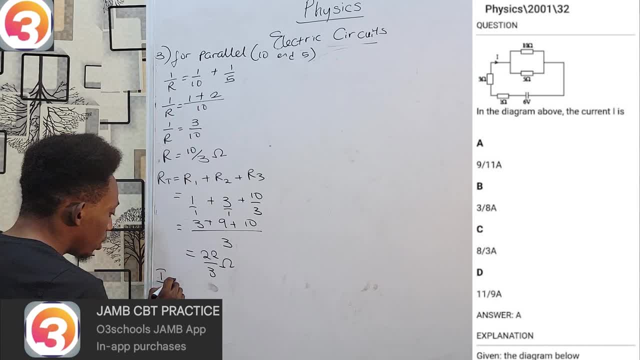 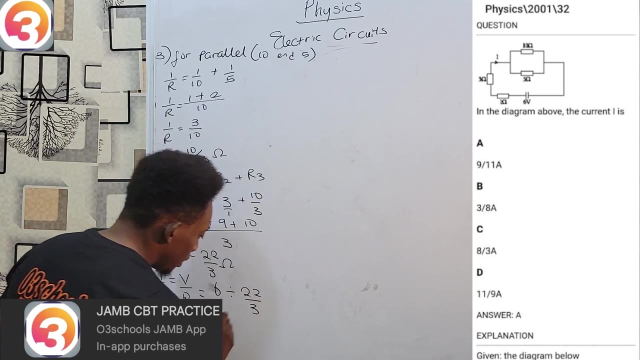 to get my currents. remember working for current all along. i'll be voltage over resistance. my voltage for my circuits is six volts over means divide and my resistance is 22 over three. that gives me six easier knowledge of mathematics. division comes two times and this guy turns around, that becomes three over 22. 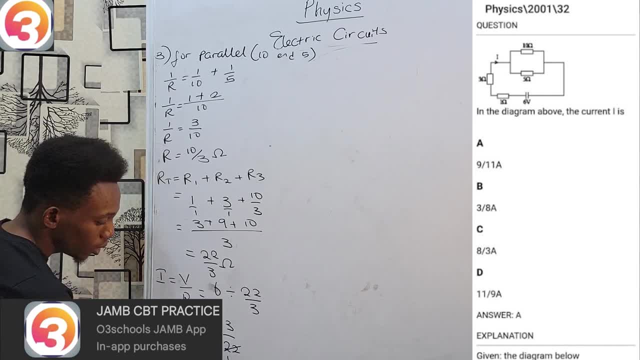 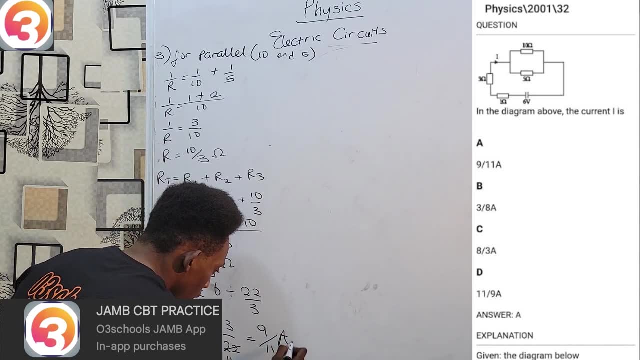 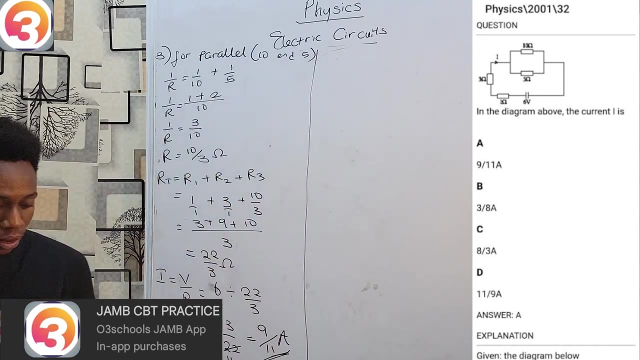 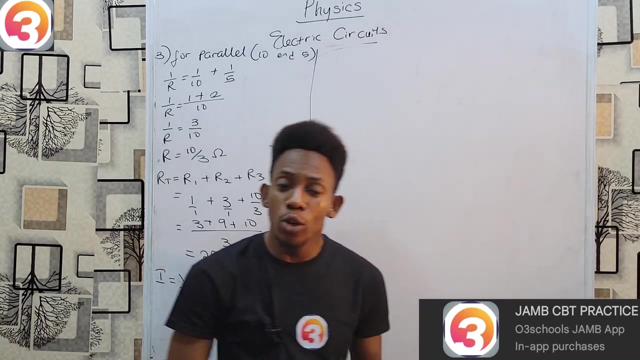 22 to six is three, two to twenty two, eleven and then three times three is nine, over eleven ampere and, as you can see, that is my answer, as shown in option a. you see simple analysis and you can get your answer. let's move on. 1995. question 31 on your 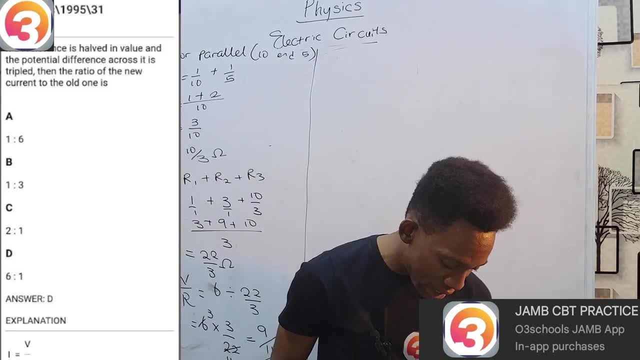 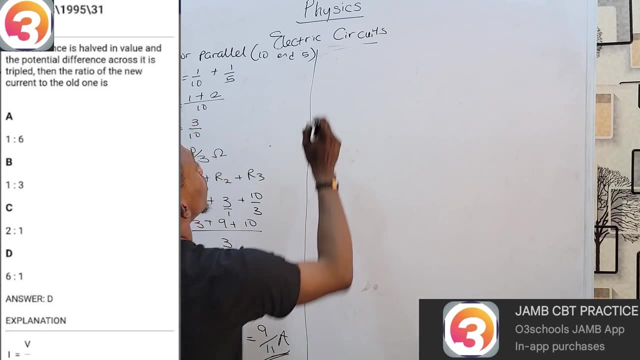 old. three schools jump up. the year is 1935, the question is number 31. this one says: if your resistance is half in value, that means initially let's say resistance was arrow first, increase the lighting. initially arrow one was arrow, then gets halved. that means now it's going to be arrow over. 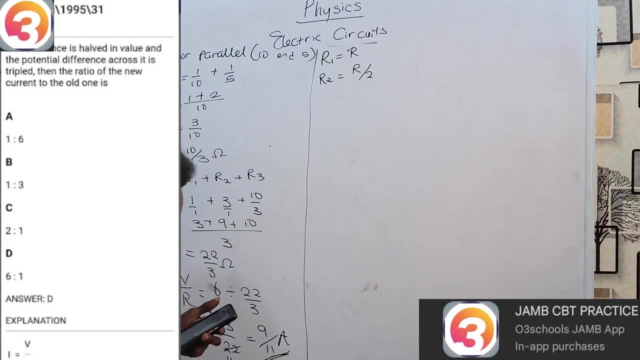 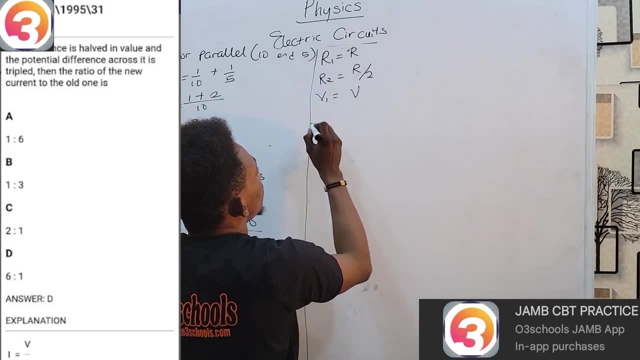 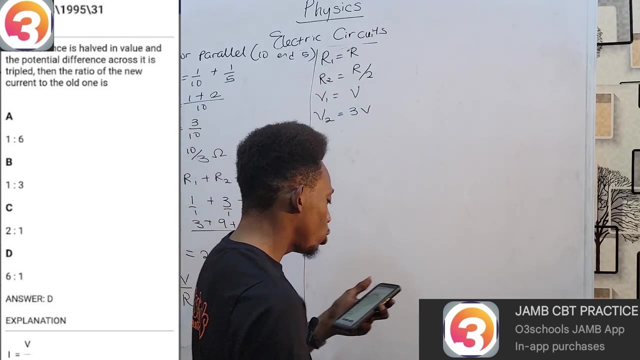 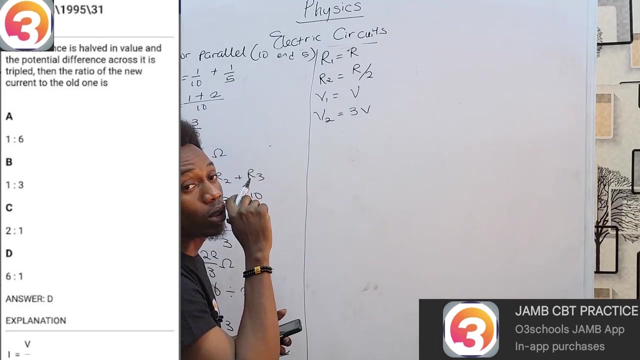 two. i hope that's okay. then the potential difference is tripled. that means initially the surface could have been v, but then it gets tripled. and tripled means times three that'll be 3v. but to find the ratio of the new current, so the old current. now all i have to tell myself is old current, i1 will be v1 over r1. 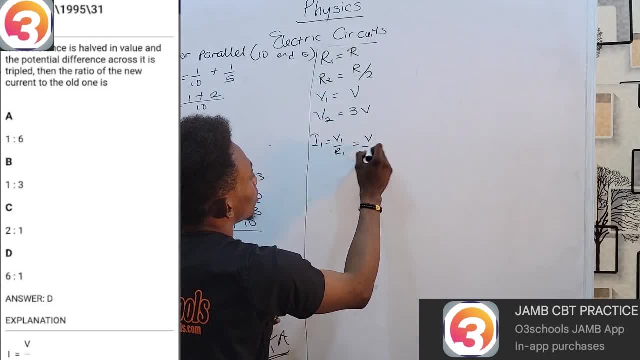 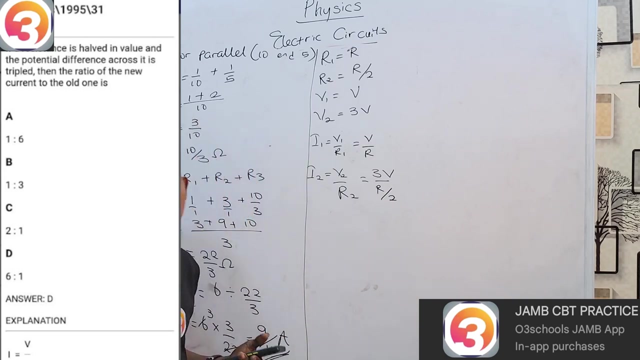 which is v1 is v, r1 is r, but my new, current i2 will be v2 over r2, my v2 is 3v and my arrow 2 is arrow over 2.. all you have to remember is that this over here means divide. 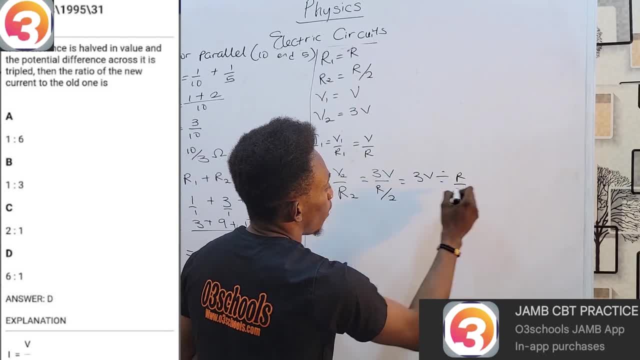 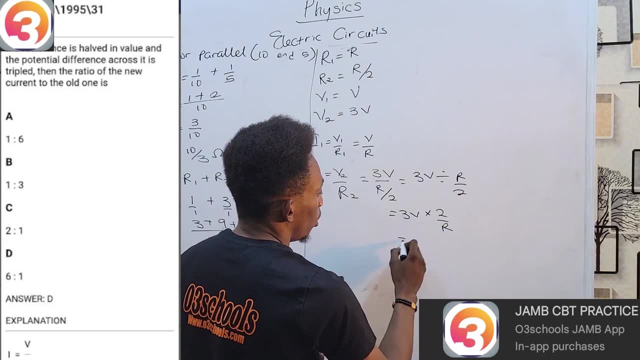 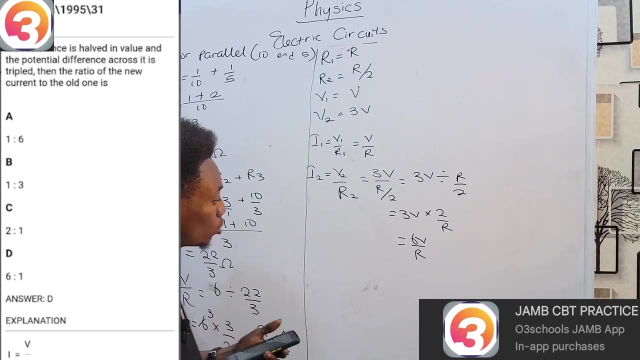 so 3v divided by r over 2, and then, using the knowledge of mathematics, that means 3v times 2 over r, which is 6v over r, and therefore the ratio of the new current to the old one, that means i2 over i1. 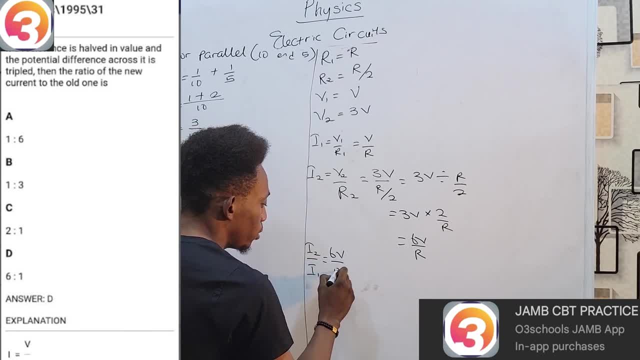 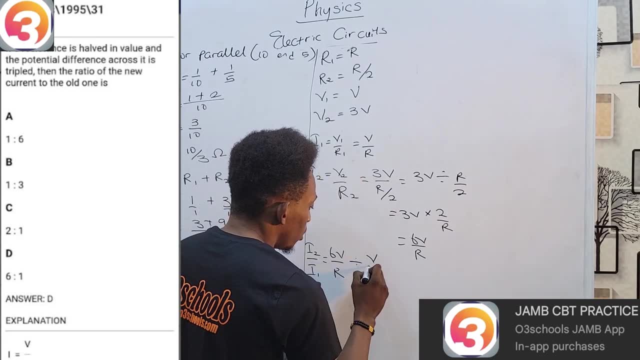 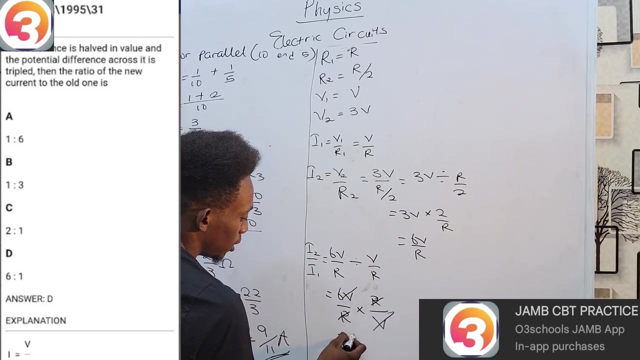 my new current is 6v over arrow over means divide by my old current i1, which is v over r. so i'll be 6v over r times r over v. arrow cancels arrow. v cancels v and that gives me that i2 over i1 must be 6 over 1, which is the same thing as saying 6 ratio 1, and that is option d. 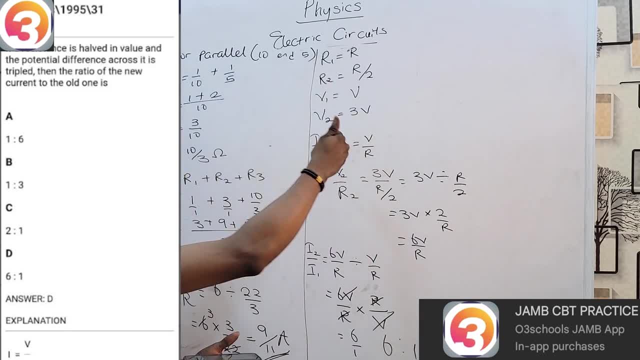 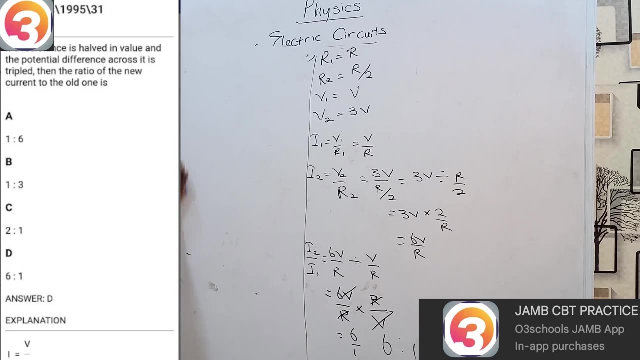 so, as you can see, when you get a question, try to write down your parameters and analyze carefully. don't skip any step, and you shall invariably be able to obtain your answer. okay, let's try a fifth question. i'm sure i'll collect this question from the year 2004. 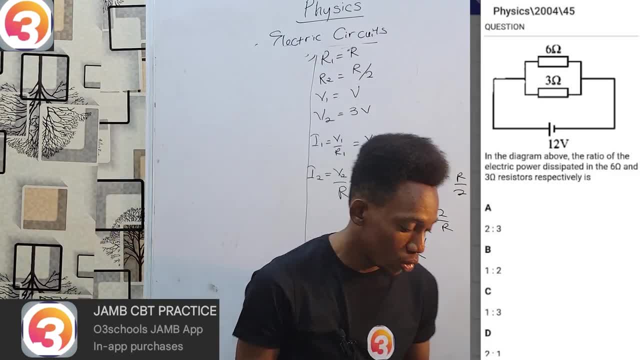 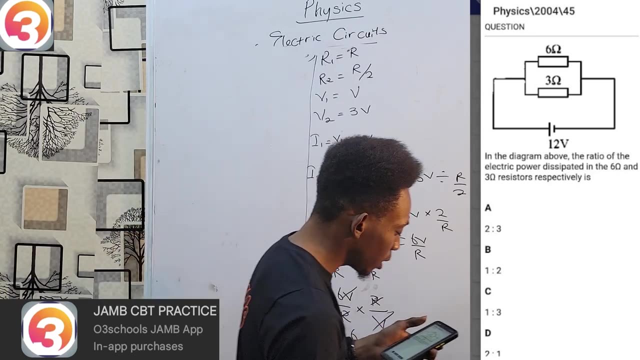 number 45 using your old three schools jump app. okay, this question now states in the diagram above: the ratio of the electric power dissipates located in the six ohms and three ohms respect resistors respectively is: we have a six ohm and a three ohm resistor, as you can see on your jump up there, and these resistors are in parallel with. 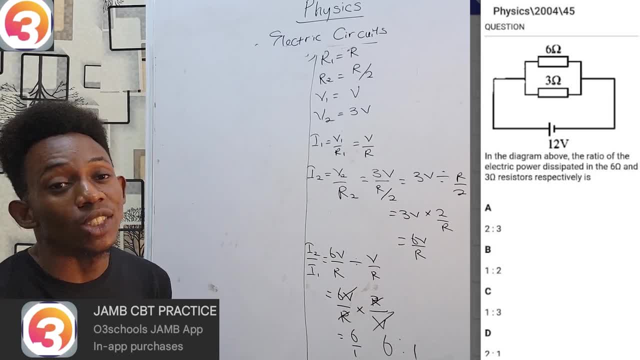 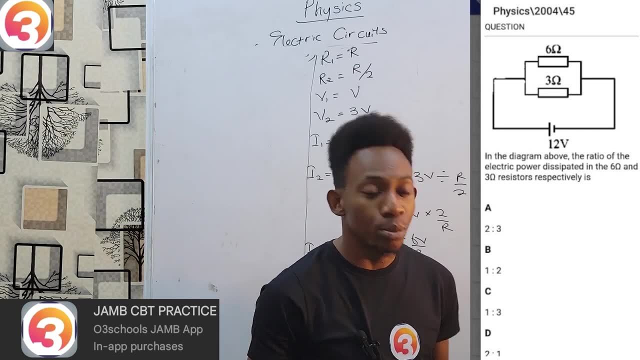 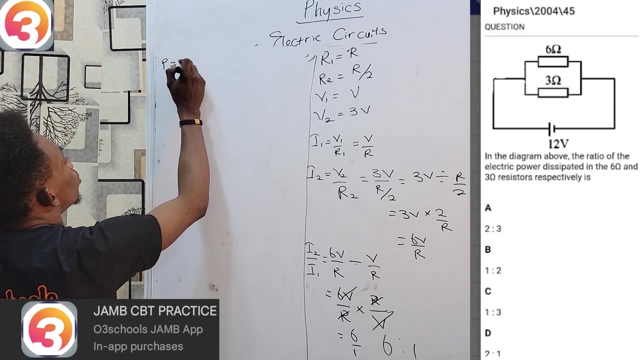 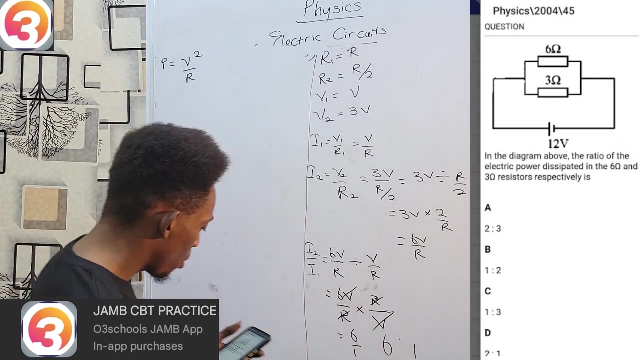 one another. what you want to find is the ratio of electric power. now, um, there are several ways to go through this. all i have to look for is a way to express the power in terms of resistance, and, as i'm aware, power equals to v squared over r. is that right? yeah, so for the first one, i can say: 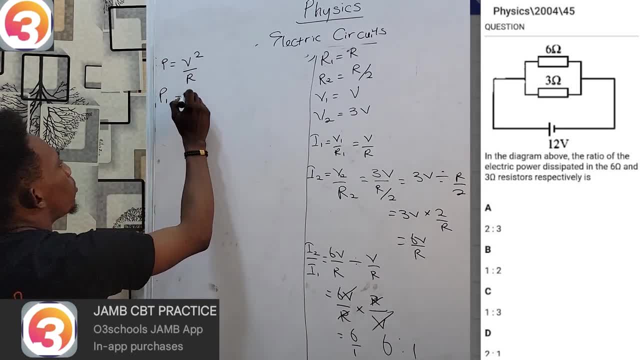 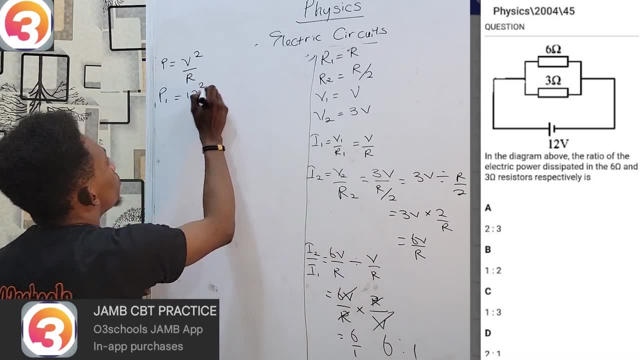 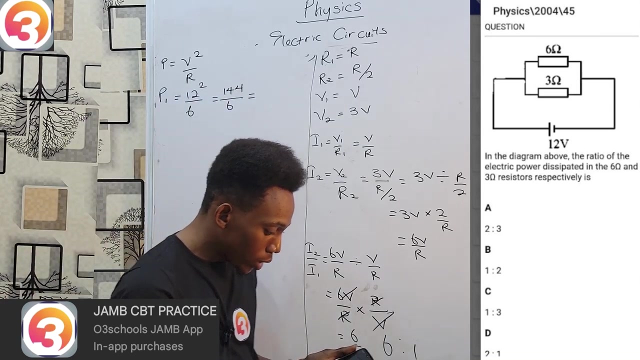 the power in the first one, p1 equals to my v, is obviously 12, because in a parallel circuit the share voltage. so that will be 12 squared over. for my first resistor, i'm going with six over six, that'll be 144, which is 12 squared over six. and if you were to divide that using your calculator, as you can see on the 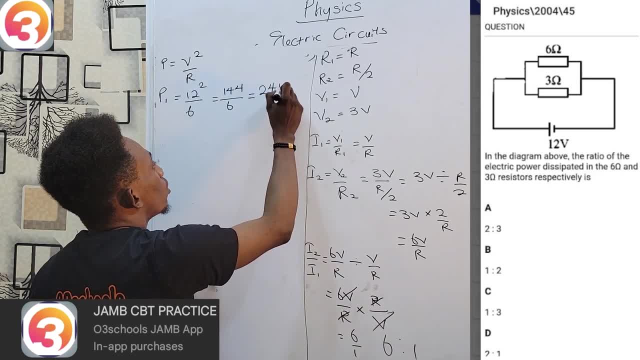 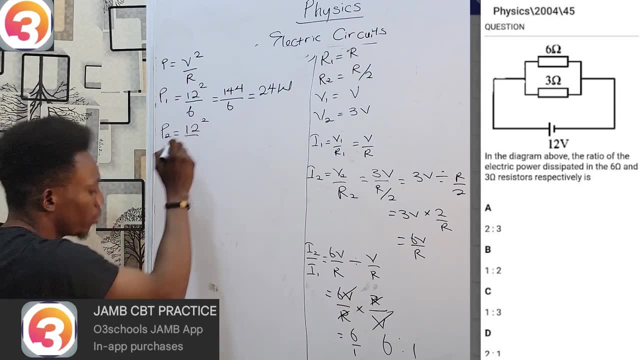 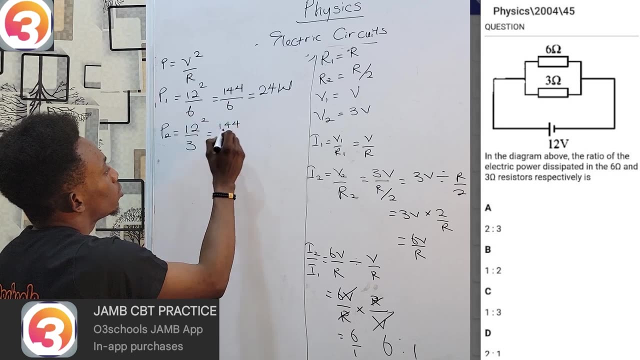 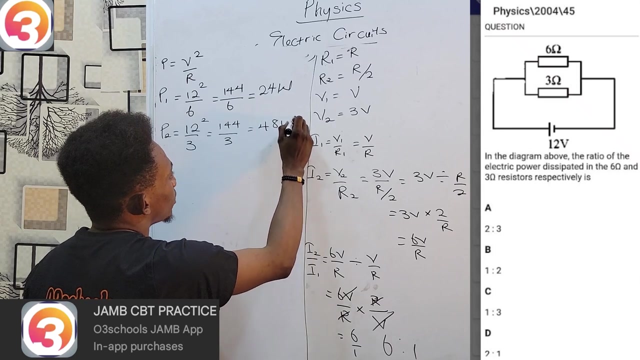 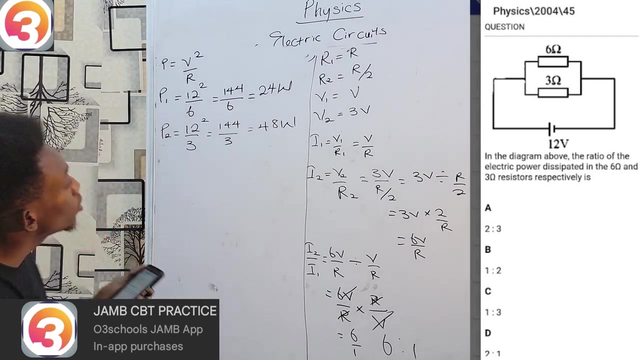 jump up, you get 24 watts. then for the second resistor your voltage remains 12, so 12 squared, while this resistor is three ohms, so 144 over three and this gives you 48 watts. so that means the ratio of the power in the six ohms to the three. ohms is my sixth is my three. 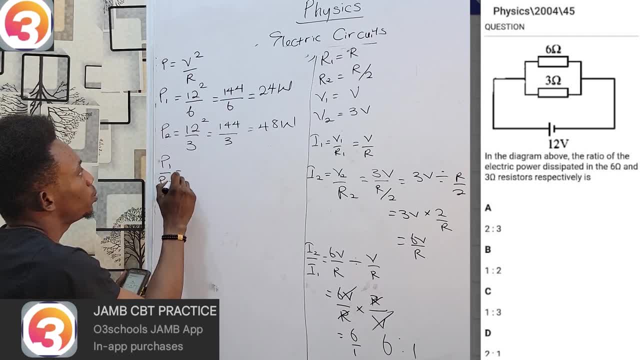 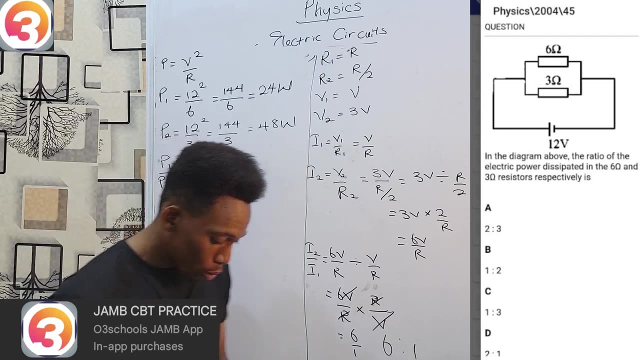 so p1 over p2 will be 24 over 48. 24 into 24 is 1, 24 into 48 is 2. so my answer is: 1 ratio, 2 option b. so please, if i was faced with what you clearly understood now, standardization is okay. 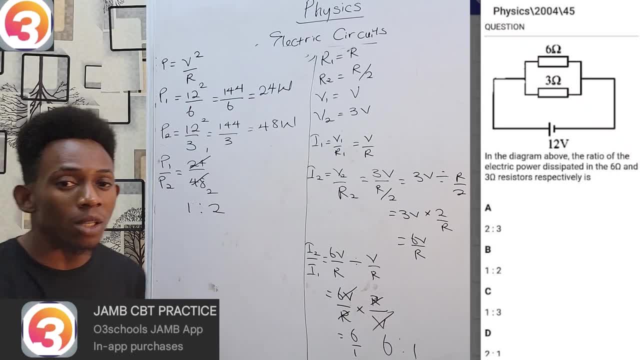 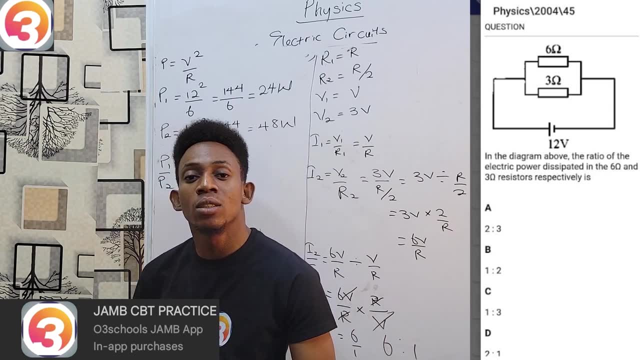 it can also be standardized. and so if you see, if, at, let's say, reduced tolerance, let's say we have this longand signal- i'm going to fractionalize that just by two of these two around here- then i will notice that we are left with this little. 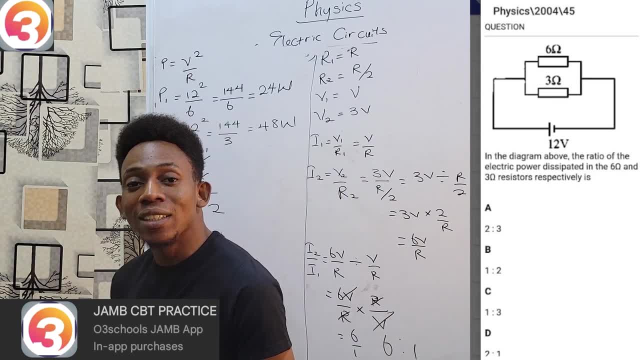 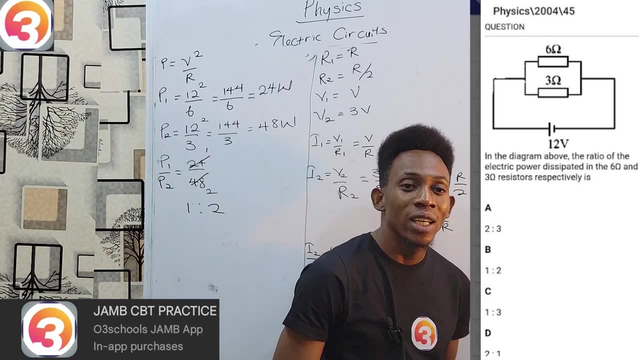 one and how that would be utilized to determine the power in program Governors withります. so what we can do is to blow that up and takehi out that band like one over five. radio connect two resistors in series, the total resistance is always greater. 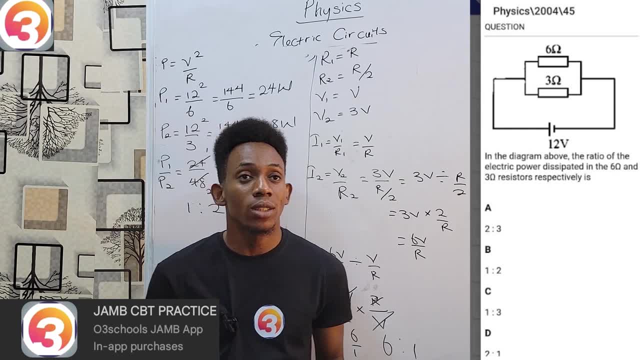 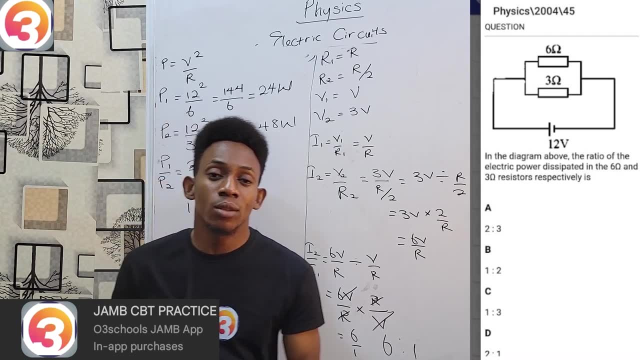 than the initial resistance. If I'm to connect, say, two ohms and four ohms in series, I get a bigger value, which is six. If I'm to connect two ohms and four ohms in parallel, then I will get a value which is smaller. 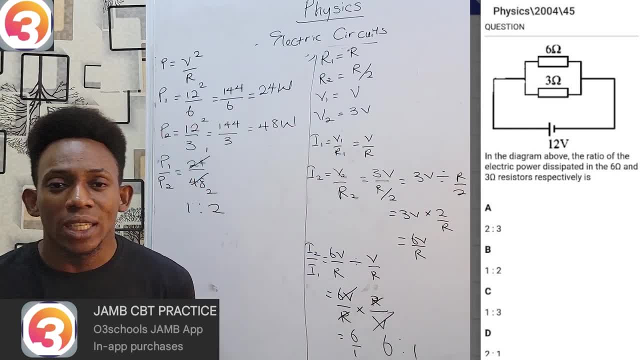 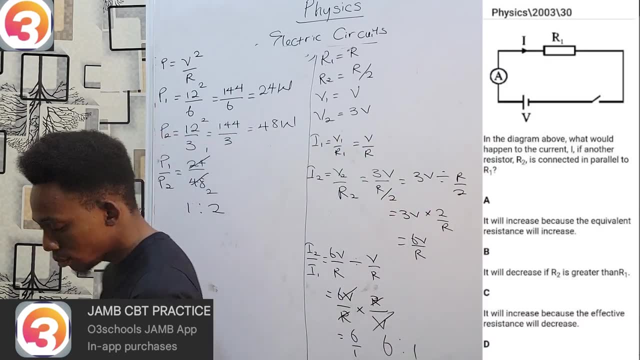 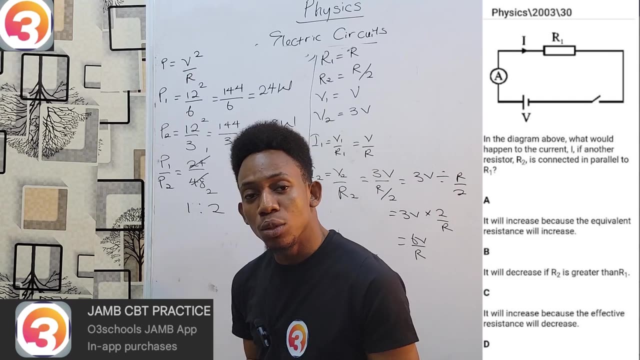 than both two and four. That's how resistances work, Such that, if you look at the question in 2003, question number 30, where we are simply told if we are to connect another resistor in parallel to the first resistor existing, 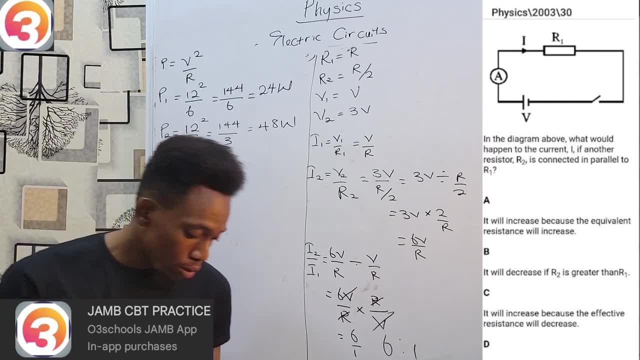 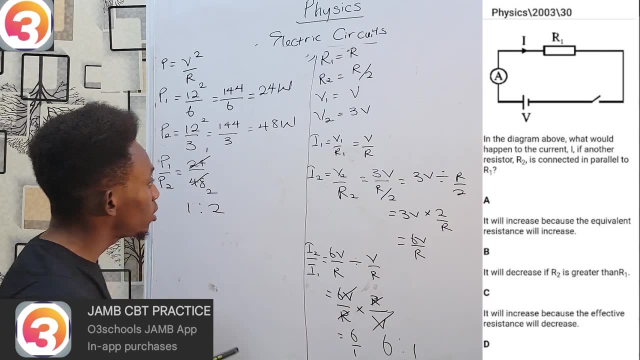 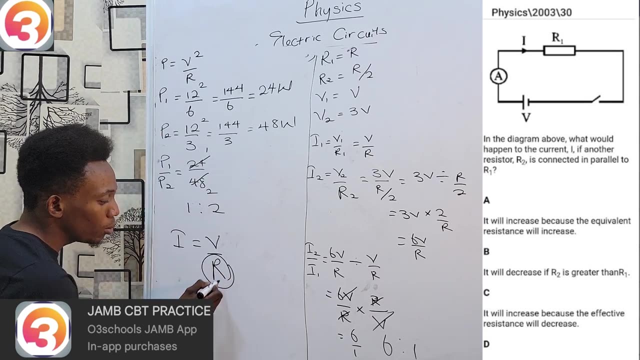 if I connect another resistor to the initial resistor. that was there. what happens to my current? As you are aware, current is simply using ohms law. I equals to V over R. The smaller my denominator, the bigger my current. and the bigger my denominator, the smaller the current. 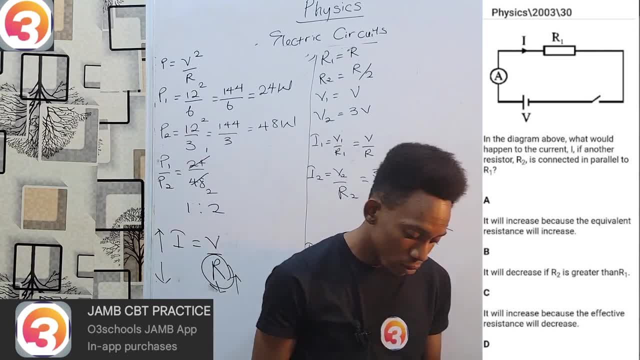 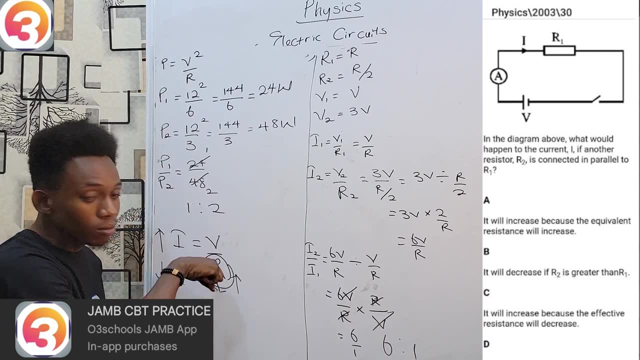 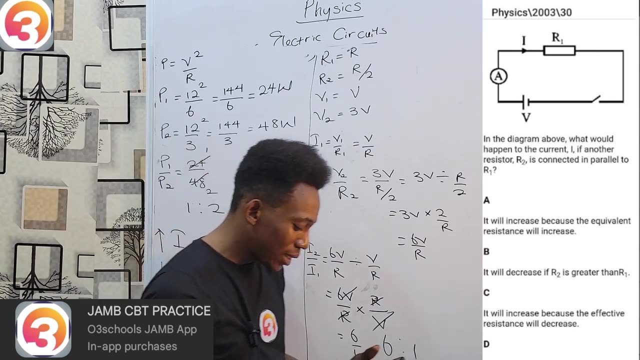 And now I know that if I'm to add another resistor to this, if I'm to add another resistor in parallel, then my total resistance will decrease. If my total resistance decreases, then my current increases. See, so the ocean becomes sea. 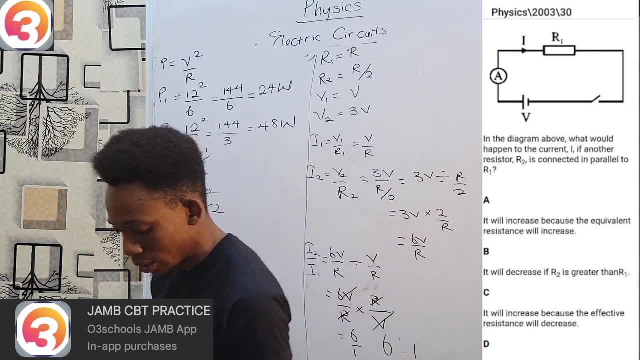 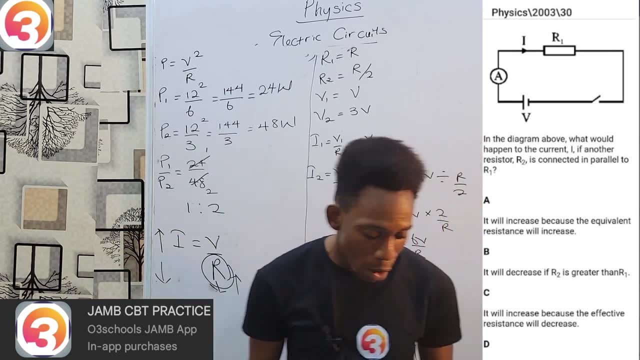 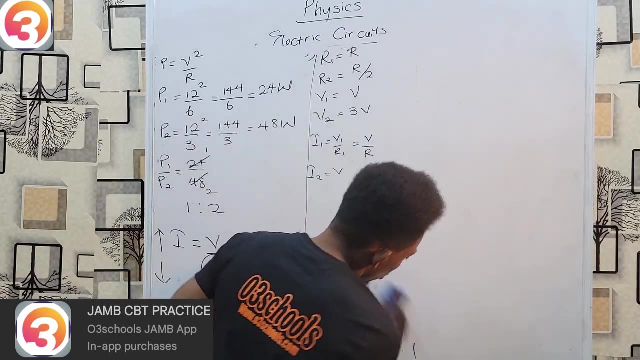 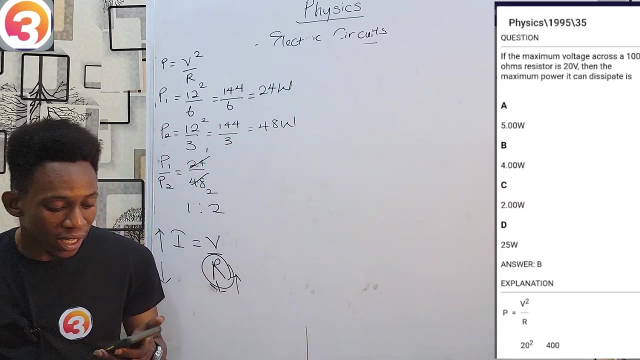 It will increase because the effective resistance will decrease. See, those are some of the simple questions we have to know how to analyze. Then, moving on, 1995, question number 35, which your old preschools jump up. 1995, question 35.. 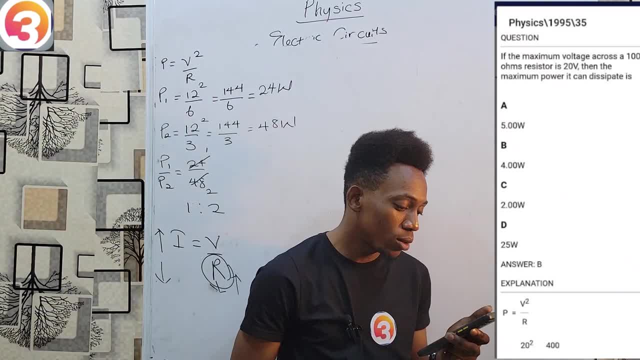 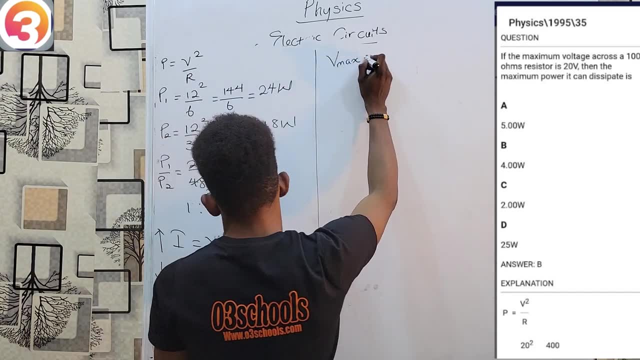 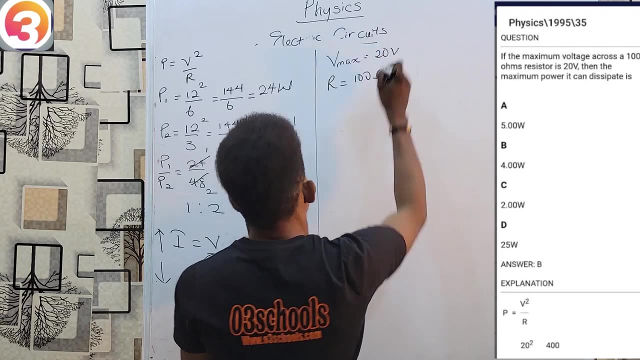 If the maximum voltage across a 100 ohms resistor is 20 volts, the maximum voltage- let's call that the Vmax- across a 100 ohms resistor is 20 volts, We have to calculate the maximum power it can dissipate. 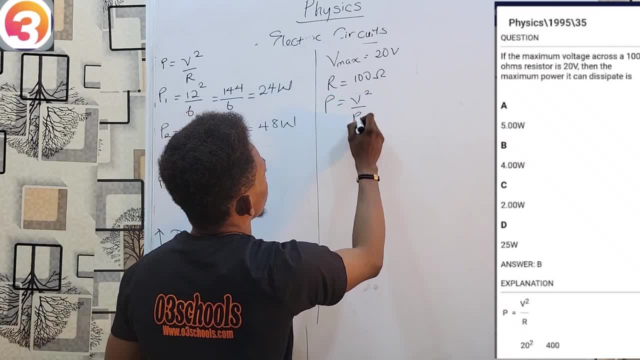 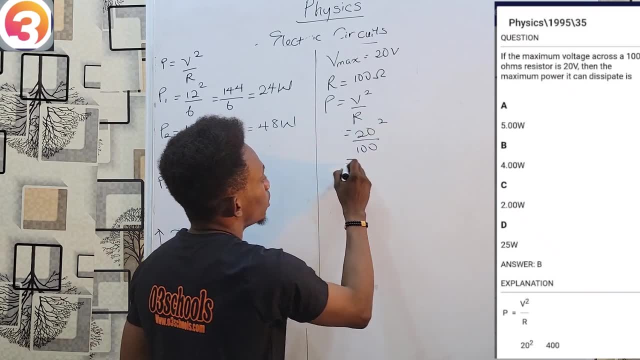 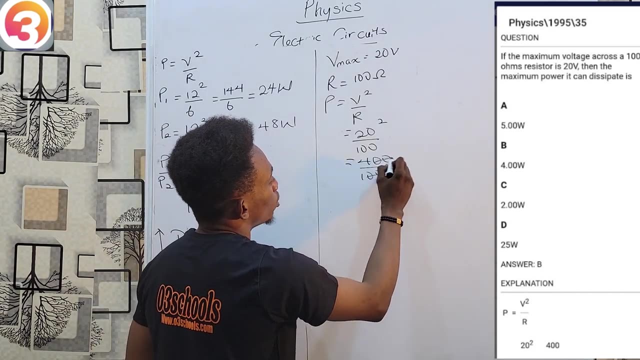 You have to remember, power equals to V squared over R. See quite simple Now: V is 20 squared over R, which is 100.. 20 squared means 20 times 20, and that is 400 over 100.. Zeroes cancel zeros and that is four watts. 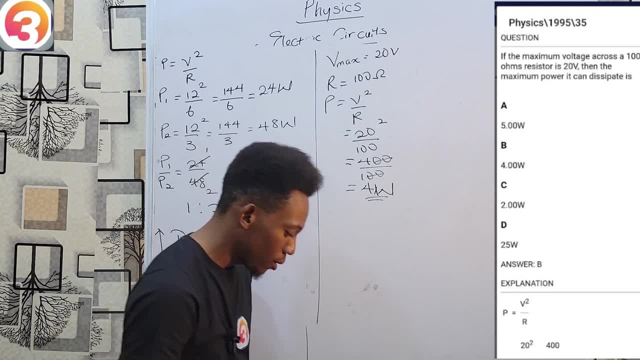 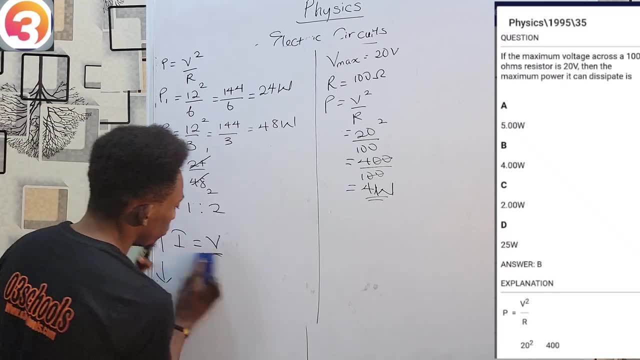 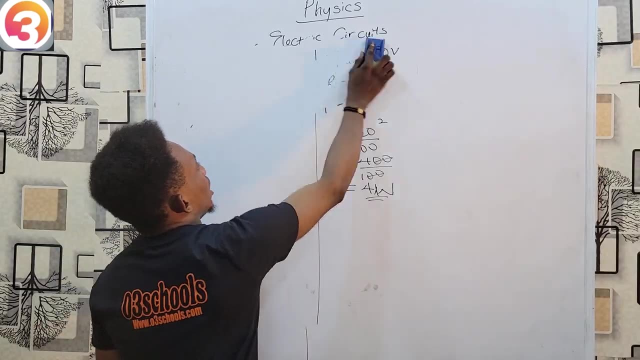 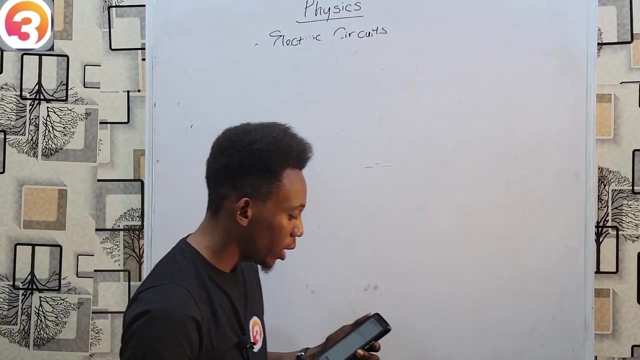 See option B. Very, very, very simple, And I think we shall solve one last question and we shall be able to see that we've done a complete and thorough analysis of resistors in electric circuits. Okay, And now this, our last question comes from the A. 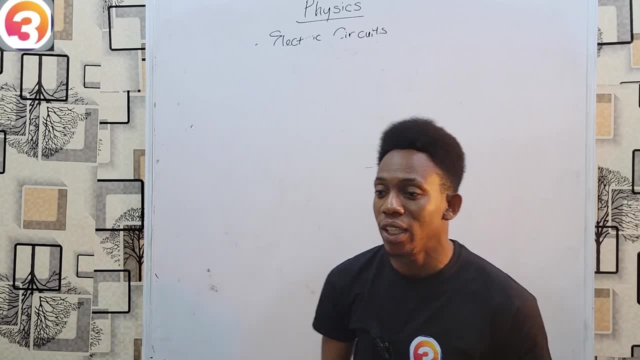 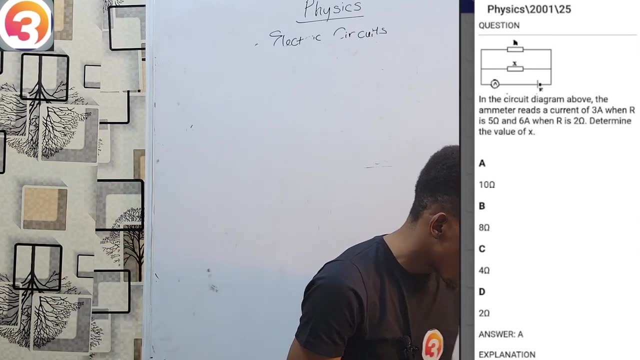 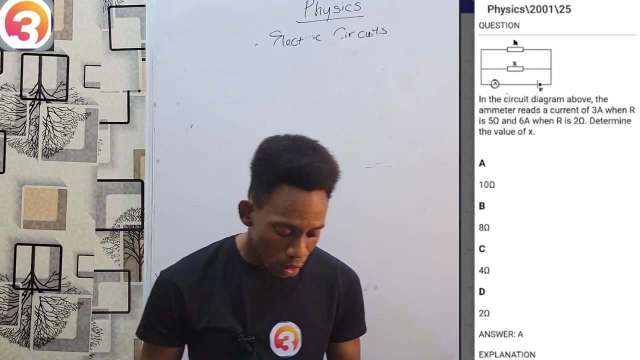 2001,. question number 25, 2001,. question 25.. Taking a look at your old preschools, jump up you can see. we have a simple circuit diagram and we are told that the ammeter reads the current of three ampere. 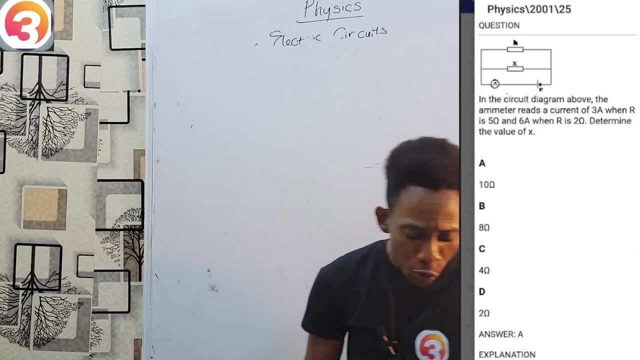 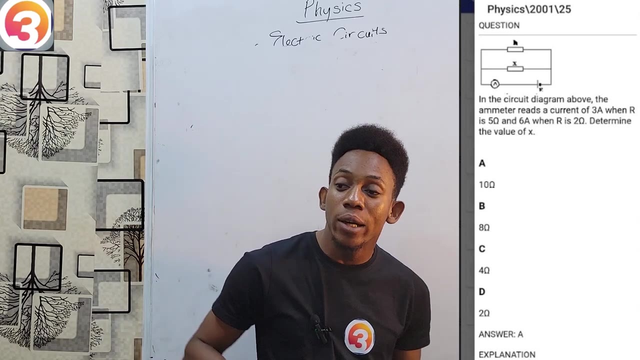 when R is five and it reads: the current of six ampere when R is two, that will determine the value of X. Now, before we do any analysis, we must first of all understand that my two resistors, R and X, are parallel to one another. 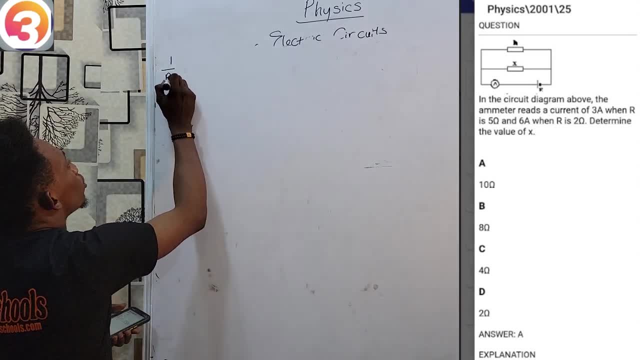 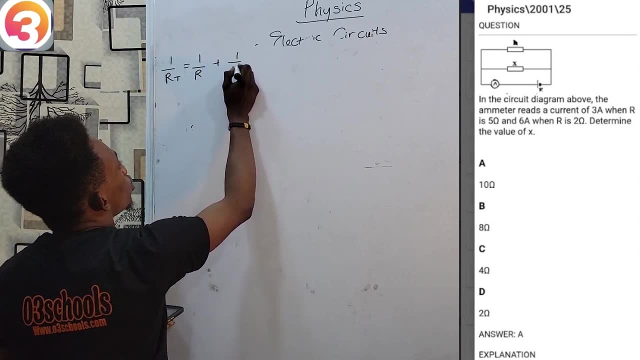 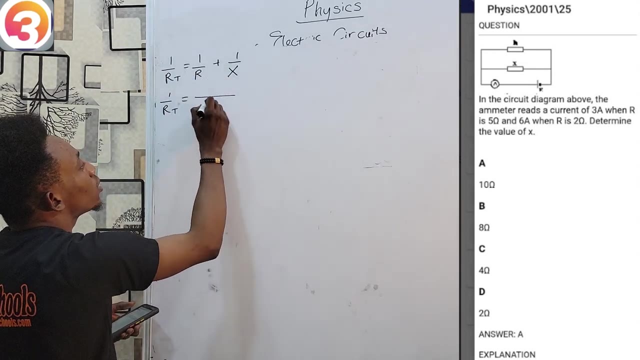 and that for any parallel combination, one over R, total must be one over R one, taking my R one as R plus one over R two taking R two as X. So one over R two becomes L same of R, and X is R X. 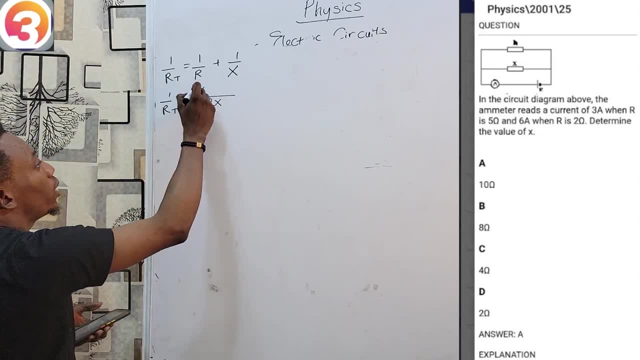 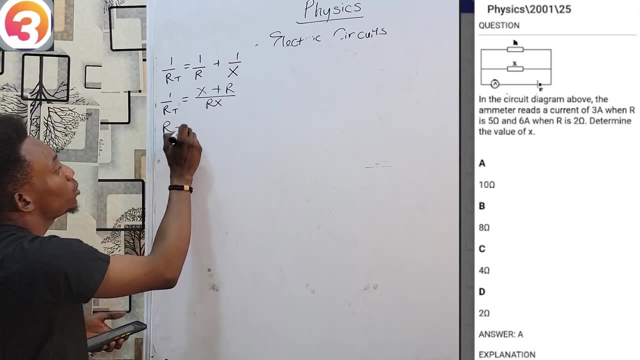 plus one over R two, taking R two as X. So one over R two becomes L same of R and X. is R X, R, X over R, X, R X over X R. Now, turning both sides around, R T becomes simply R X over X plus R. 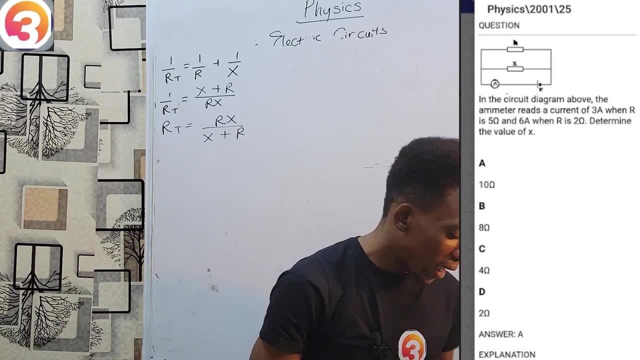 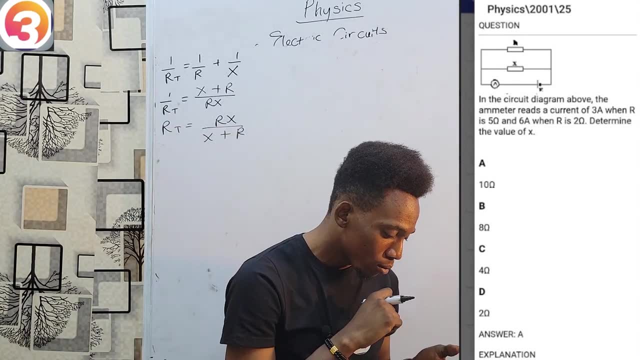 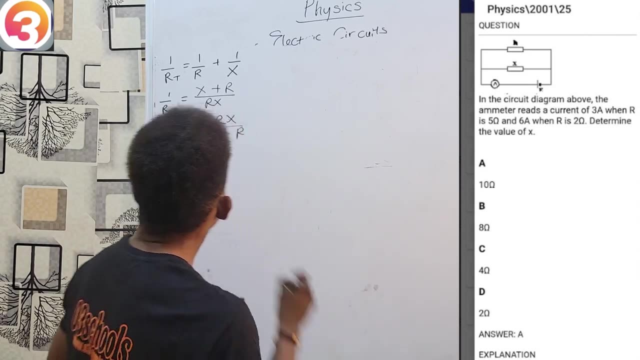 That means I have a simple way to determine my resistance given any single value of R and X. Now for my question. what I know is that I get the current of three when R becomes six, And I know that my voltage, or EMF, 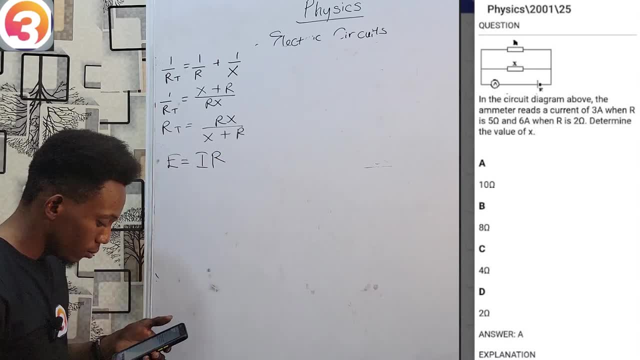 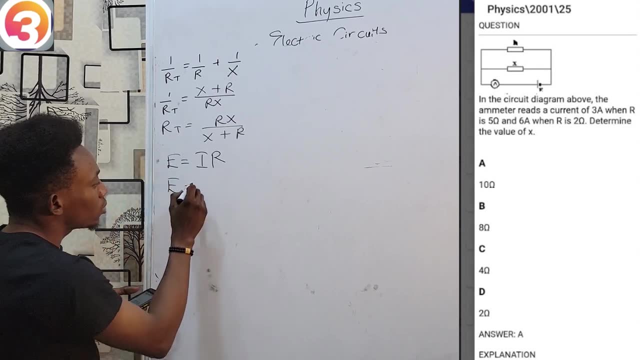 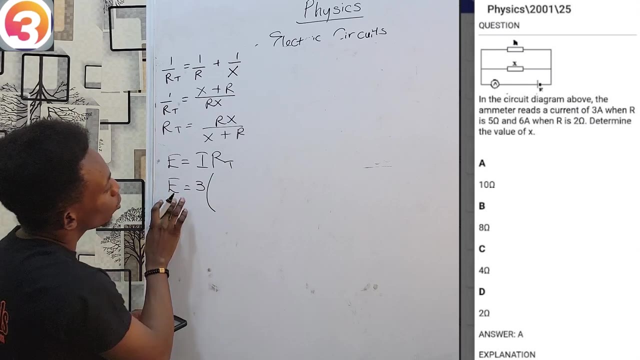 at E equals to IR. Now I don't know the value of E, but I know that I becomes a value of three when R becomes a value of five, So E equals to three. When this, my R, becomes five, then R T becomes. 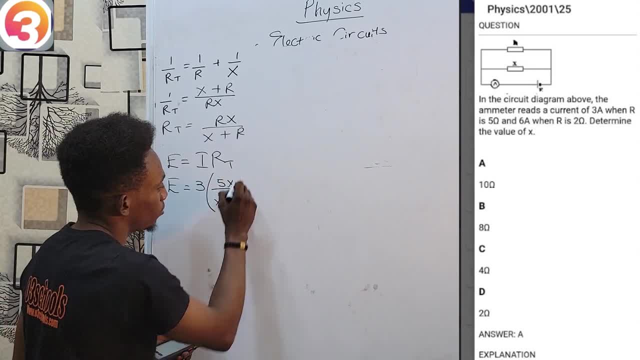 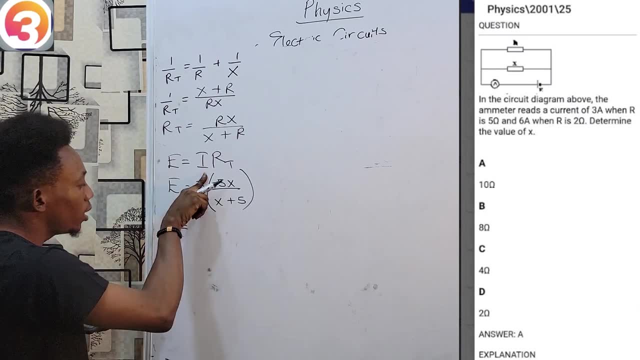 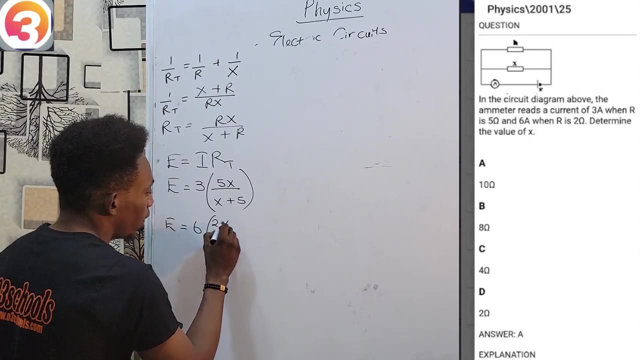 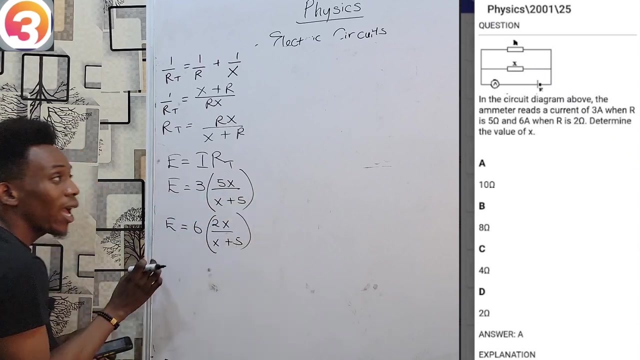 five, X over X plus five. And E is also equal to I again, but my new value of I is six ampere. when R becomes two, That is two X over X plus five. Now you see, E equals this, and yet E also equals this, indicating therefore: 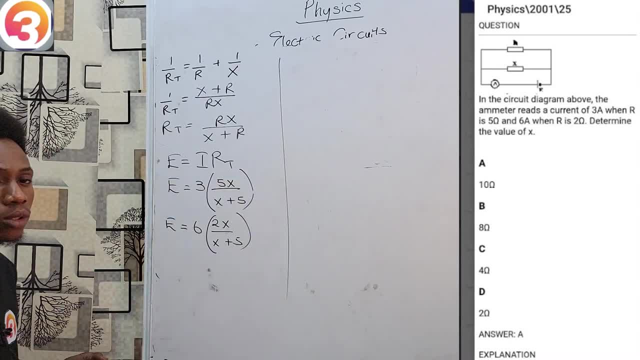 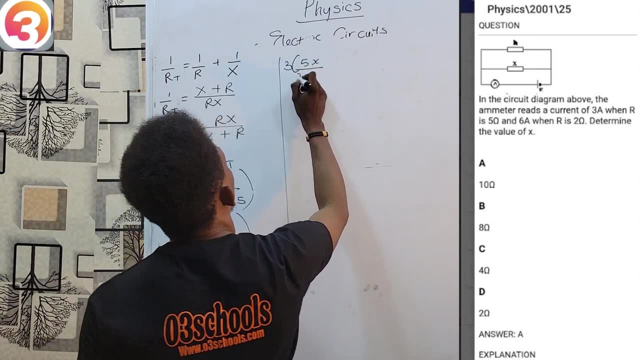 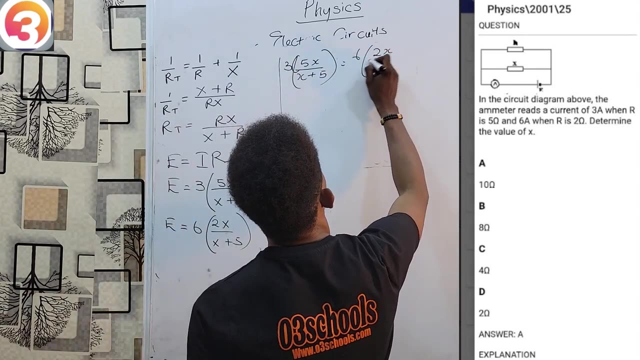 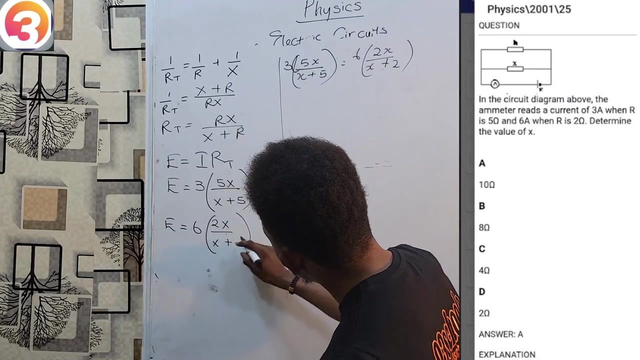 that this and this must be equal, So all I have to simply do is note that three into five- X over X plus five- is equal to six into two X over X plus two. That was almost a mistake. please be careful. 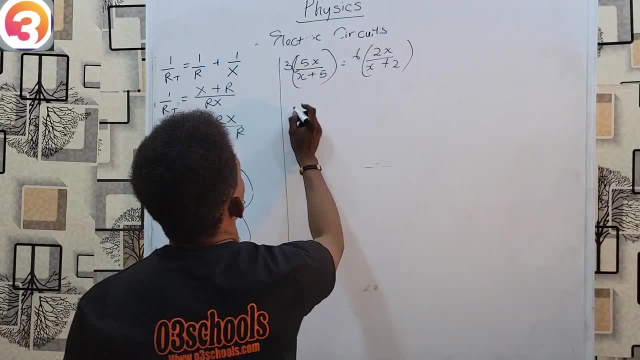 It's X plus two because R is now two, So open my brackets. three times five is two, So open my brackets. three times five is two, So open my brackets three times five. X is 15X over X plus five. 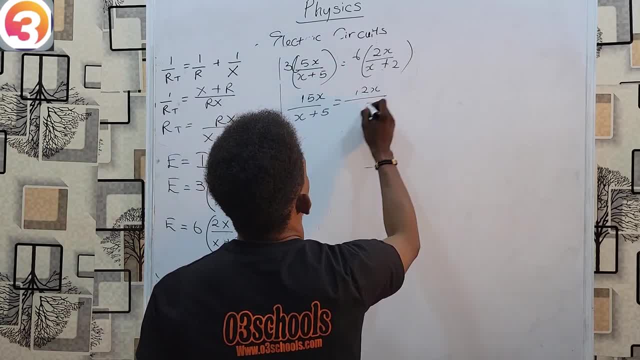 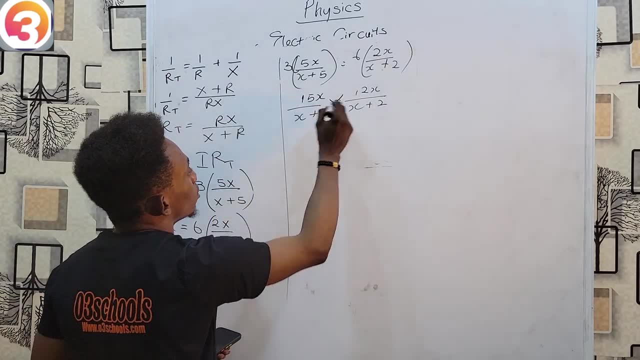 Three to six times two, X is 12X. all over X plus two Is 15X over X plus five. three to six times two, X is 12X all over X plus two. Now, if I cross multiply it gives me 15 X into X plus two.